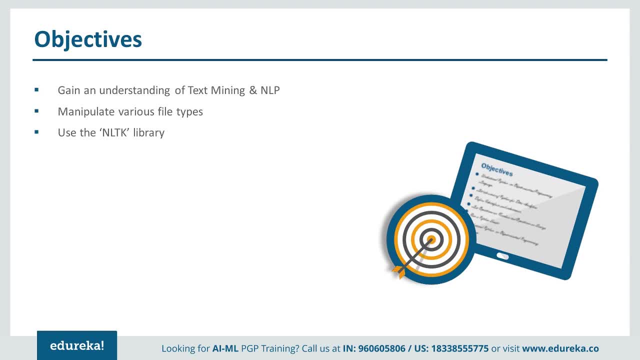 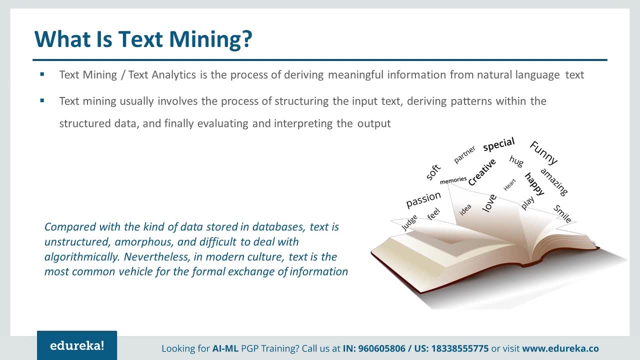 how to manipulate various text file types and how to use the NL TK library. So what do you mean by text mining? text mining, also known as text analytics, is a process of deriving meaningful information from natural language text. Now the question comes is: what is natural language? 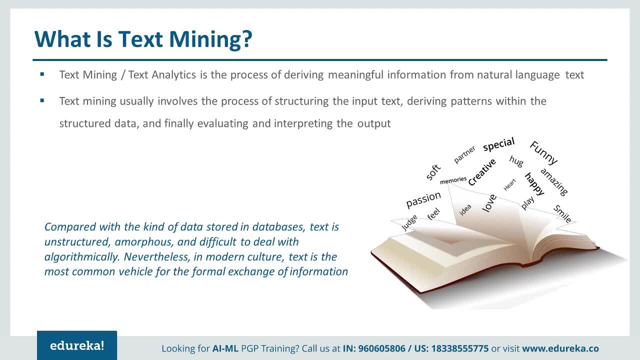 So this word natural language comes from the English. like we are, whatever we speak, Maybe a natural language is something which other person understands while interacting. So maybe I don't know English, I know Hindi and I'm interacting somebody with Hindi, So my natural language is something called Hindi. 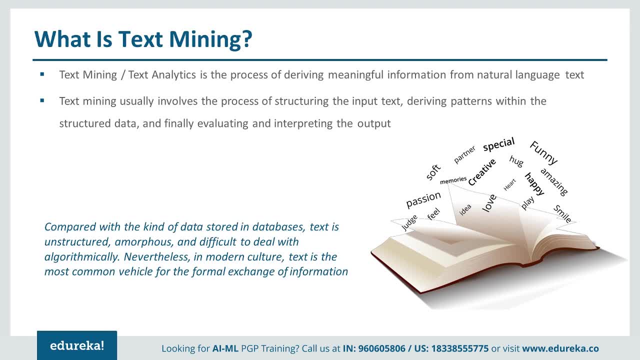 which other person understands. So in terms of computers we talk about natural language. So what very commonly used language is English, language which computer can understand? and for natural language processing We use English as a primary language for natural language processing. You can do natural language processing in German, in Chinese. 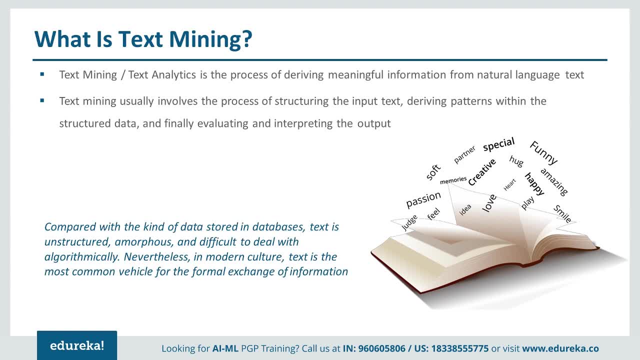 or maybe Hindi, but whatever we speak up in system is able to understand it correctly. that is known as text mining. text Mining: the process of deriving meaningful information. driving meaningful information means whatever we are speaking or whatever the text we are giving, maybe in the form. 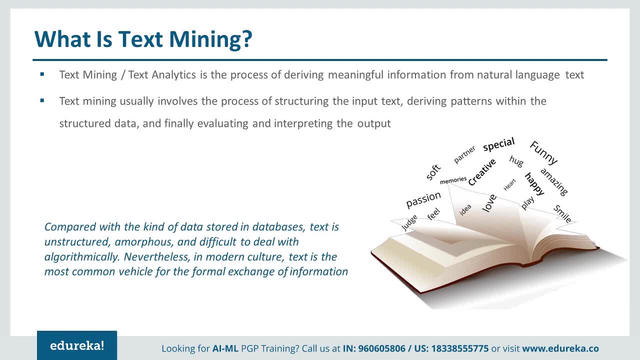 of a words, maybe in the form of a sentence, maybe in the form of a paragraphs- system can understand it and get some meaningful information out of it? How system can get meaningful information that, say, I use a word like I am going, so I am going is English sentence? 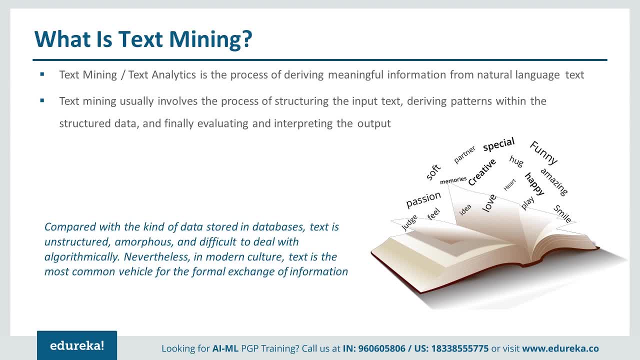 which is continuous sentence. It is not in past tense, It is not in future tense, It is simply in the present, continuous. that, okay, I am going to certain place now. system should understand whether we are talking about the past or whether we are going to talk about the future. 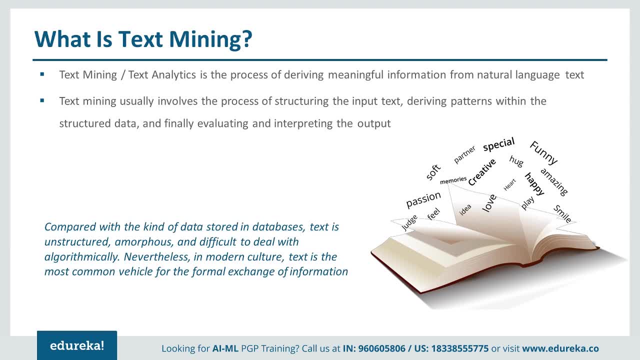 or whether we are doing going to talk about the current point of time. So it is going to identify various identifiers in this world. It is going to divide this word into various identifiers internally and understanding how many verbs are there, how many adjectives are there, how many nouns are there, how many pronouns are there? 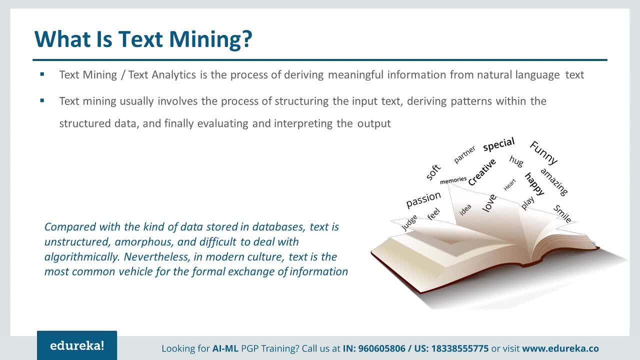 So, internally, it is classifying the word depending on the word, what exactly it is. So I'm going. so going is a word which is continuous in nature. System is going to identify by tokenizing each word, by taking separately each word and define its characteristic. 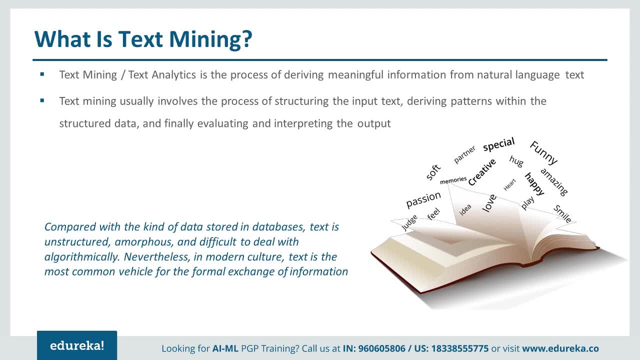 whether it's belongs to a noun clause, when it belongs to a pronoun clause, whether it's belong to adjective clause, and based on that, it is deriving some meaningful information. meaningful information can be: if I'm going, that system can remind me. Okay, Why don't you take your mobile phone as well? 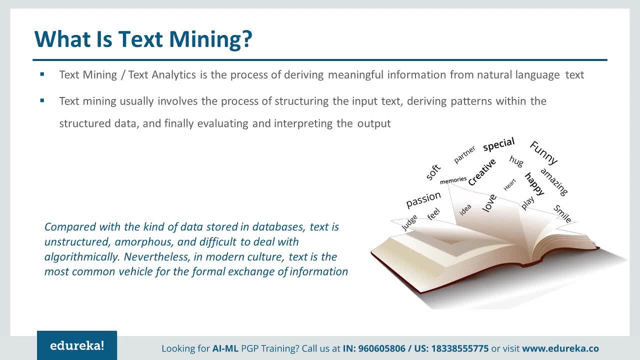 Or why don't you take your purse as well? So, based on this information system is going to take some decisions, whatever the words you are giving or whatever sentences you are giving. so text mining, or text analysis, is basically deriving meaningful information from the contents. 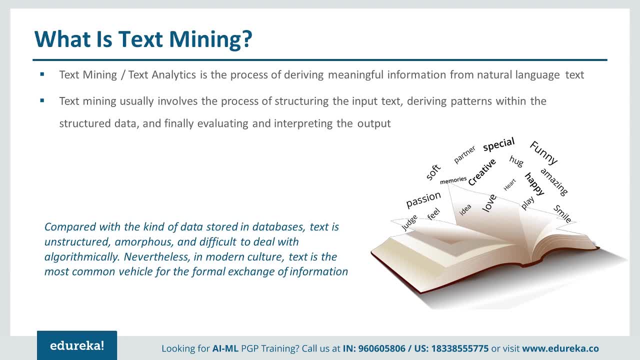 We are giving to the system. text mining usually involves the process of structuring the input text, deriving patterns within the structure data and finally evaluating the and interpreting the output. So there are various steps in text mining. First of all, we process the unstructured data. 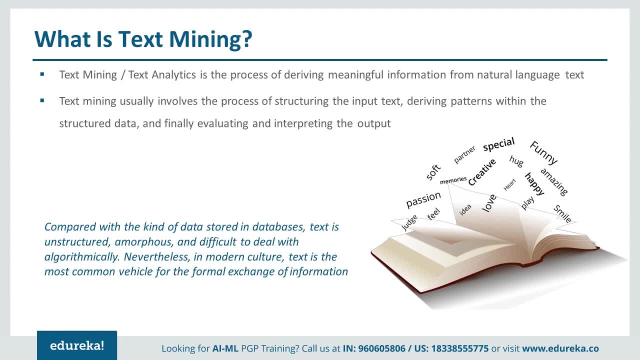 or the input data process, means we are going to tokenize it in terms of what is verb, What is adjective, What is at verb in that, deriving some patterns there but driving some common characteristic that says you are saying I'm going and I'll be moving with my car. 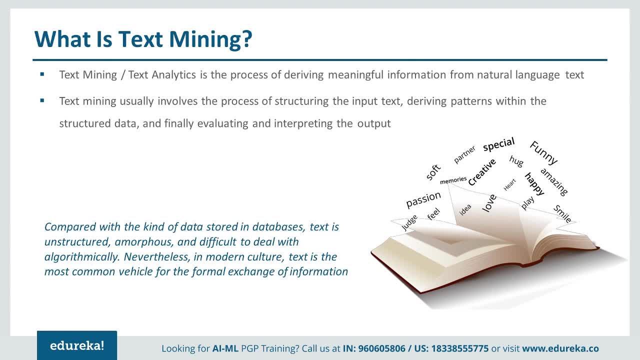 I'll be going with my car. So it's finding the relations between the different words. So if you're going, how you are going, by which mode you are going, which transportation you are going. so it is driving some patterns from the existing data. So if you supply some sentence, 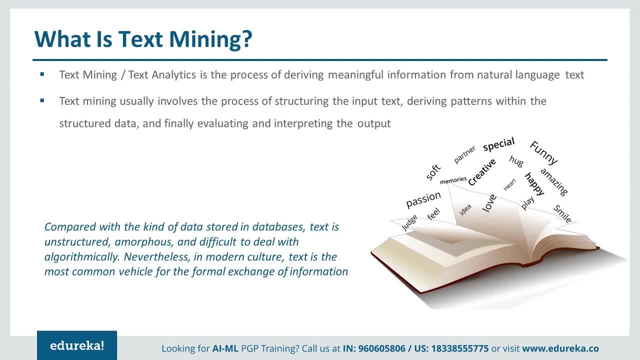 it is finding out the correct details out of it. Suppose you say I am going, another sentence You're going says I am going by train. second sentence is more complete in terms of how you are going. So it is finding out the patterns in the data. 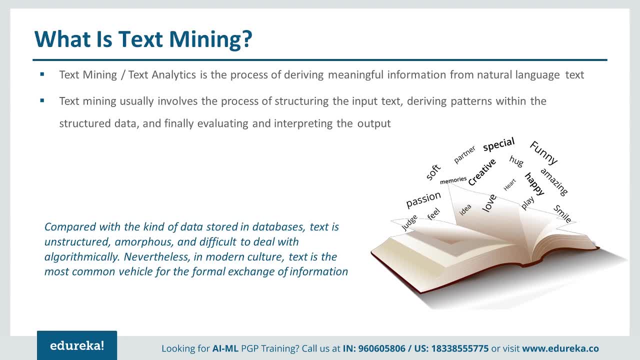 like how it is shifting from one pattern to another. Let's say you are talking about a future data. It is going to talk about okay, in future This is going to happen, So everything will be the future tense. So system is going to identify some unique patterns in the data. 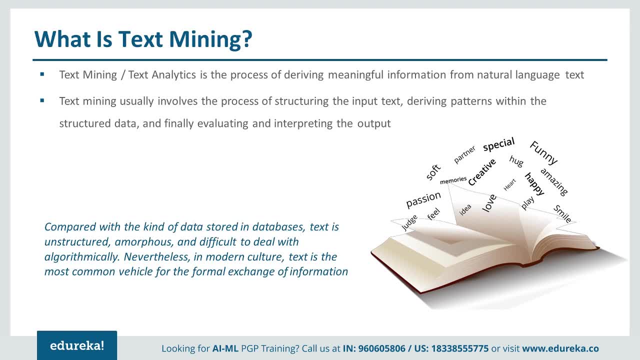 We can see it's unstructured or structured, anything. and finally, evaluating the, interpreting the output. So what is output? output can be. let's say you are going by car. The output can be: system is going to recommend you. Okay, why don't you take some keys of the car as well? 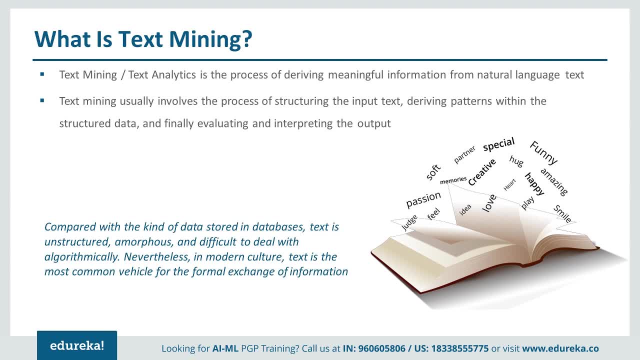 or have you taken the your wallet as well or not? So, based on certain data which you're providing to system, system is doing some kind of a decision-making what actions to be taken. It's more like a action reaction kind of a situation in natural language processing. 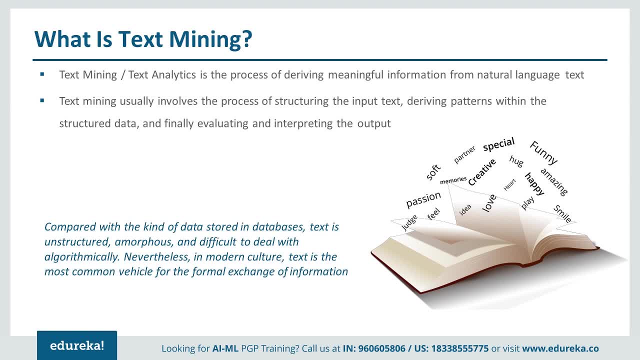 Whatever the action we are taking based on that system is reacting to it. depending on that sentence, We have feed in into the machine to compare to the kind of data stored in databases. Text is unstructured, enormous. It's huge in size and difficult to deal with algorithmically. 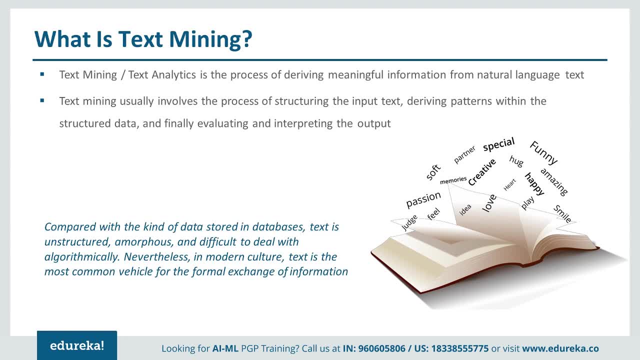 So you might have worked on machine learning. all the projects You might have seen. all the machine learning projects require discrete, continuous data. It is not going to work on discrete data. So text mining is basically filtering out the important words from the text and, based on that, taking some decisions. 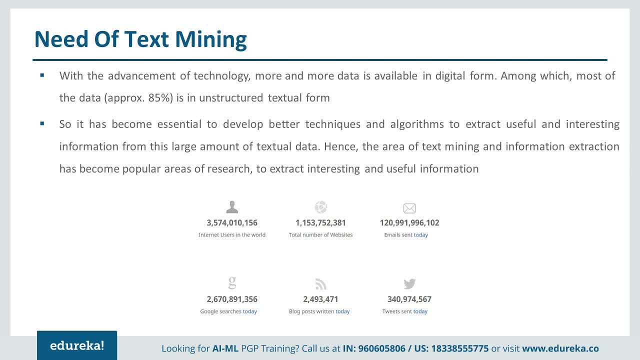 So what is the need of text mining? with the advancement of technology, more and more data is available in a form of a digital format, among which most of data, that is, 85%, is in unstructured textual format. So in today's world, whatever data we are having, 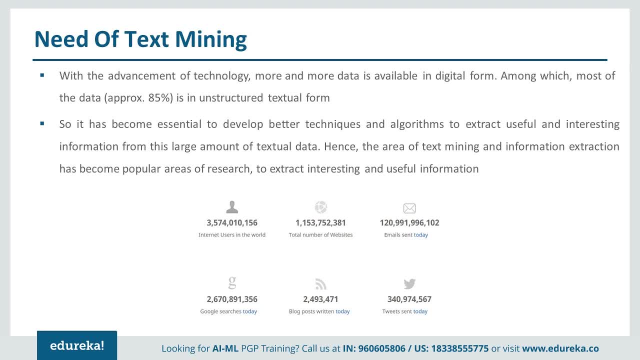 which is huge chunk of data. if you imagine hundred percent. 85% data is unstructured, which is not following any structure. What do you know? unstructured data which is not following any structure means column headings or any kind of a tuple having column headings. 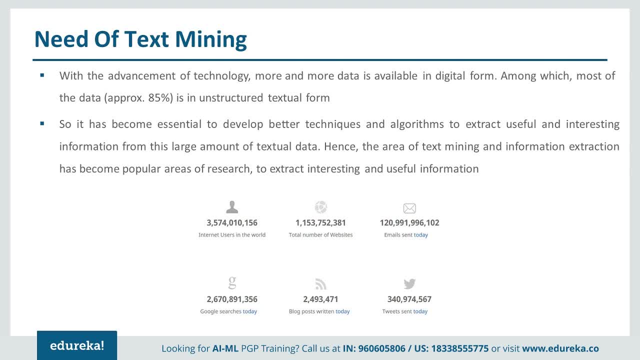 or you can say attributes there in the data. So it is unstructured, means it is kind of a sentence. It can be five word sentence, It can be hundred word sentence and it is in a textual format. So it has to become very essential to develop better techniques. 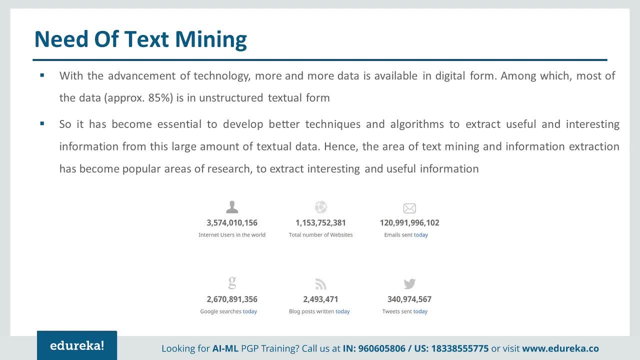 and algorithm to extract useful and interesting information from the large amount of textual data. So now it's our role as a data scientist to figure it out: How this textual data looks like, what are the benefits of reading it, how to take decisions based on that. 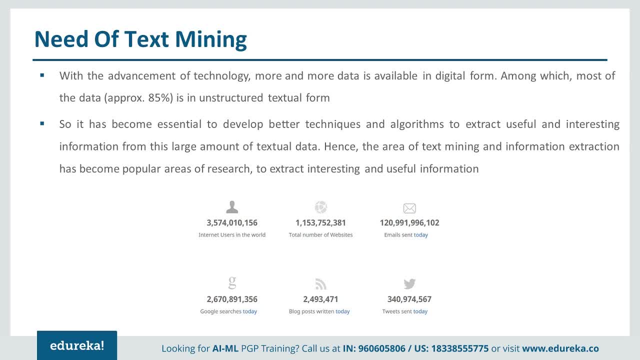 and dealing with the chunks of huge amount of data. It's a real challenging task because all the words are different, how they are used and everybody has a different style of writing some letters, maybe emails, if you need to figure out the feature vectors from that email. 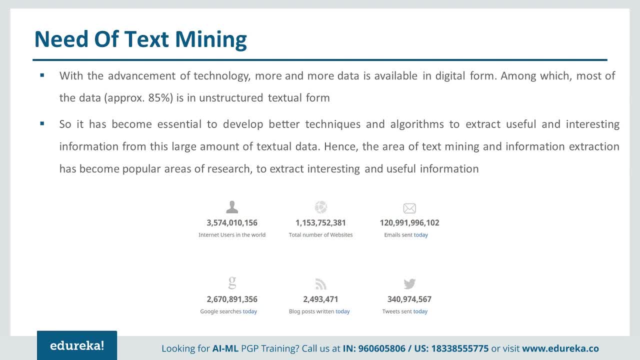 Okay, this is the style of somebody to write the email, So this mail belongs to this person. So hence the area of text mining and information extraction has become popular area of research to extract interesting and useful information. So one of the areas we use text mining is: 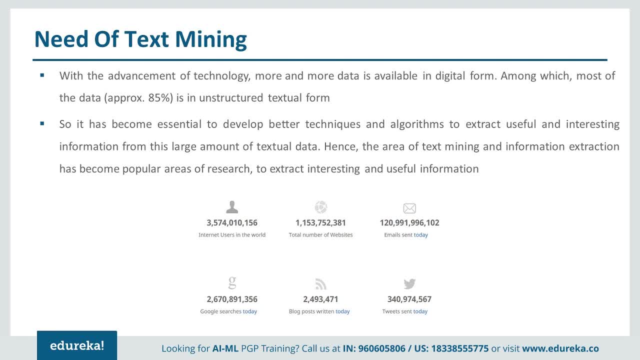 to extract some interesting features from the data, to find out insights into it. So, if you see, internet users in the world, there are almost like figures, which is something very big: total number of websites, email sent every day, Google searches every day, blog posts every written today. 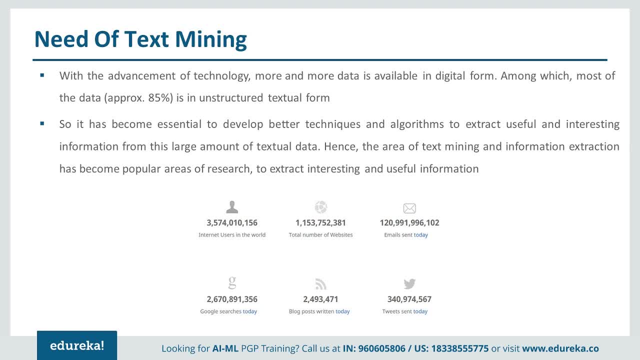 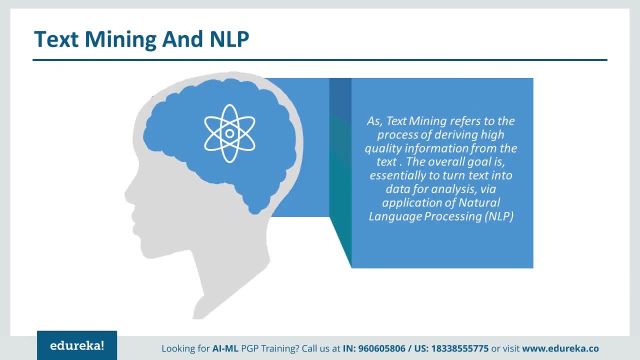 to its friend today. So you can see, there's so many millions of users who are sending data in a form of a text from one format to another. so, as text mining refers to the process of deriving high-quality information from the text, The overall goal is to essentially to turn text. 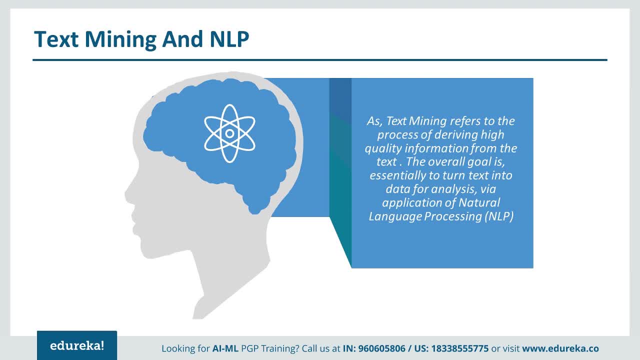 into data for analysis by application of natural language processing. So what does this mean? text mining refers to the process of driving high-level, quality information from the text. So what is the aim of text mining? to figure it out The important words that we supply in the text. 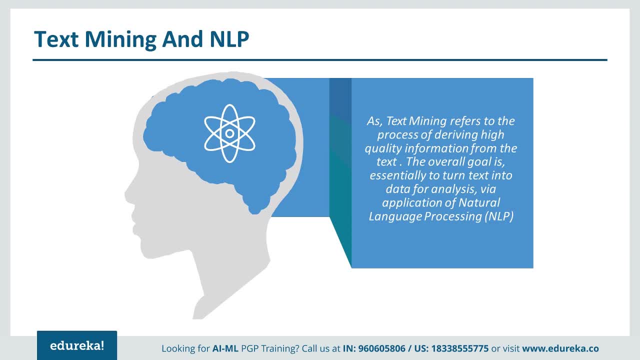 get some valuable information from there. The overall goal is what? to turn text into data for analytics. So we have seen the simple English words and we convert them into a format so that we can use it for data analysis, and that is done through natural language processing. 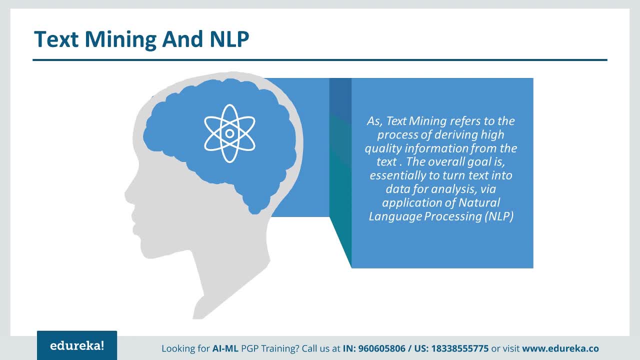 Whatever the text we are getting, natural language processing algorithms internally is going to create some kind of a structure internally how the words are similar to each other, how many they are coherent to each other. What are the verbs in that? what are objective? what are nouns? how they are getting used frequently. 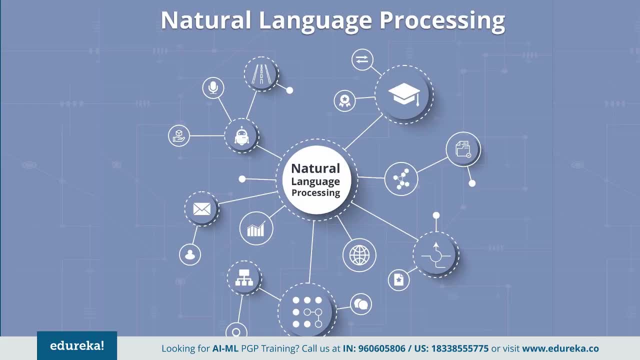 but it's going to map all this internally, So natural language processing can be used in any of the fields, maybe on the internet, maybe in the colleges, maybe in the housing industry, or maybe retail, maybe sales, maybe emails, maybe some kind of external file reading, maybe some kind. 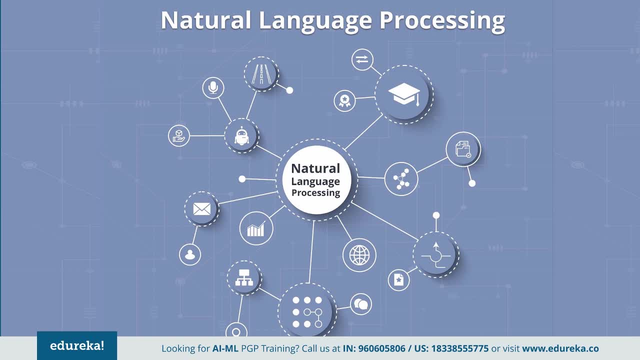 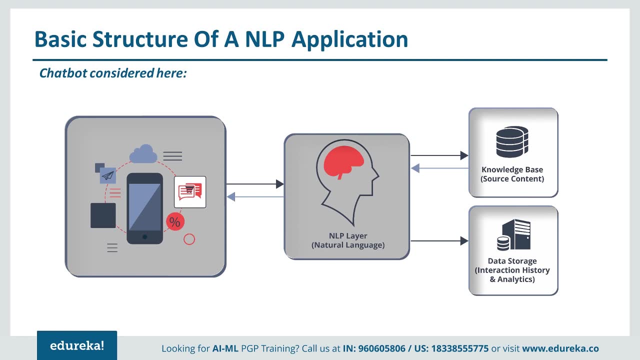 of a graduating on a subject. So natural language processing is something which is required anywhere. What is NLP? the basic structure of NLP applications? Let's say chat box. consider here, So the chat box. the data is coming from different sources: by email, via cloud, via presentation, via some calculation. 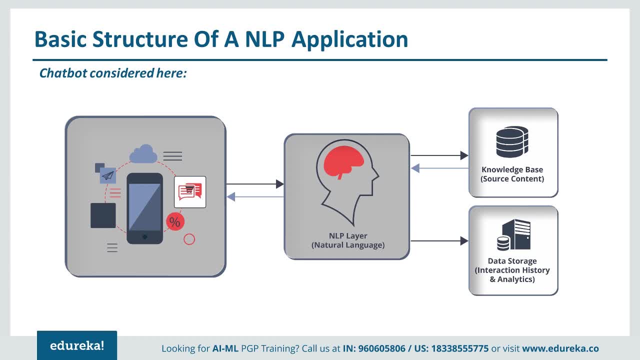 or whether from system tablet. So it is taking the information into NLP layer- that is also called as natural language processor layer, and once data is there in NLP It is going to search and knowledge-based source, knowledge-based source content and it is going to search and data storage. 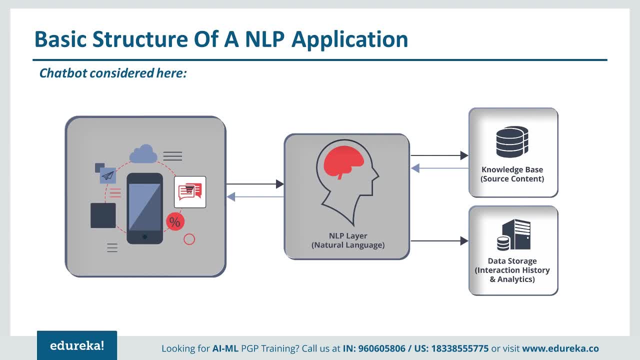 internal history. on analytics, The two types of search NLP is doing, one is called knowledge based search. knowledge based search means already existing libraries in LLTK. So there are chunks of libraries and LLTK wherein it is going to search for a particular word. 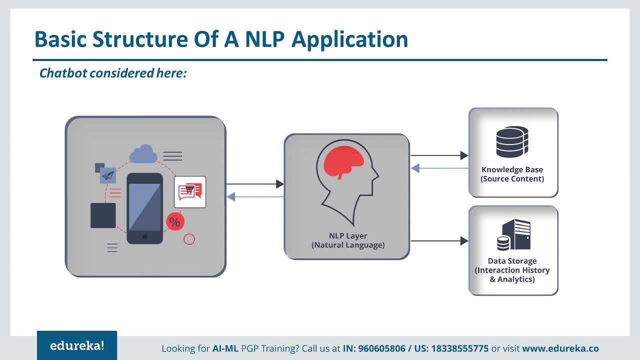 Suppose I say I am going, so going is a verb here. It is going to check internally wherever the going word is coming, What is the meaning of it, in what context person is saying I am going. then it is going to check the historical data. 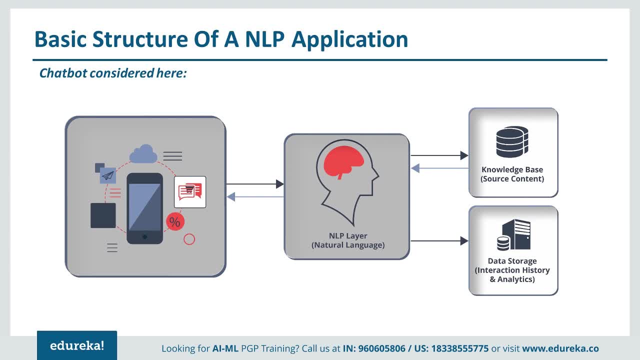 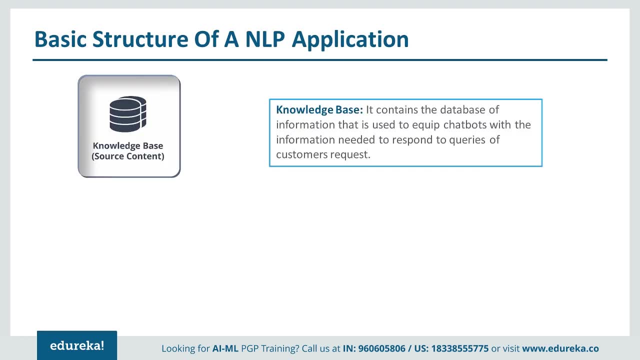 wherever going, word is coming in the historical data. What was the context there? and trying to map up with a situation where historical data is going to match with future data. So this is the architecture of NLP: knowledge-based. contains a database of information that is used to equip chat box. 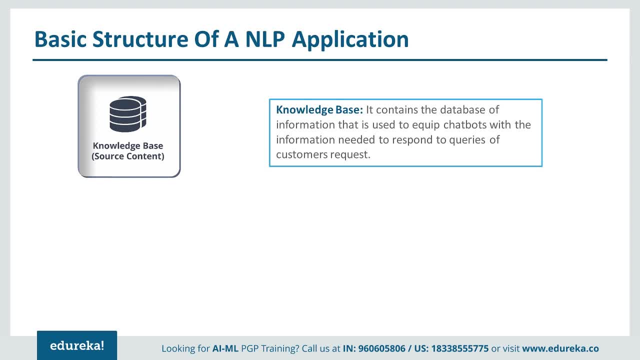 with the information needed to respond to the queries of customer request. So knowledge-based means, depending on the question system, is going so giving some answers. It has got some intelligence in that, for example, when you log into ICC Bank and you say I want a balance inquiry. 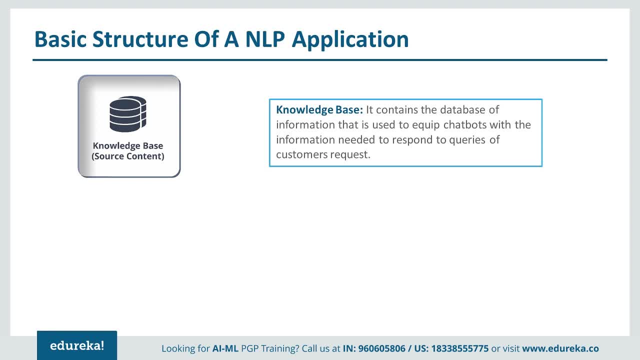 but picks up the word balance and based on that, it is giving you options. So might have seen this, but they want a current account balance or a saving bank account details. So, based on that, content-based filtering is done and it is taking some decisions. 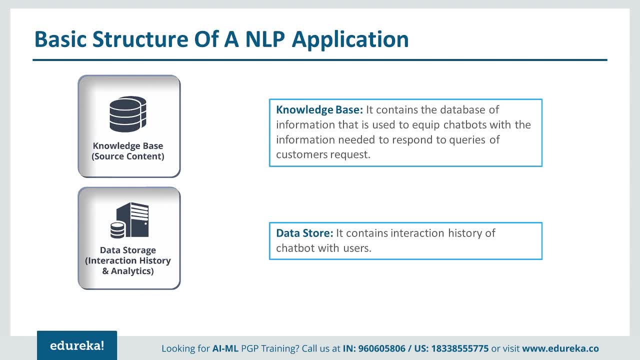 Second is data storage. So once that it contains interaction is to have chat box with the user. once interaction is over with the chat box, It is going to store it for the future learning so that algorithm can improve day by day. So whatever the discussion is happening on the chat box, 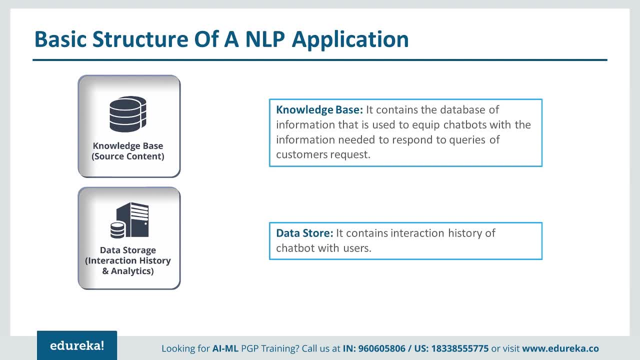 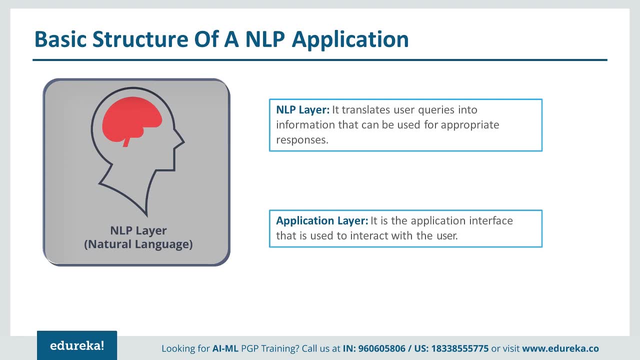 it get archived, it gets stored in the repository and people in the back and they do more research on that right of data. what user is providing? and improve the algorithm. Now there are two layers: NLP layer: It translates user queries into information that can be used for appropriate responses. application layer: 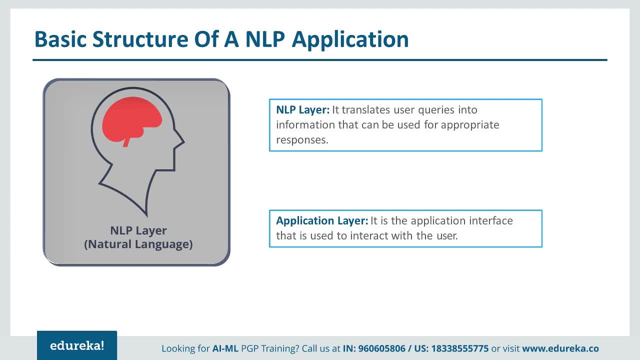 It is application That is used to interact the user. So basically there are two layers, or you can say there are three layers, like in Unix shell scripting. What we do, we have a code that is hardware. hardware interacting with what shell hardware is interacting with kernel- kernel- 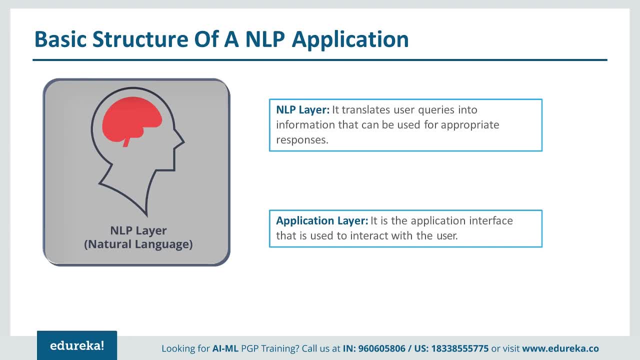 is interacting with shell. similarly here, whenever you give some language or text to NLP, it comes to NLP layer, which is used to translate the queries into appropriate responses. So what it's to internally, it is going to check the question, what you are asking for, the chatbot comparing it. 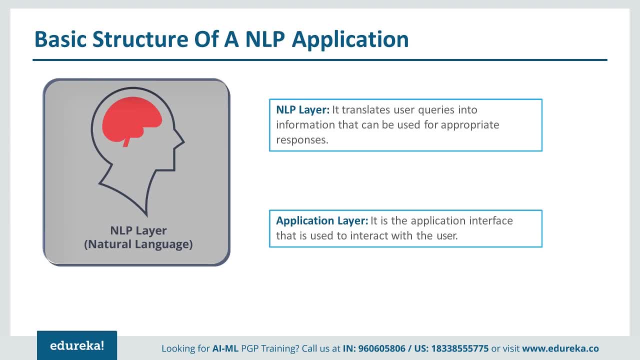 with a historical data, what it has, similar type of question and based on that It is giving some results. So the application layer, user application interface, used to interact with the user. So in the back end the information has been fetched. Let's say, if you say, what is a seat number for some PNR? 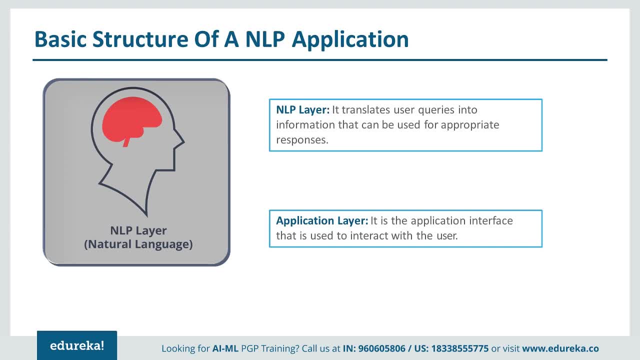 So seat number is a keyword here, PNR is something keyword. So it is going to filter internally PNR and keywords from some external file or maybe at the application layer. It is going to give you some results on the screen that is known as application layer. 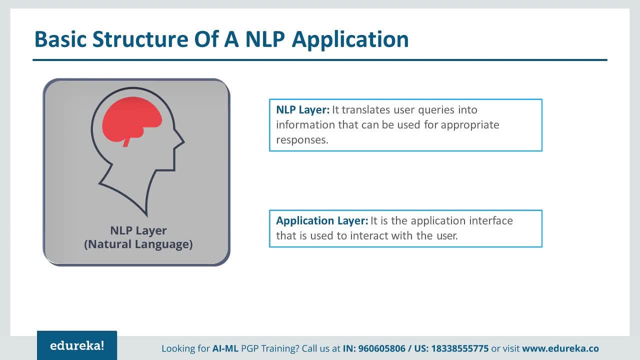 So NLP layer is basically used for mapping the problems with the solutions, and application layer is just for the interface with the end user to show the results to the end user. So we have an NLP layer. translates your queries into information that can produce appropriate results. 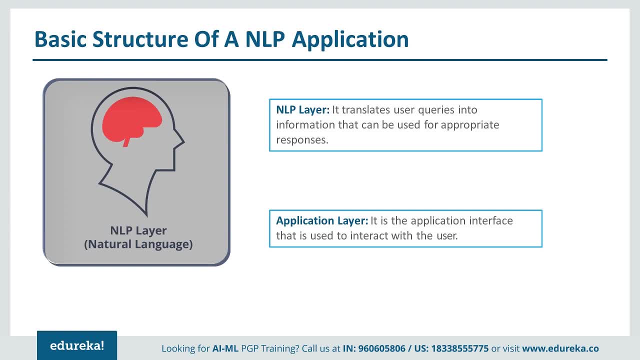 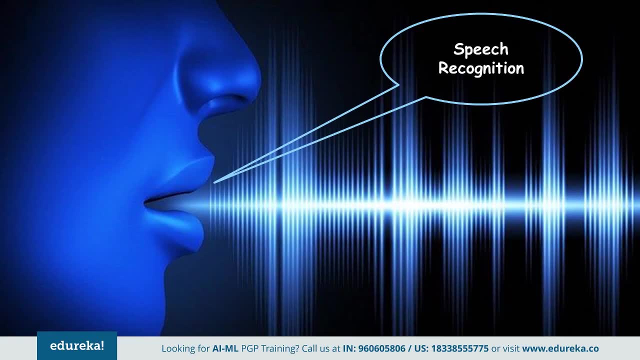 and this application layer, which is kind of an interface where you get the results. What are the different applications of NLP? Where do we use natural language processing and day-to-day life speech recognition? This is one of the most promising features of NLP is. 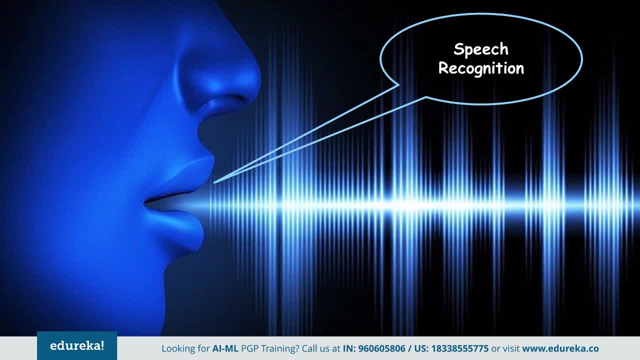 that whenever you speak, something system is going to record that and we can work on the recorded audios or videos and convert the text, whatever the you are speaking, into a sentence or maybe a paragraph and, based on that, taking some decisions. So one of the live examples is: you might have seen Alexia. 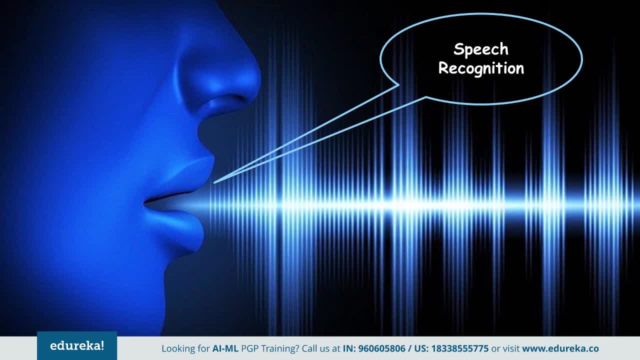 That is a music player that is quite popular in Amazon. you say, okay, Alexia, why don't you play a song? and you give the name of a song and it is going to play that song. So how does doing it is recognizing your speech depending? 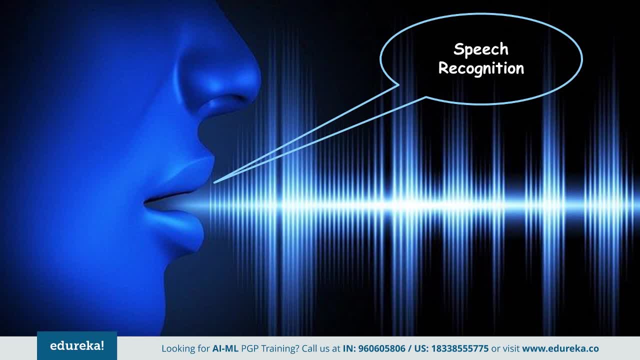 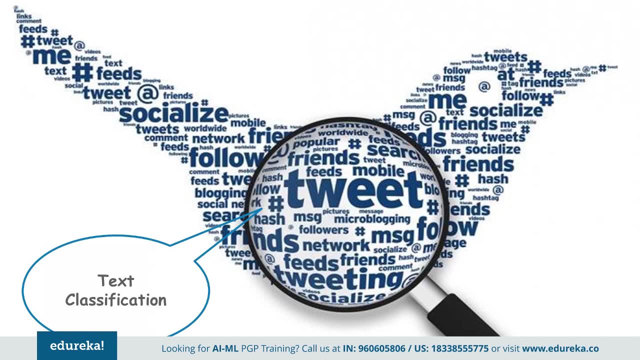 on what words you are saying. it is filtering it out, looking for the results over the net or maybe on the repositories and playing that song. So one of the application is speech recognition, text classification. So whenever you are writing some text, maybe on the Twitter, maybe on the Facebook, 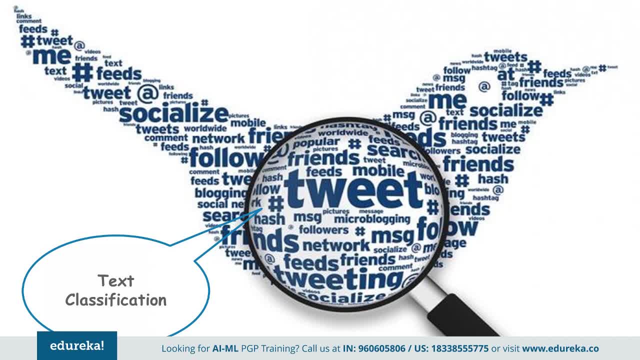 Or maybe on the WhatsApp, whenever you send some text, there is a sentiment analysis. So sentiment analysis is what sentiment analysis? finding out the classifications, kinds of classification problem, where in you classify the text based on positive or negative words maybe, or maybe some kind of a keywords. you are finding out the tweets. 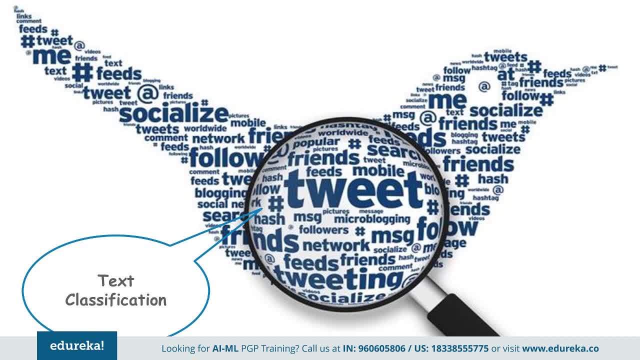 and filtering out the records from there. So, for example, if I say whether Ford is more popular or Honda is more popular, if I have a question there in my mind, I suppose let's say I want to open a new store which is going to sell. 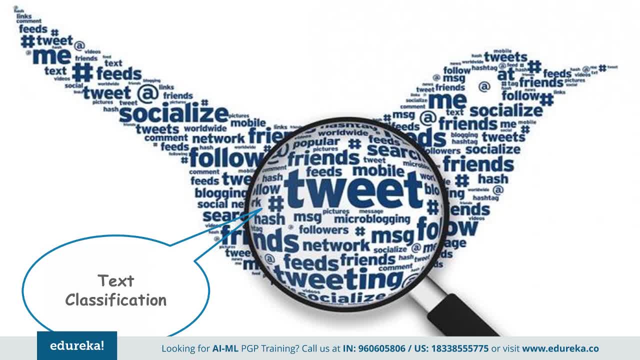 a set of pizzas, while asked in the locality whether pizzas are more common the people are buying, or whether it's a bread which people are more buying, or whether it's a fruits which people are more buying. So you get a results based on this kind of a criterias. 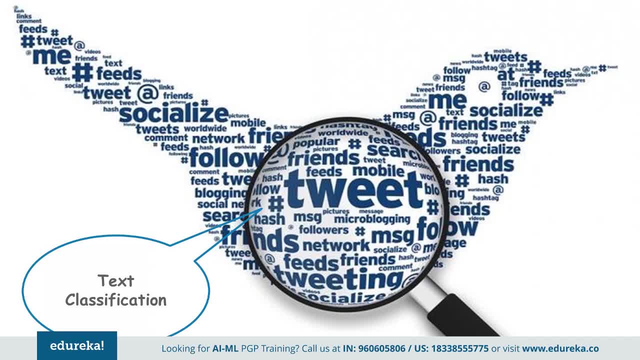 from the text that you already have there in case, For example, if Ford is more popular or Honda is more popular. you see the Twitter tape tweets and you'll see the positive words there on the tweets, whether people are saying good responses about Ford, and we are going to do a sentiment analysis in terms 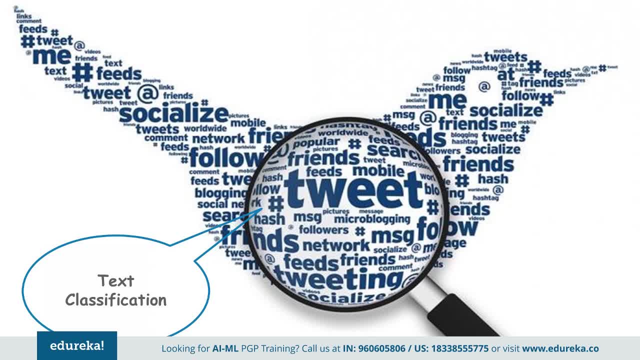 of the objectives which people are using, So like, for example, people may use for the, Ford is good, Ford is excellent, Ford is having the great efficiency of Ford. mileage is really excellent, So these are all positive to it. Somebody can say Ford is not a good value for money. 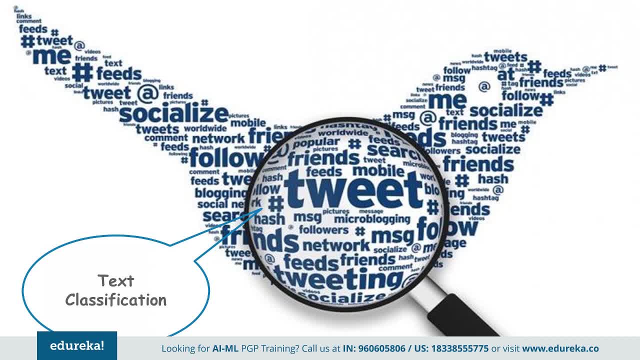 or it is not that good or it is having some worse characteristics. So these: you get a sentiment analysis on the negative words and based on that you are filtering out the data into a pandas data frame and then count the number of positive words people are saying. 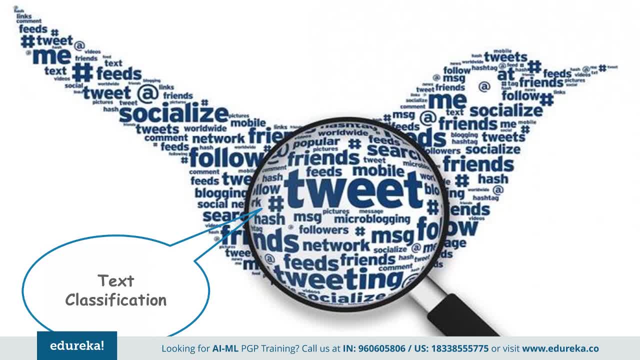 and count the negative words which people are saying and then you're doing final decision. Okay, these are the hundred tweets which I filtered out. hundred seventy percent people are saying good thing about the particular word and 30% people are saying negative things about this word. 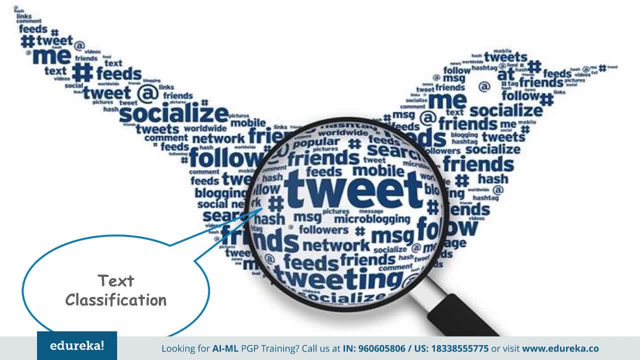 So we can say Ford is more popular as compared to Honda. So this kind of a decision-making generally people do for business analytics and that is one of the text classification: classifying the text based on their characteristic, whether it's a positive or it's a negative. 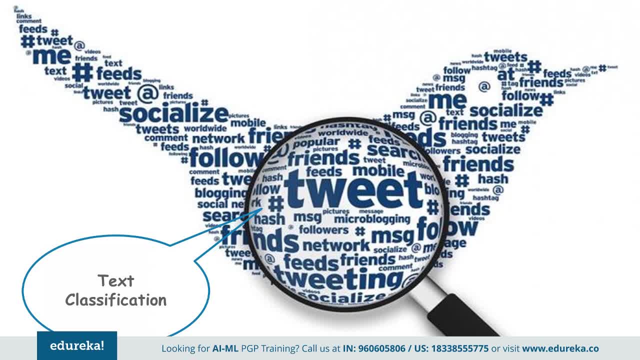 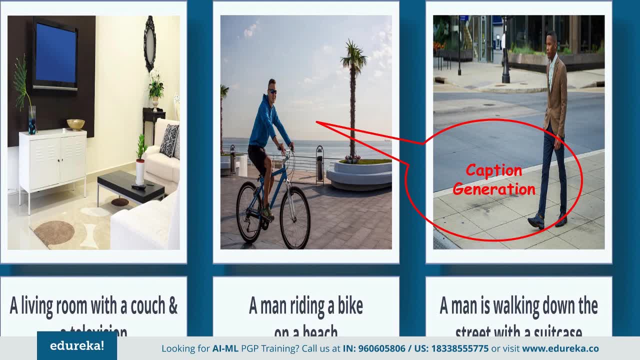 or maybe it's an objective, or it's a noun, depending on the kind of search you are doing, maybe in a form of our image caption generation: a living room with a couch and a television, Riding a bike on a beach, a man walking down the street. 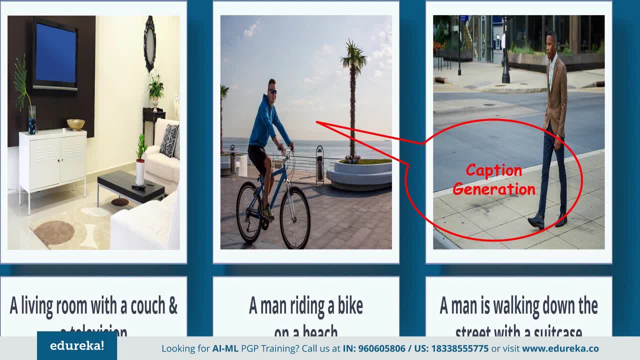 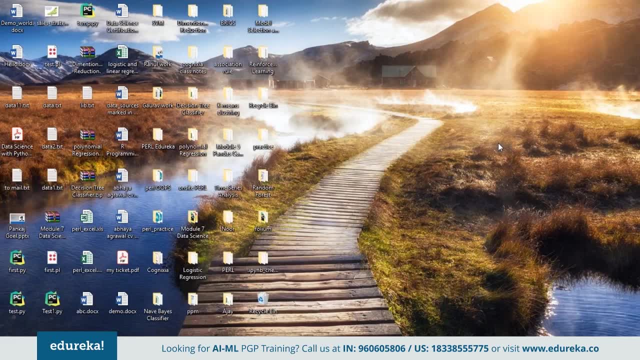 and suitcase. So there's something which is comes in the reinforcement learning. where manless cars are there, It is taking the image, capturing the image, converting to vectors and taking some decisions. So let me explain you the different types of learning mechanisms. So first type of learning is known as a supervised learning. 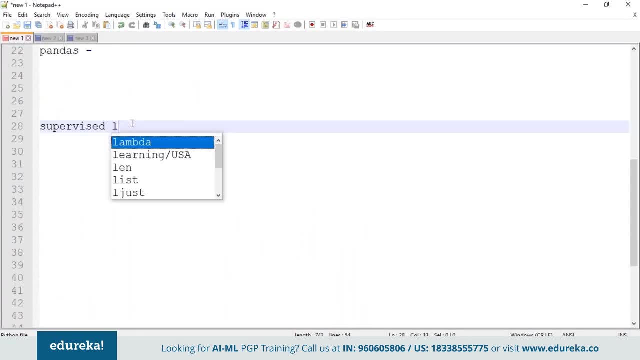 Let me write down here. I'll tell you the exact differences in them: supervised learning. supervised learning has column headings, So any data which you get has column headings is known as supervised learning models Like, for example, we have a rainfall, We have a humidity, we have a temperature. 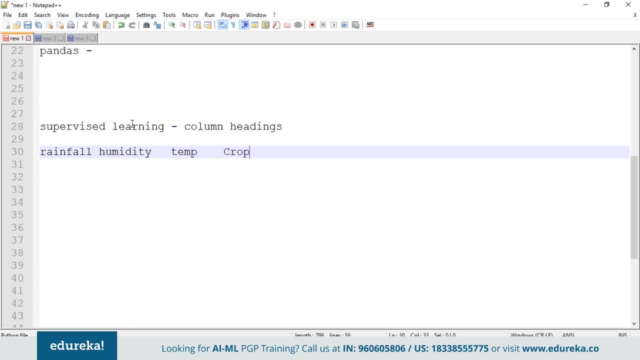 and based on that, we have some dependent variable called crop yield. So here we have three independent variables, that is, rainfall, humidity and temperature, and we have a dependent variable called crop yield. Now we want to find out a relation between rainfall, humidity and temperature with a crop yield views. regression analysis. 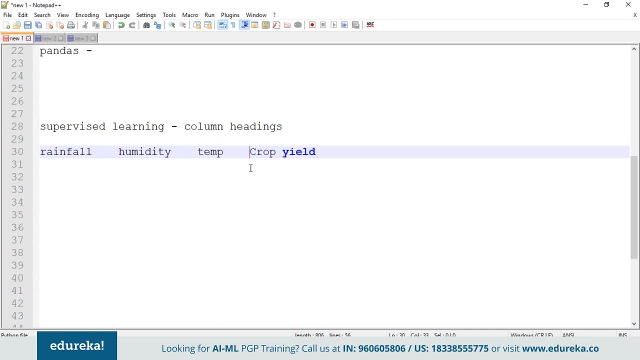 Maybe to find a relation between rainfall and crop yield, humidity and crop yield and temperature and crop yield. So we have a column headings, We understand the data completely and that type of learning, where we do, is known as a supervised learning, where we understand the data completely. 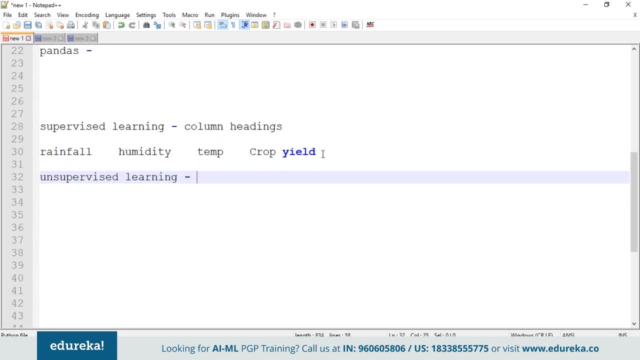 second type of learning is unsupervised learning, where we do not know the data, We don't have column headings. For example, if I give you some numbers- 1, 3, 5, 6, 8, 10, 12,- it can be height of a person. 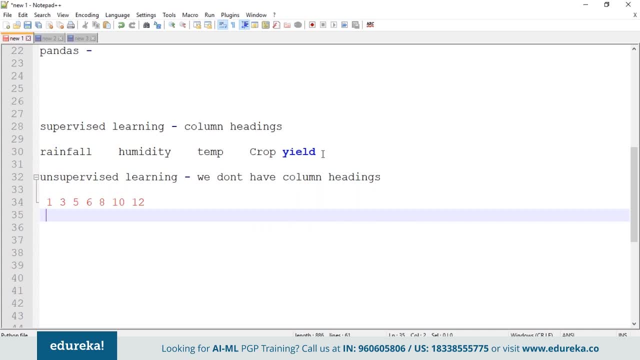 It can be weight of a person, It can be kilometers We have driven, it can be anything. now, if I want you to cluster them in two different groups, So I'll do. you may be using a k nearest neighbor algorithm. You may be using k means algorithm. 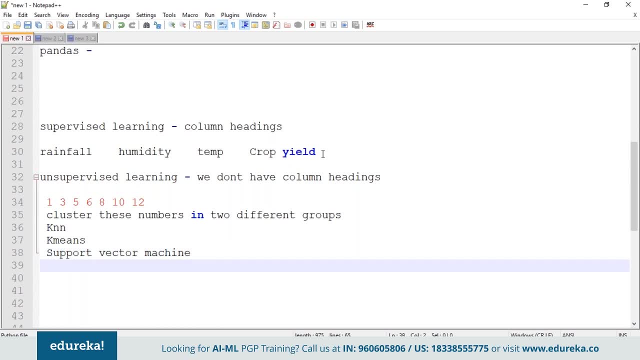 You may be using support, You may be using vector machine and you classify the data based on some common characteristics or maybe the mean value, with what all values are nearest to the mean value. So unsupervised learning example can be: suppose an archaeologist find a bone deep inside the earth. 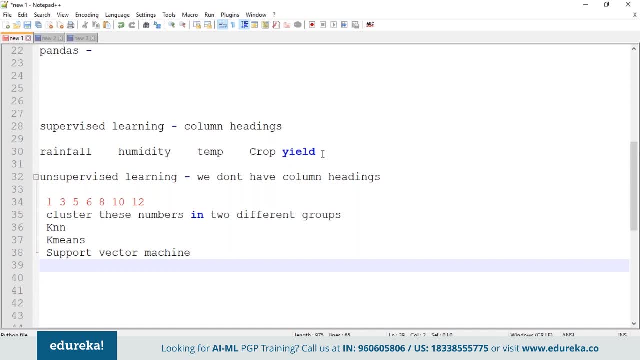 We do not know anything about the bone. He do not know whose bone it is. So what he'll do? he'll find out the feature vectors from the bone. He will find out the shape of the bone, color of the one, texture of the bone, size of the bone. 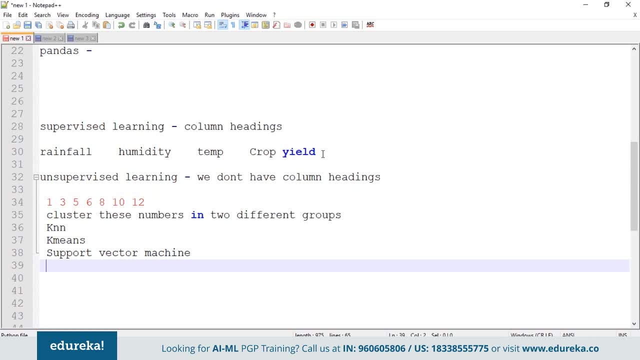 and based on that it is going to match the historical data and compare whether the bone is most likely matching to the dinosaur or a human or us, any other animal. that is known as unsupervised learning. So reinforcement learning is basically a learning by experience learning. my experience simply says that you have certain problem. 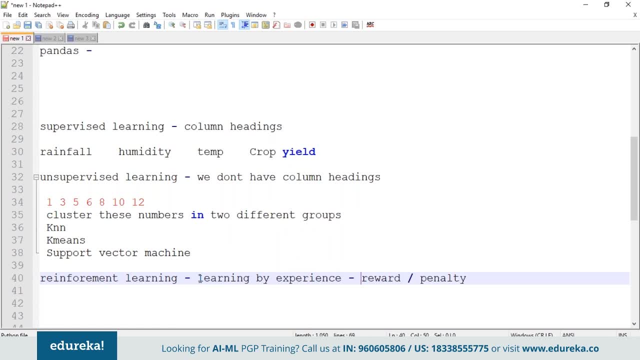 and you find a solution for the same. Once you find the solution, you put it in the repository and next time the problem comes again. You use the same problem, you same solution, again and again. So reinforcement learning is learning. my experience, Let's say, feed in in my system hundred images about the roads. 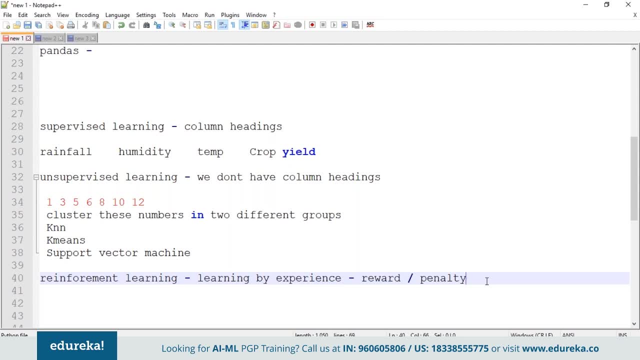 roadsides and the red lights and let's say, I want to have a car which is a self-driven car. So it is going to see the images and, based on that, we feed in some decisions into the system that if you see a red light, you need to stop. 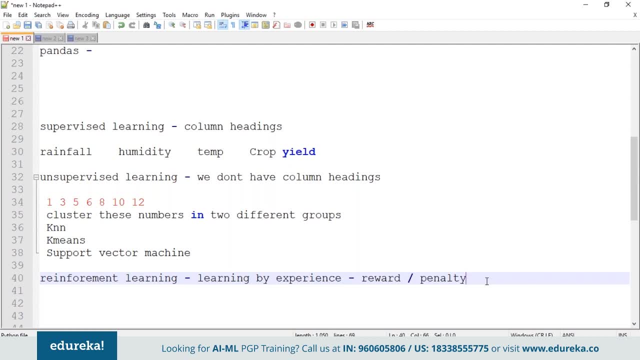 if you see a car ahead of you, you need to stop and based on that, it is running the algorithm and taking some decisions. Maybe after some time I have a thousands of images coming more. I'll feed in into the system. I'll train my machine again to learn those images. 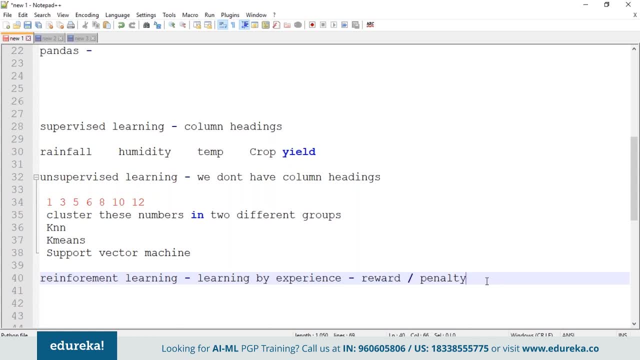 and, based on that, some actions and similarly. suppose I have a 1 million images, I'll feed into the system and training the algorithm. So every time, what we are doing, we are learning from the experience, means we are taking some decisions, whether we are taking some positive rewards. 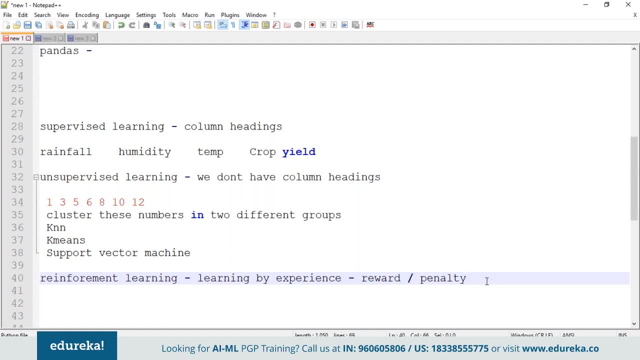 out of some actions, or negative rewards out of some action, and slowly and gradually system become robust. So one of the typical examples of this is aerodynamics or maybe autopilot. So you might have seen in the airlines Most of the flights are run by autopilot mode. 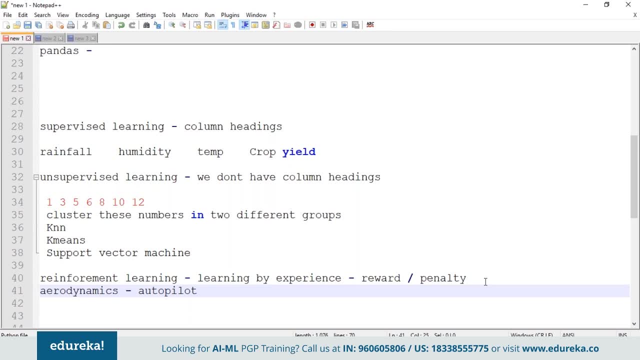 and why it is so? because it's the most safest way of driving a plane, because aerodynamics or autopilot system automatically knows, like if the air pressure is this, humidity is this outside, or maybe rainfall is there or not, or temperature is down, What to take the action. 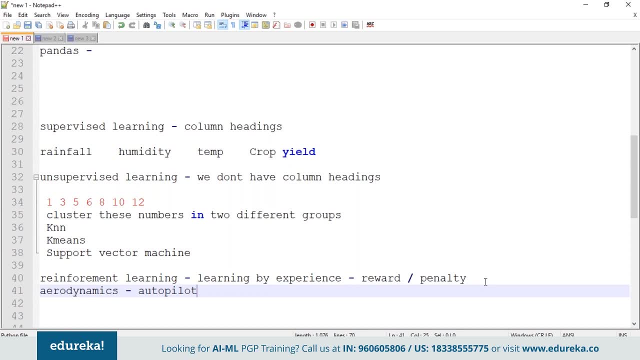 human may not think of those thousands of permutation combinations, but autopilot knows what needs to be done, So there is known as a reinforcement. learning system has become mature after learning so many years all permutation combinations about the weather, and in future something comes up. 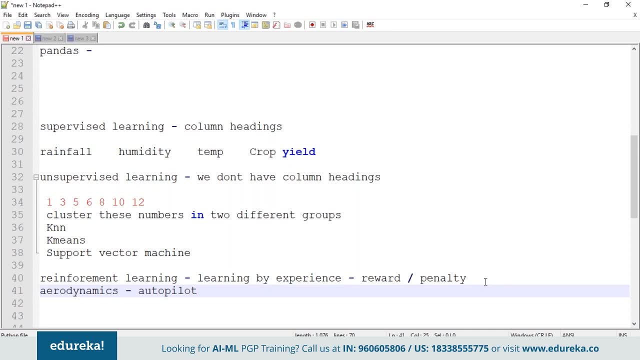 He already knows what needs to be done. So reinforcement learning is a basically learning by experience. supervised learning is when we know the data, completely unsupervised something when we don't know the data, we want to find the feature vectors. For example, if I give you a fruits, 10 fruits. 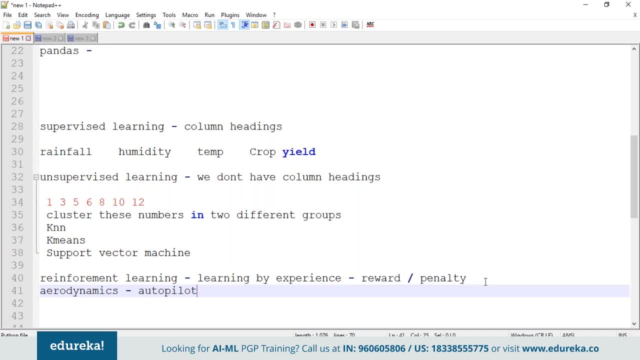 and I'll say, classify these foods. So how you classify based on color, you are going to classify based on shape, based on texture, based on weight and lot of parameters, what you can think of. and once you classify based on these characteristics, suppose new fruit is going to come to you. 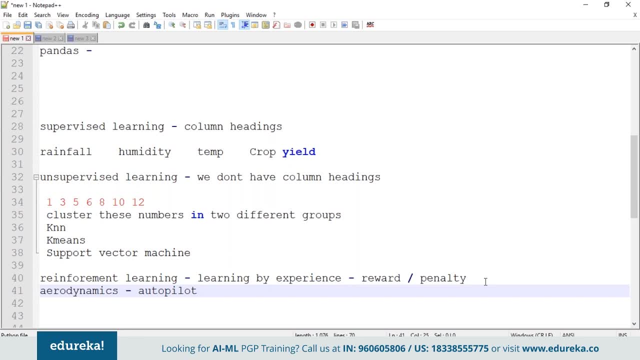 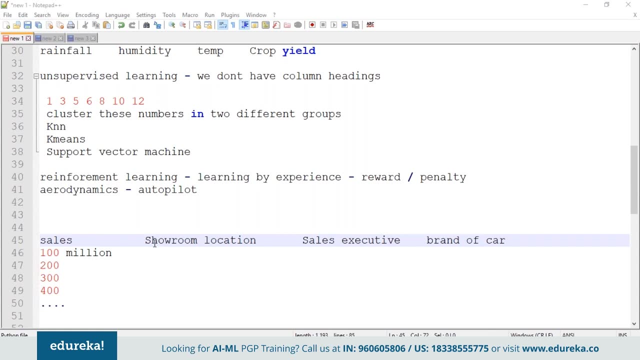 You are going to classify correctly, saying that. okay, These are the characteristics of the foods there. with me, It is most likely matching to the other food. that is a learning call: unsupervised learning. So these three types of learning has to be really good with you. 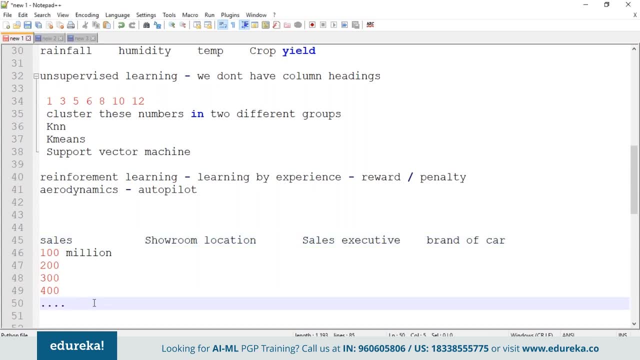 If you really want to work as a data scientist and want to go for a natural language processing was. these are basic algorithms. Now my question comes here. Let's say you have a rainfall, temperature and humidity. Let's say I have a rainfall as 100 mm, humidity 60%. 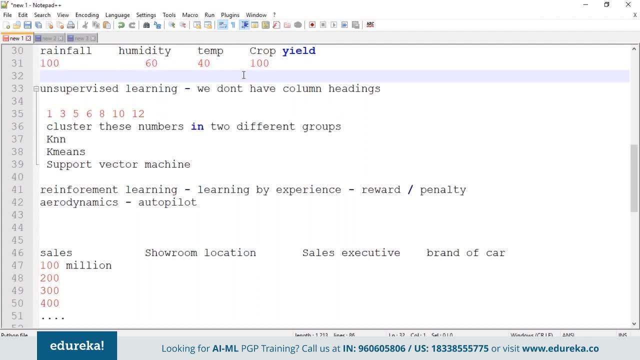 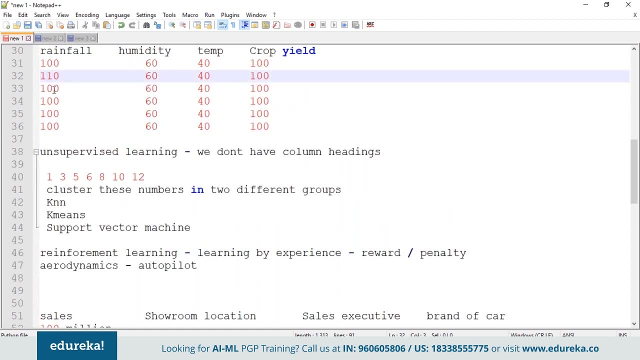 and temperature is 40 degrees, crop It is 100. and let's say you have some dummy data like this: historical data, maybe for last 10 years, Maybe you have certain changes in this. Let's say, some historical data, maybe 70, some random data. 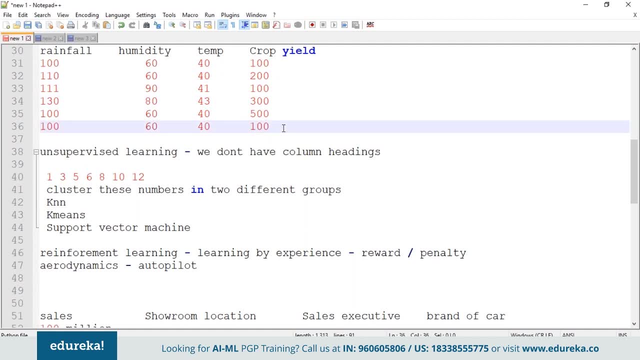 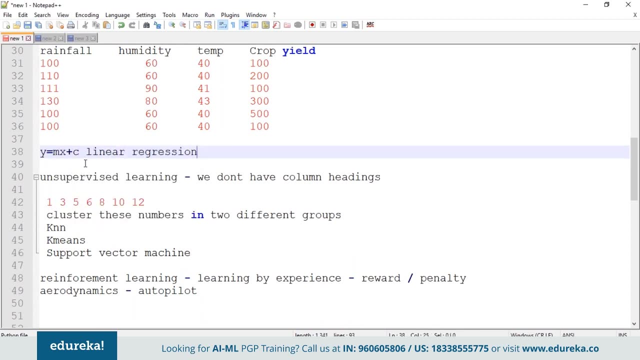 maybe some random data. Now my question here is: let's say you have a historical data and you made a question of a line Y equal to MX plus C and use a linear Regression here and your model is ready which is running on linear regression. 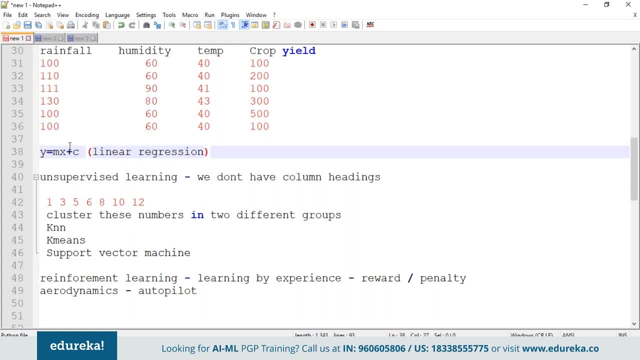 and based on this linear regression, maybe you take a rainfall. Let's say: and based on the rainfall, let's say you have a 200 mm rainfall and you want to predict the price, predict the crop yield. So easily with this equation you can easily predict, because dependent variable is Y. 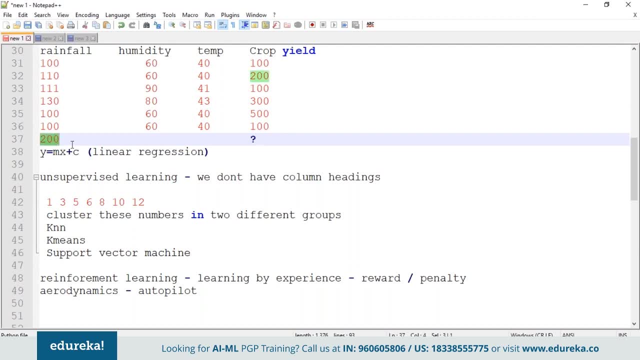 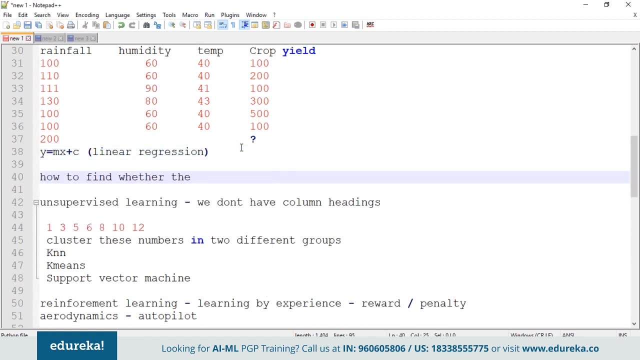 So X value you already know. slope, you know because you have done regression analysis, intercept. you know now how you find the accuracy of the model, how to find whether the results or the equation you made Is giving right predictions. How can we show that the model which you have created? 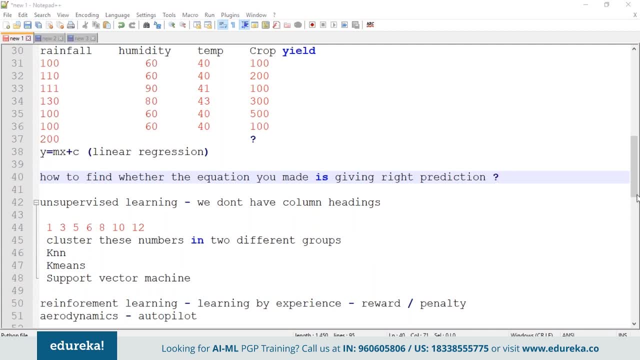 is giving right predictions. Suppose I predicted some value using this equation, How can we show that it is going to be accurate? So there is something called k-fold technique in machine learning. careful technique is doing What careful technique is going to divide the data. 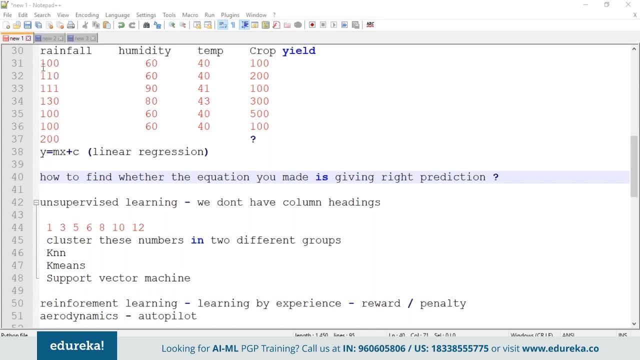 into number of folds. We say suppose I say careful. as for, it is going to divide the whole set of data into four parts internally. It takes the first part into testing and rest everything into training and the second one. It puts second part into testing, rest everything into training. 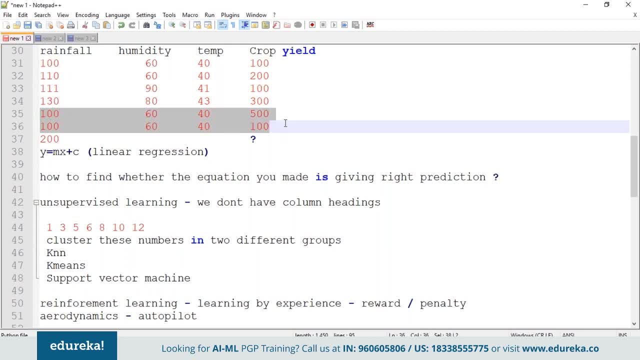 in the third part. It puts third part into testing, test everything into training, find the accuracies of all the models and average them out. That's the best possible way, because if you do k-fold, you will realize that at any point of time one of the tuples will always come. 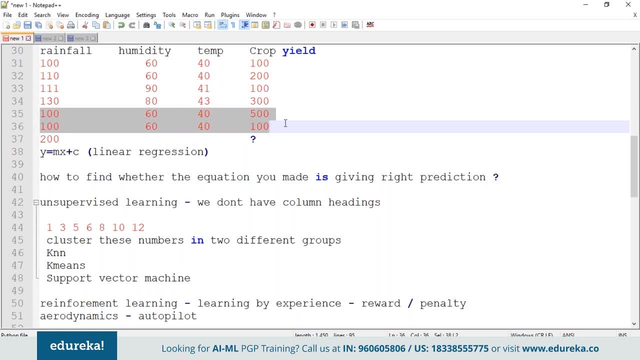 in training and testing both of them. So if you run this in like a fold, one row may come in testing at any point of time. It may come in training at any point of time. again, It may come in testing at any point of time. 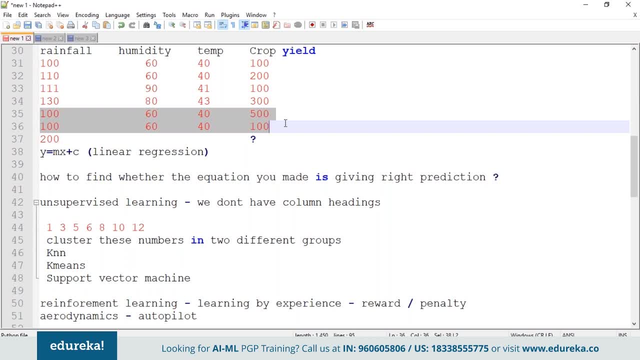 and you have covered all permutation combinations there. So careful technique is one of the best way. We divide the data into four parts of five parts or six parts, take every part into testing and rest of the parts and training, find the accuracy and go on, keep on doing it. 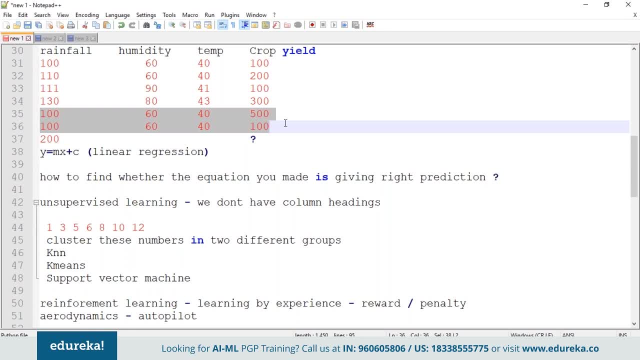 The system is internally running the k-fold algorithm and number of times, filtering out the data on the random basis in the testing and training, and run this algorithm maybe 10 times or six times or five times, depending on the k-fold value, taking the average out of it. 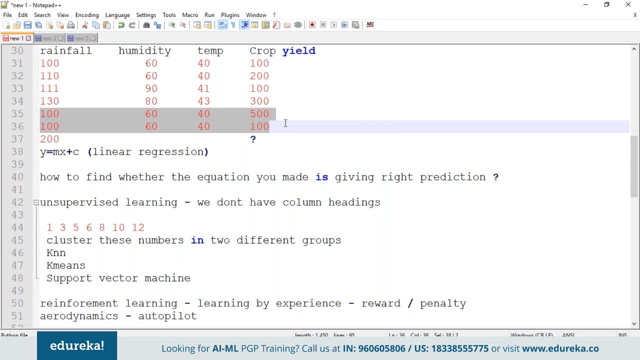 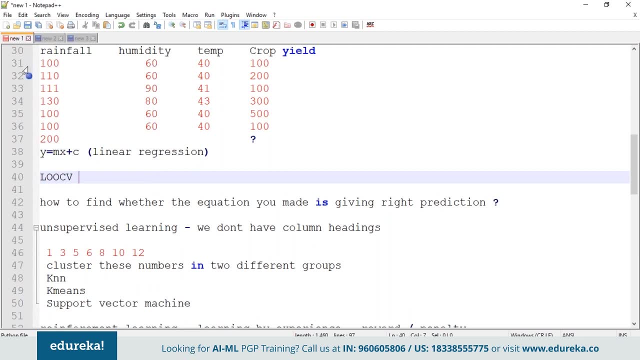 And that is the best accuracy which you can achieve from the particular worth of. there's another technique called look of technique. look of technique takes every row into testing and rest all the rows in training. in the next one It takes into testing, rest all the rows in training. next run: 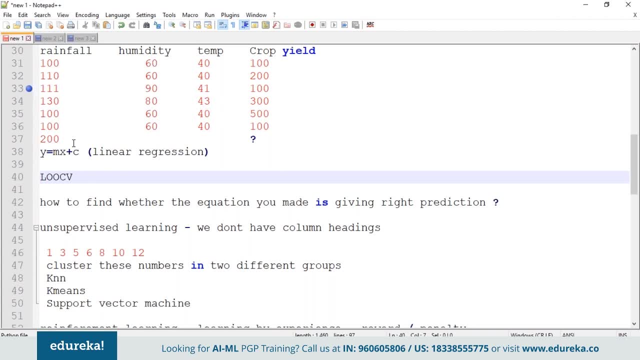 It takes the third row in the testing, rest all the rows in the training and keeps on running for 1 million records, 1 million time algorithms and taking the average of all the accuracies. It's a very expensive technique. generally We don't use it because it's a very, very hectic. 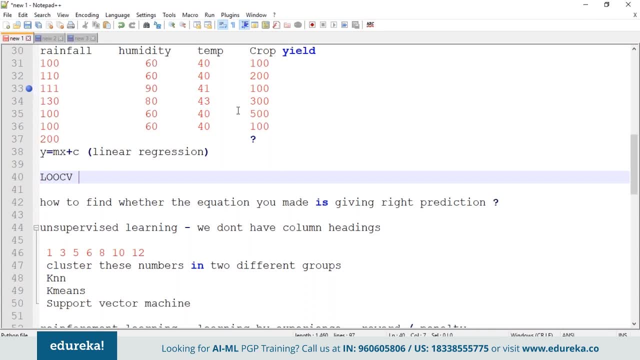 over very costly affair, CPU wise as well as time wise. So look, of technique is not very much supported. k-fold technique is which is very optimal. the other techniques as well- gradient search techniques and other techniques as well. We're in what parameters to pass we decide, like for example, 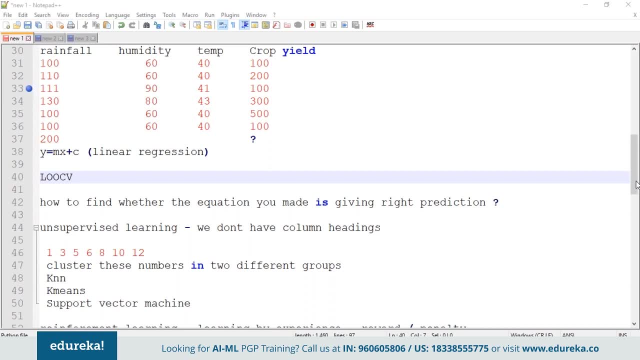 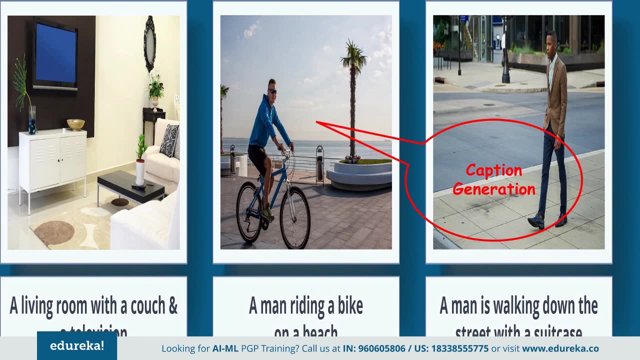 if you run random Forest, you pass the number of estimators. suppose the number of estimators are thousand, how you come to know whether to pass thousand or 500 or 10,000. So let's move on. So here we talked about a reinforcement learning. 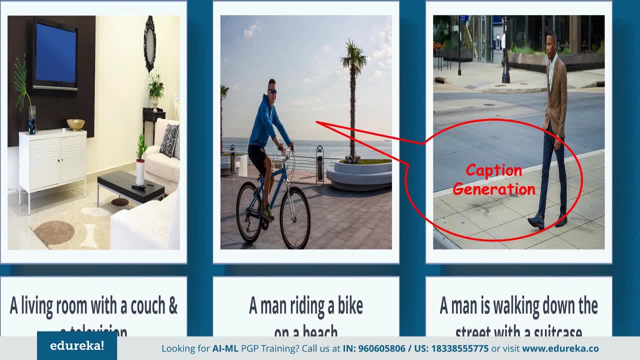 So reinforcement learning is learning from the experience. looking for the images, you decide, Okay, whether what actions to be taken depending on the images, and this is known as reinforcement learning. time to time system is fed in with the images. based on that, Some kind of additions, whether it's a positive reward. 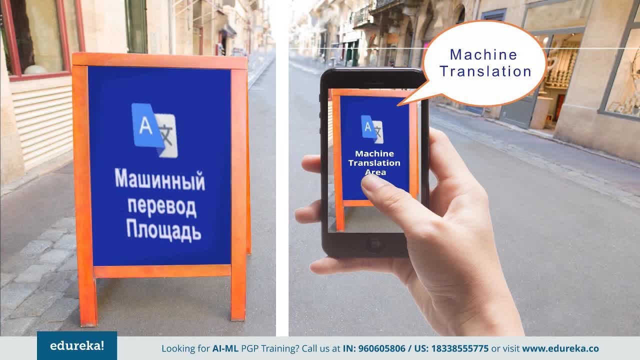 or negative reward and based on that system, is behaving. so machine translation is what? changing a text in one language into another language? That is again a kind of a machine learning translation. I would not say it's a completely machine learning. It's something like a mapping, which may or may not be having. 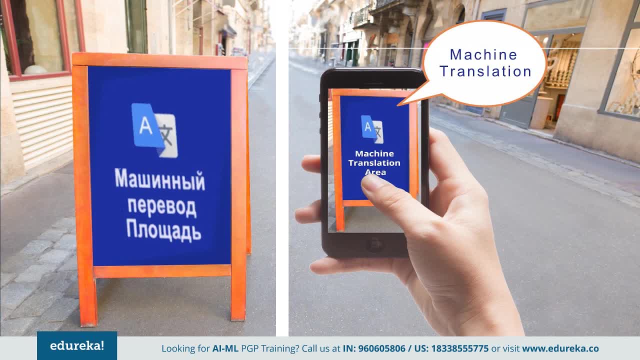 machine learning required in. that. machine learning word is only used when you do predictive analysis based on the historical data, You do some kind of a predictions in the future. That is the right word for machine learning. So this is just a machine translation. machine is translating. 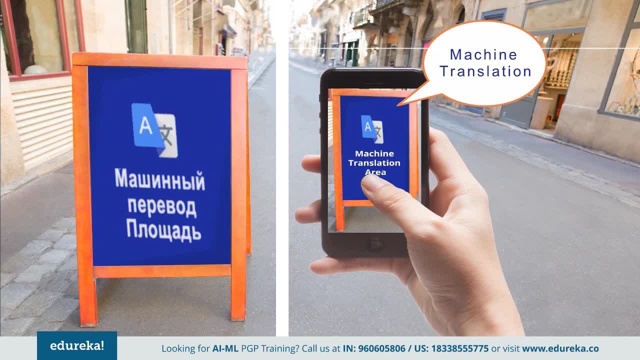 the word or sentence in other language to English letters. That is translation. that is not machine learning. So there's a difference in machine learning and translation. translation is simple algorithm which is running in the back and converting every word into a sentence, a word in a different language. 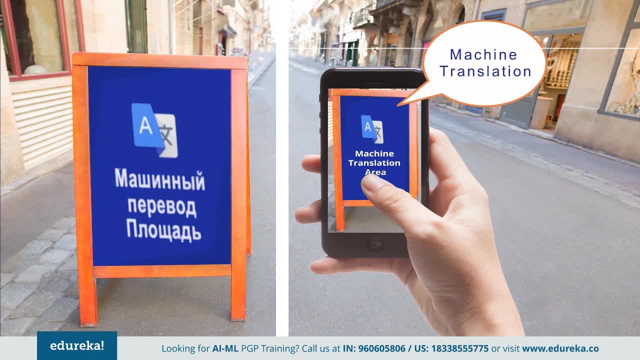 or different language. machine learning comes into the picture when you see the context of changing, when you see the context of changing means. suppose I say in English I'm going to Delhi and in some other language will say something in different language. So are you converting in the same tense? 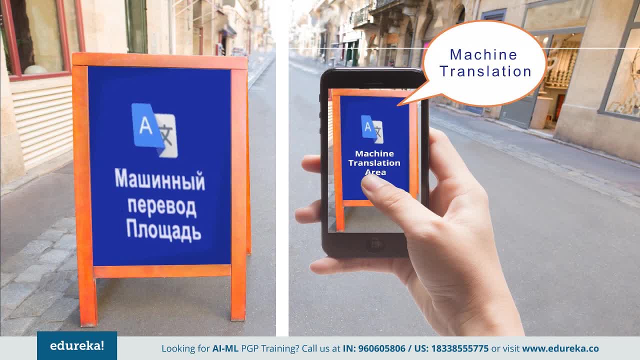 Are you converting with the same meaning? that is where the machine learning comes into picture: whether the context has not been changed. It should not be simply converting the words into English sentences or maybe one language to another. So we have seen what is machine translation. 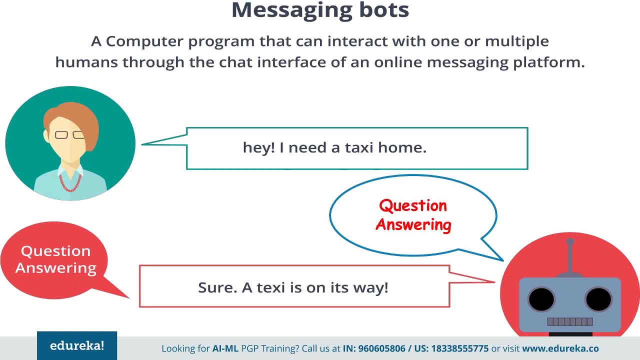 So computer program that can interact with one or more multiple humans to the chat interface on an online messaging platform. There is something called here: I need a taxi home show taxis on the way. So how does this chat box understand what you're saying? 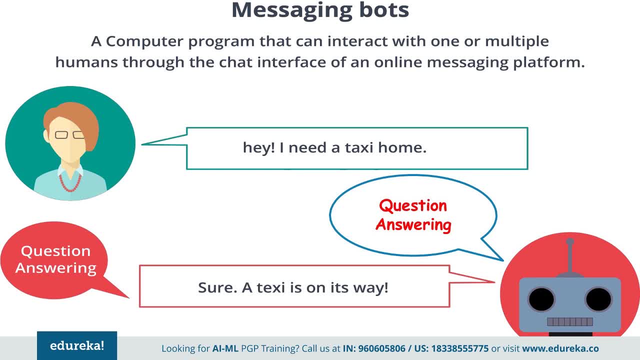 See, it is looking for the keywords, Like how the spam mail filtering is working. So if you know the recommendation engines or if you know the some kind of spam filtering kind of engines, what they do- they search for the keyword lottery or maybe you win the price of $10,000. 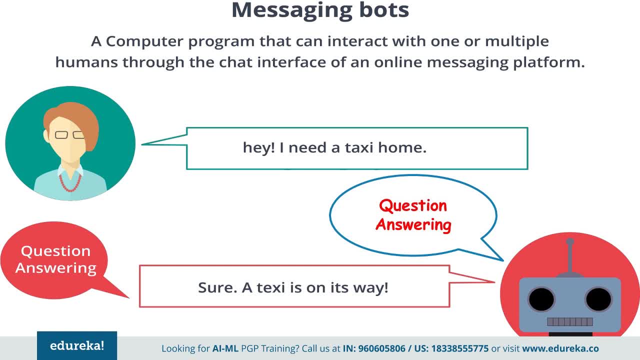 So, looking at certain text or keywords, it is filtering out the mails. Similarly, these chat box are looking for some keywords like, for example, need. so need is a keyword here which is telling the system that he requires something. some information is required then taxi. 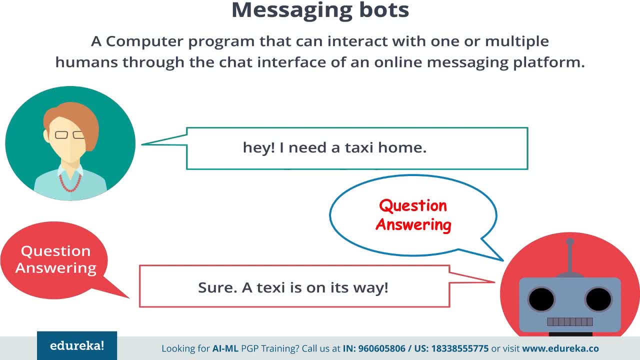 It is going to inference: Okay, he's looking for a vehicle and home, home is again like where you want to go. So the inferences which we are taking from this sentence, which we understand as a humans. that is a purpose of natural language processing, to understand the context. 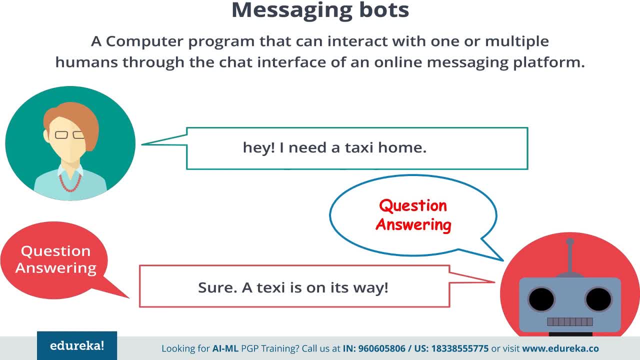 of the sentence, what it wants, rather than simple English words, finding out the relation between the words and finding out the context, what it wants to say. that is the purpose of an LTC. So these messaging bots and all is one of the examples where we use an LTC. 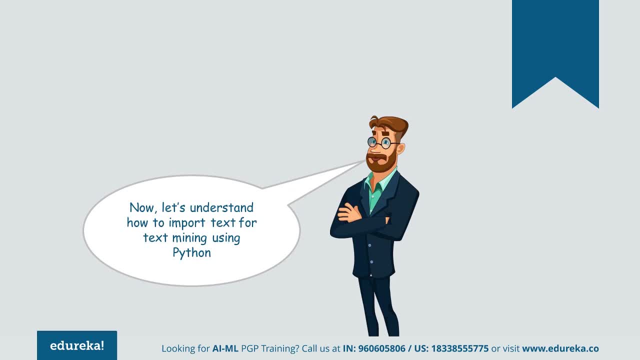 Now let's understand how to import text for text mining in Python, so that we are going to discuss about operating system library. So OS library is basically used for reading some external files. So a lot of file handling requirements to be done here. So how do we, how do we import external text file into Python? 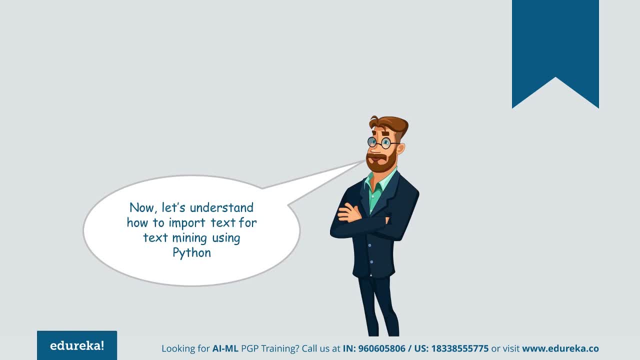 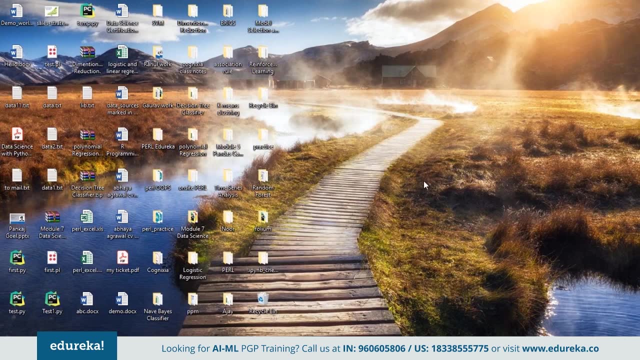 So once you open a file you have a lot of functions there in it, like see, tell or mode in which you have opened the file. So we'll see some operations on the file. external file, just to brush up. So there's operating system library. 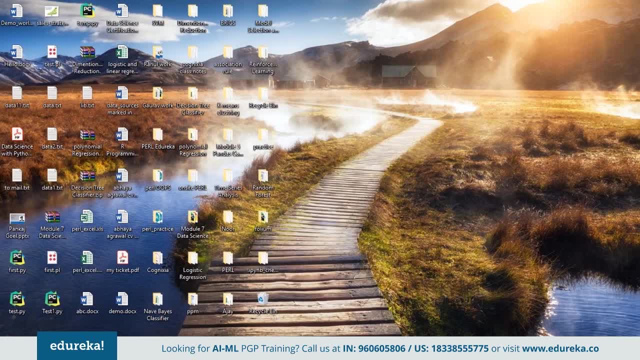 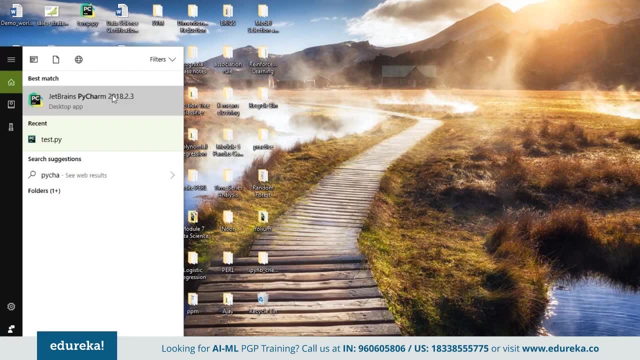 which is basically used for reading the external files, and this library is basically used for manipulating with the files in the operating system. So, for example, I'll take some example over here. So in the meantime, let's discuss about few commands of the operating system. 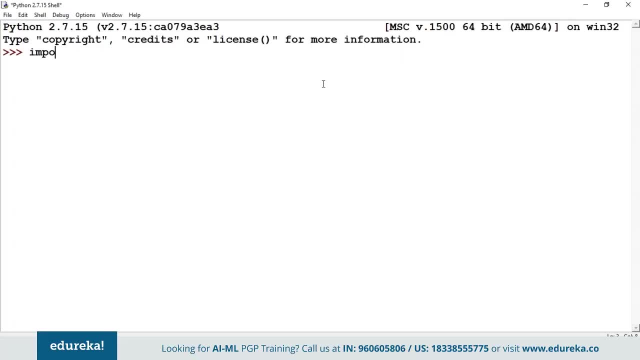 So you need to import our OS library. So this is a python idle. You already aware of this is a python idle. We are in, we can write down the commands like an interpreted manner and we get the results there and then so write: import OS. 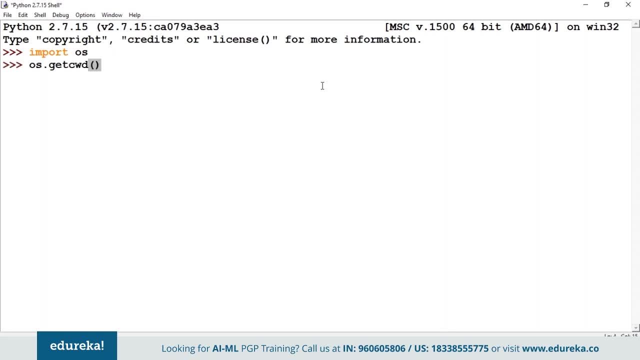 and OS dot get current working directory. It gives us the current working directory, which is C, Python, 27.. I can change it to some other directory- OS dot, CH, dir- and I change the directory, Let's say, to desktop. now OS dot get current working directory. 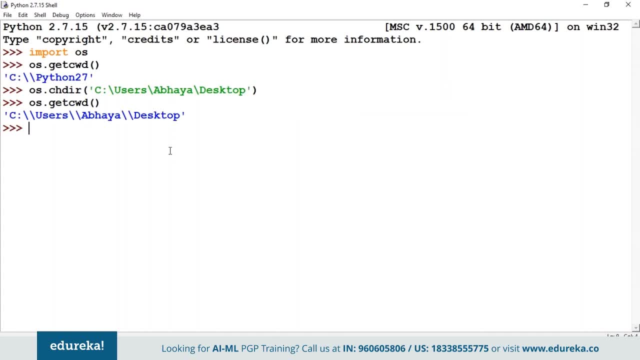 will tell me where exactly we are changes to desktop. Similarly, we can say OS dot remove, it is going to remove some external files. So if you'll write OS dot remove, it is going to remove certain file, and suppose I want to remove some file. 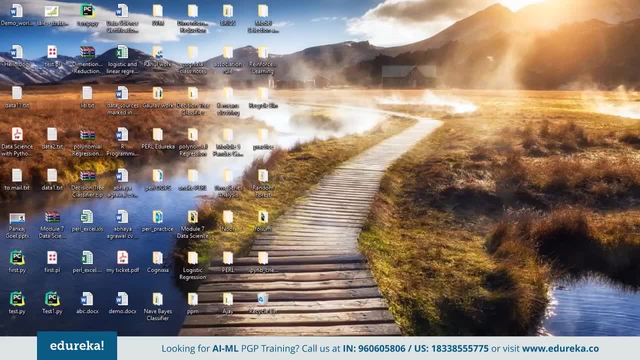 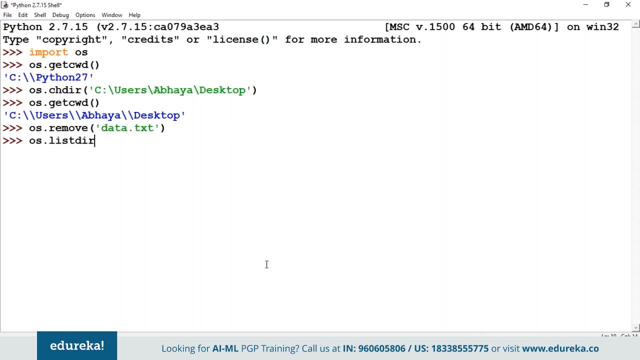 called data dot txt. So you can see data dot txt has been removed from there. So as dot remove is going to remove some external file. Similarly, we can say OS dot list dir and if I'll say OS dot, get current working directory. 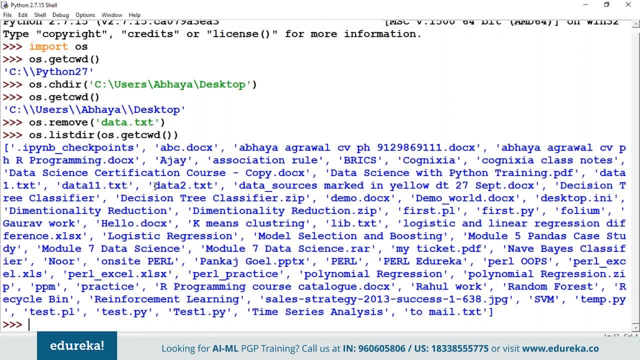 it will list all the files and folders in the current directory. So in my desktop these are the files and folders present there. So it is going to list all the files and folders present in the current directory. Now in order to work on files. 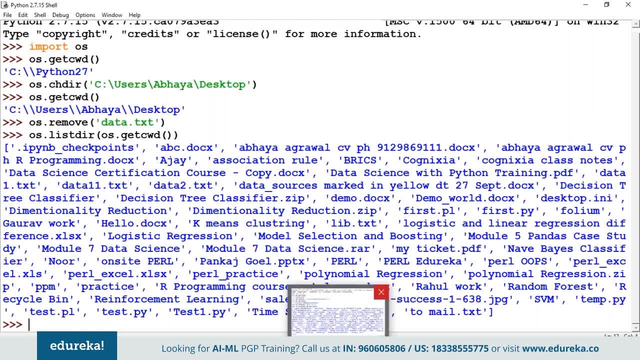 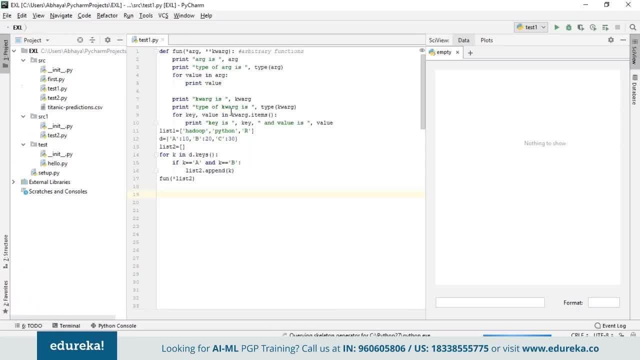 we need to open the file and we need to read the contents of the file. That's the first step, because maybe your data is coming in a text file or a word doc or a PDF for document. The first step would be you need to read the some external files. 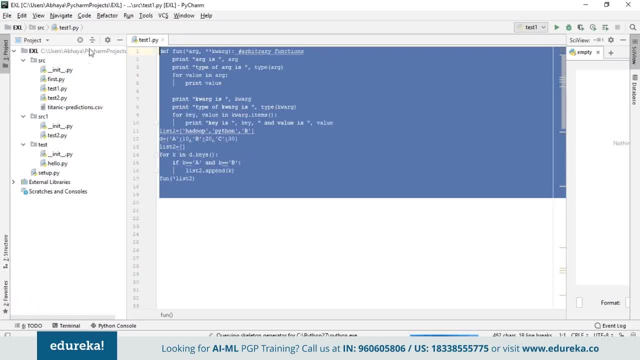 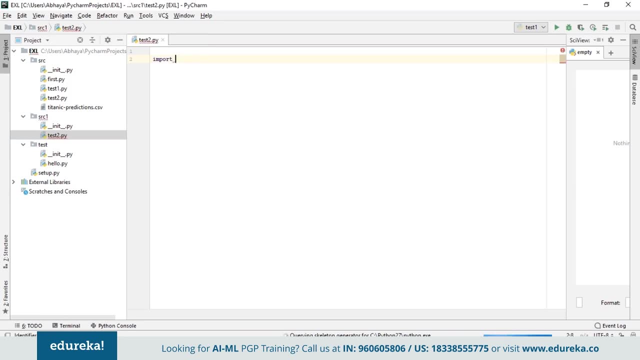 So how do we read some external files? Let me show you the results. suppose I say, or let me do it in some Other program. So how do you read external files? Suppose I say import OS, let me increase the font size, So I read some external file. 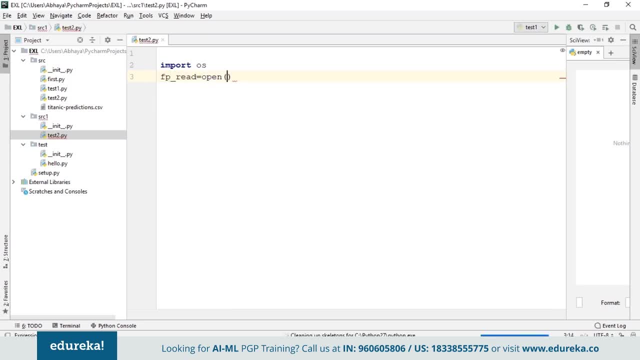 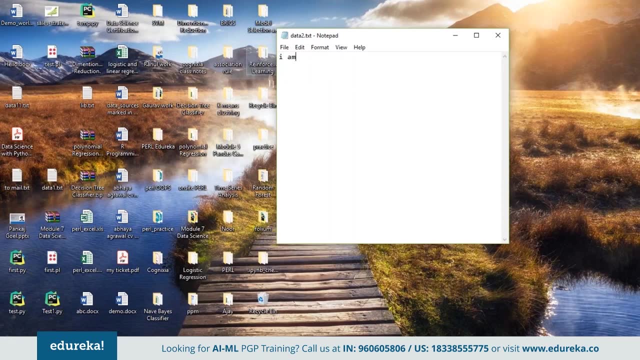 I'll say file pointer read equal to open and I'll give the path and I'll say some dummy file there with me, data to dot txt, and I write down some contents in this that I am working on, Python. Python is fun to use, So I'll read this file: data to dot txt. 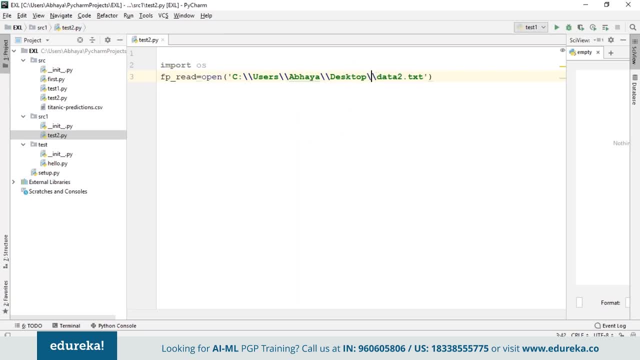 So in Windows machine we need to give double slashes to override the special meaning of slash. and I'm going to read this file in the read mode and I'll say for line in file pointer, read print line and I'll close the file pointer So it is going to read the external file. 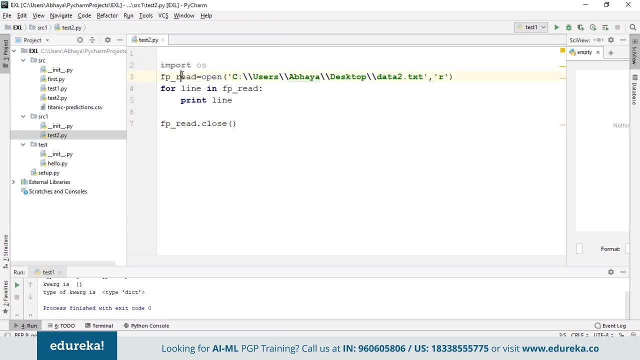 So if I'll run this, so it's a wrong file which I've run. I'm working on Python. Python is fun to use, So it is going to print line by line all the contents of this file. Now we need to check whether the file pointer is closed or not. 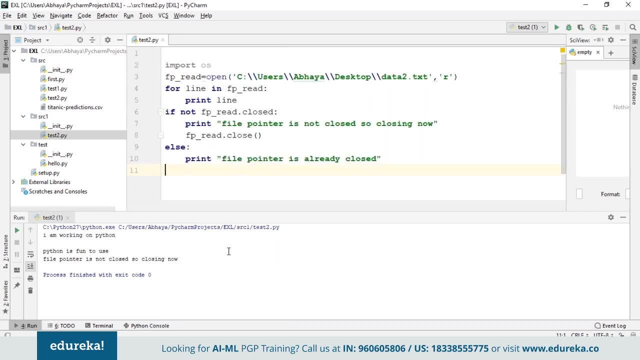 So we'll check. and also we need to manually close the file pointer. So file pointer automatically We get closed when you open any other file pointer with the same name. So if you open another file pointer creed so we open the file pointer for reading mode. 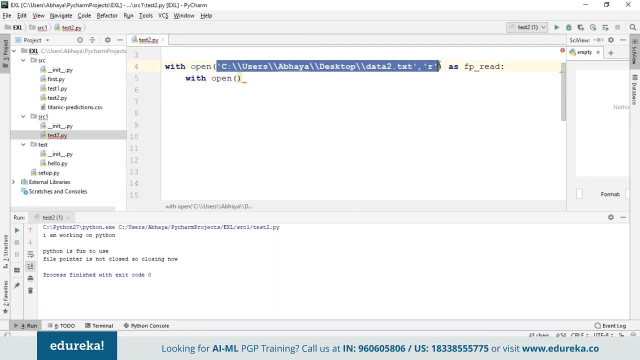 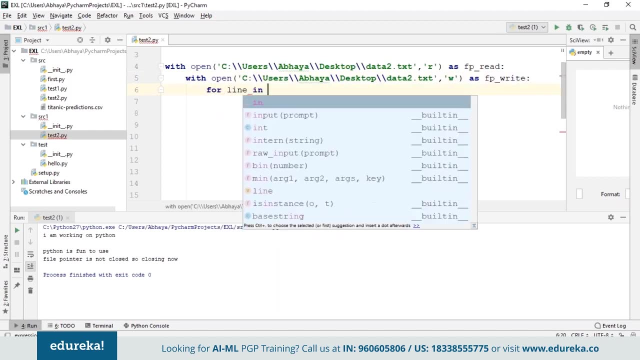 then we say with open and same path, I want to open the file pointer in writing mode and give name as FB underscore right and say for line in FB underscore read FB underscore right, dot right, and we write a line there and we close both the file pointers. all that's not required. 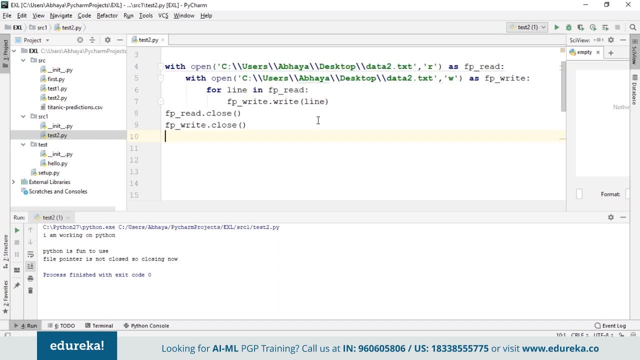 because we are using with open. So here what we are doing, We are reading the contents from the one file, writing the lines, whatever we read into the writing file pointer, That is another file. So if I'll run this program you'll see I've not changed the name. 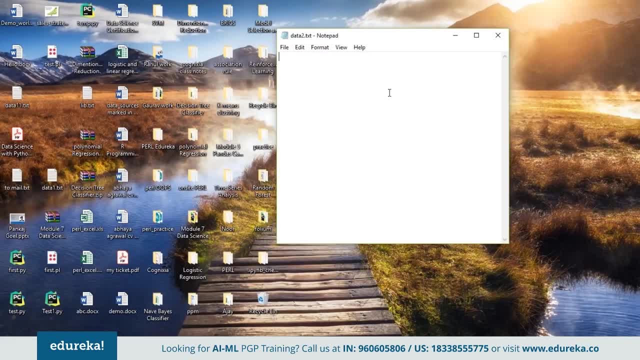 I think data to dot txt is over it in the content, So let me write down: I am working on Python. Python is fun to use and save this, not to change the file name here: data 3.. So data 3 gets created. 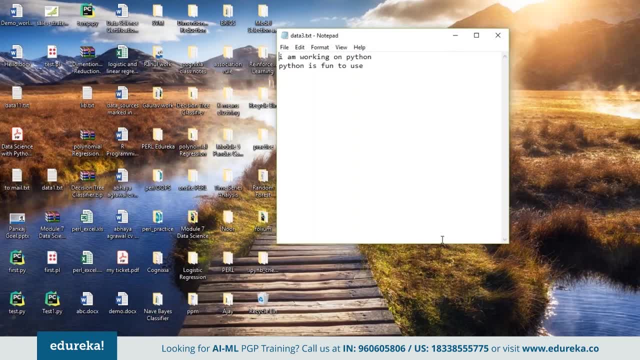 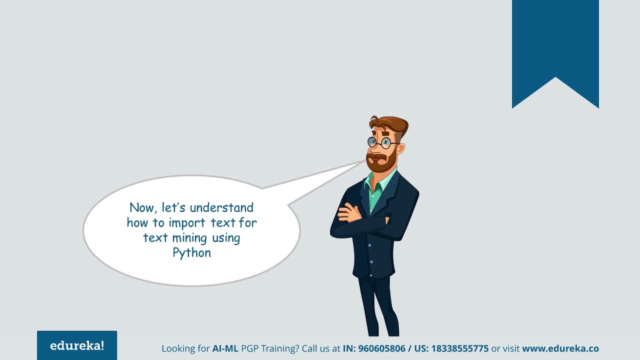 So here we have a data 3 there, with us having the same contents as data 2.. So these are some of the basic operating systems functionality We can achieve and same has been discussed here. So you can use OS module in Python to read external files. 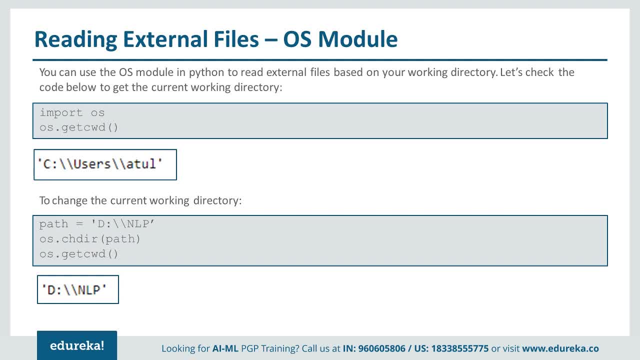 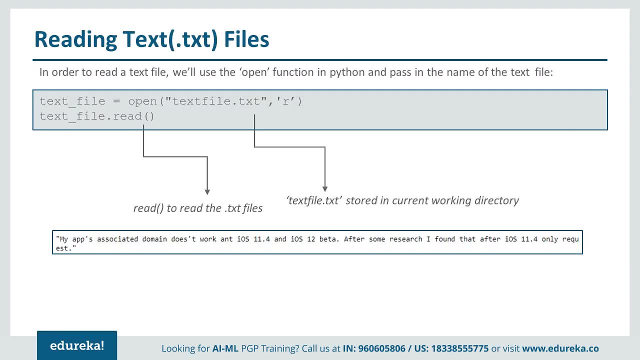 based on your current directory or working directory. Let's check the code below. So we import OS, which get the current working directory. to change the current working directory to D and LP, get the current working directory again. then you can open a file for the read mode. 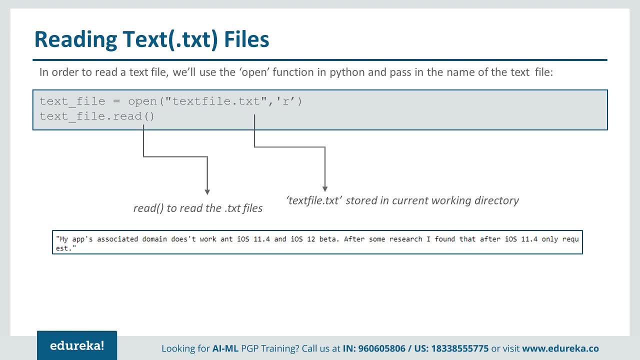 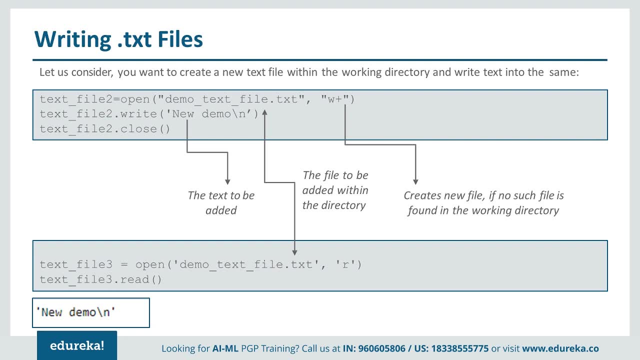 in order to read a text file. We will open the function and Python and pass the same in the text file and read the contents of the same. Then we open function in the right plus mode. Maybe right plus mode means you can create a new file reading. 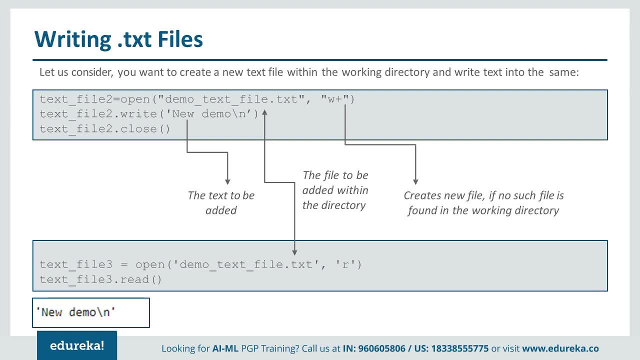 and writing both W plus means reading and writing and we write the contents, new demo and close the file. So it is just writing a text into the file and then we may open the file again and read mode and read the file It will set new demo, slash and so everything, whatever you have written. 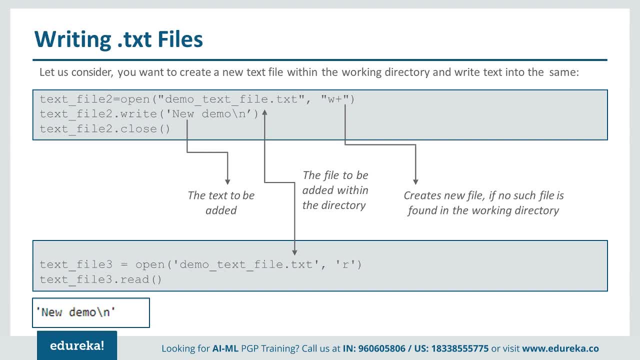 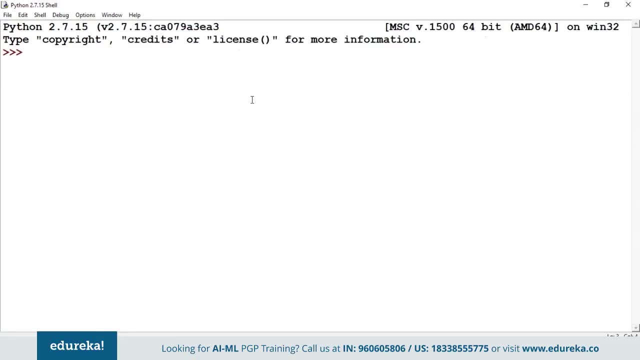 is going to be retrieved as it is Today. we are going to work on some external file, We are going to read some external file. We are going to write down something over there. So there's a very important library in python called OS library. 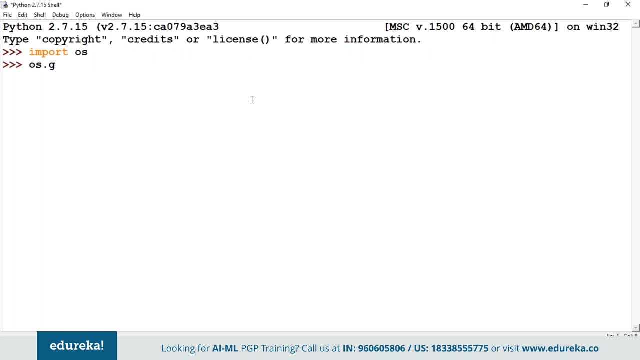 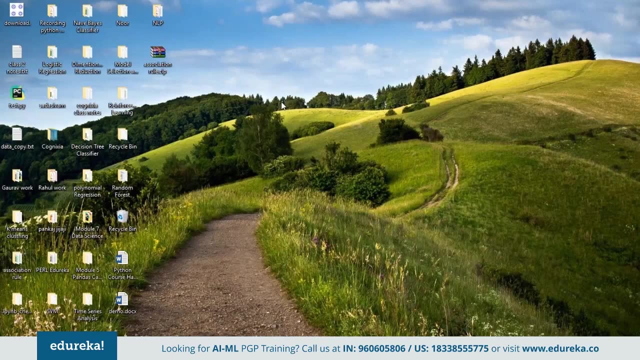 will say import OS and then say OS dot, get current working directory. So get current working directly. return with the current directory in which I am present. I can read the external file. Let's say, create some file here called data dot txt. I'll make a file called data dot txt. 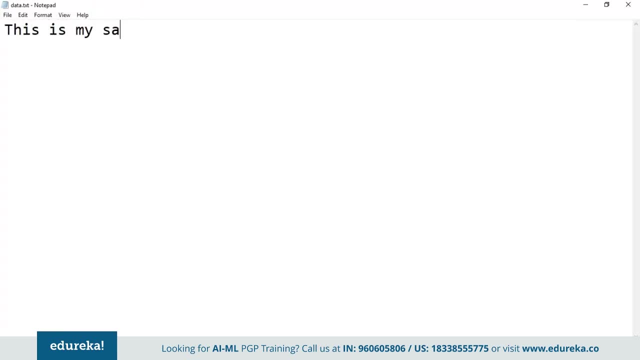 and I'll add some contents over there, Like. this is my sample file. I am learning an LP, So I'm going to read this file And first of all, I need to change the current working directory so that I can read this file. 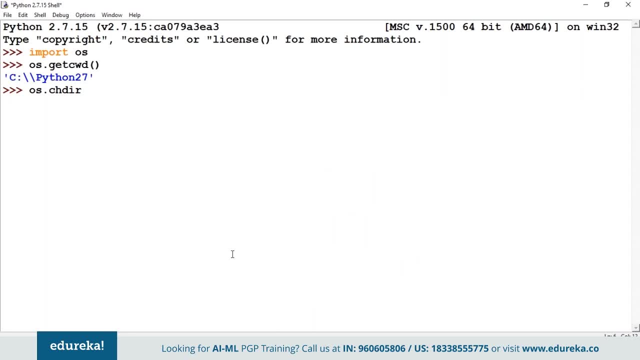 So I'm please Say OS dot ch, dir. and in Windows machine will to give double slashes to over at the special meaning of slash. now. OS dot get current working directory will show me the current working directory. Now I can open the file and say: file pointer read: 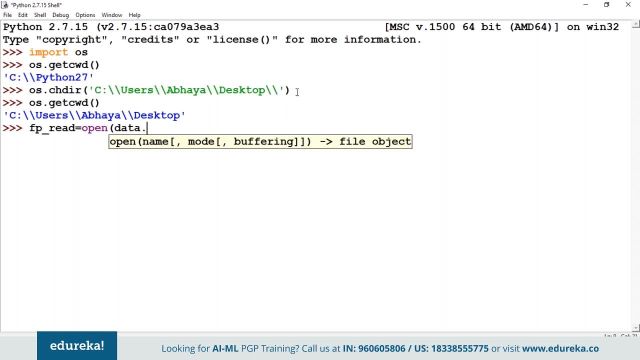 and I can say open and file name is data dot txt, and I want to open in read mode and I'll be underscore. read is going to create an object for which we can easily read the contents from this and there's a function called read. It's going to read the contents of the file. 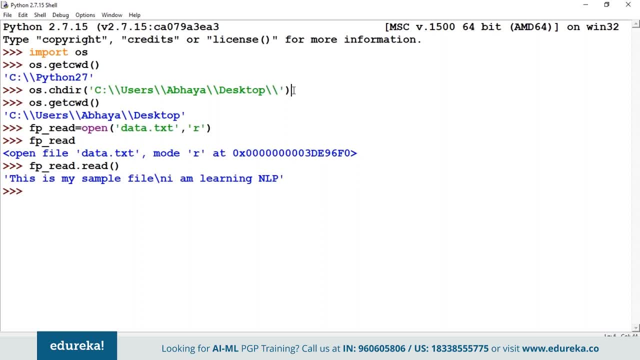 So this is sample file slash and I am learning an LP, So read function is going to read the data from the external file. Let's say I open another file. I open another file called file pointer, right, and I'll say open and I'll say data 1 dot txt. 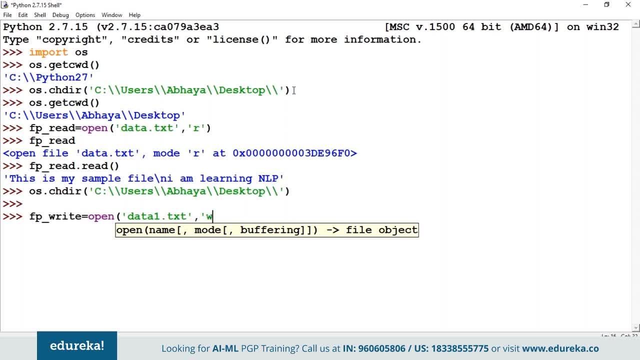 and I want to create it in the right mode: W plus, W pluses. We write and read mode both, and I can simply say FB, underscore, right, dot, right, and I want to write the contents in them as hello. So I've written the contents and I'll close the file, pointer. 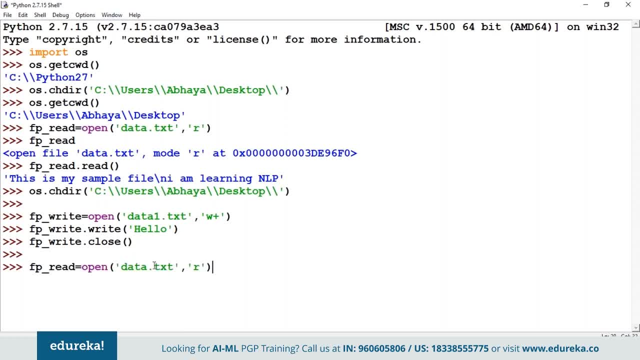 and once I close the file, point, I'll again read the file and I'll give you a data 1 dot txt and again I'll read the contents from the file. So it is saying hello, because we have put in hello there And if you see, in the desktop data 1 dot txt has been created. 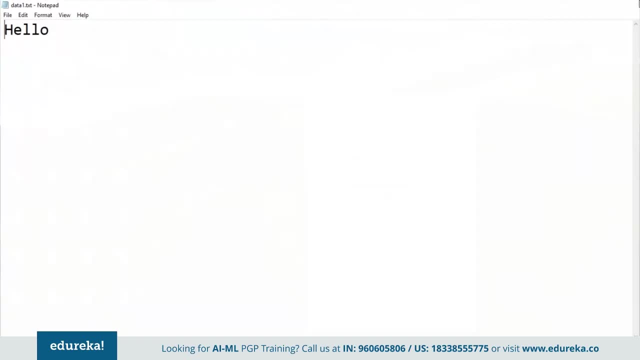 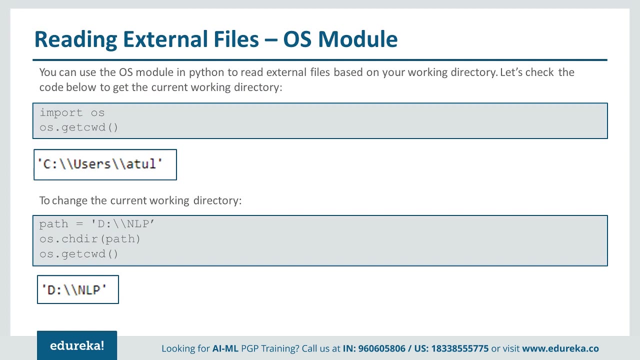 in which hello is written. Hello is written, this file, So we can read the file. We can write the file from Python. So this is the purpose of reading and writing: so you can use OS module in Python to read external files based on your working directory. 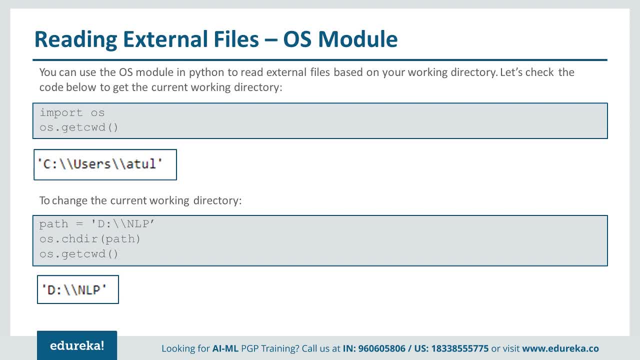 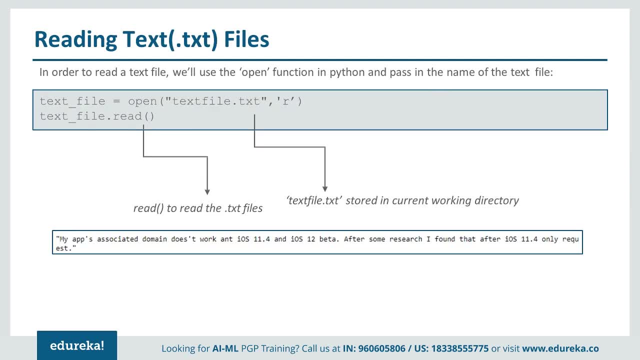 So we can import OS, get the current working directory, change The current working directory to NLP, maybe some other path, and then get the current working directory again and you'll get the latest directory which you have changed. then you open the text file in the read mode. 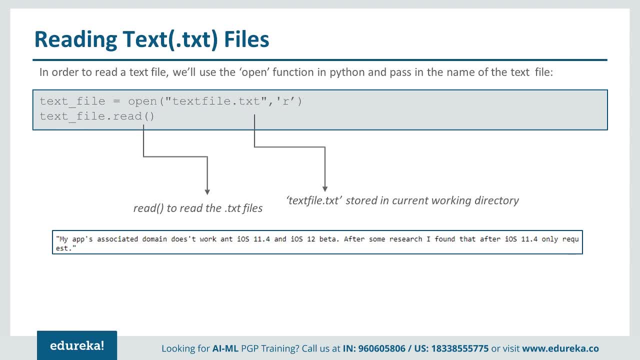 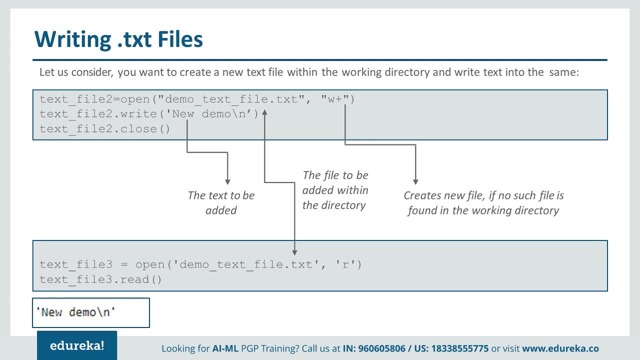 and you read it by using read function. in order to read a text file, You will have to open the function, use open function in Python and pass the name of the text file. So let us consider you want to create a new file within the working, within the same working directory. 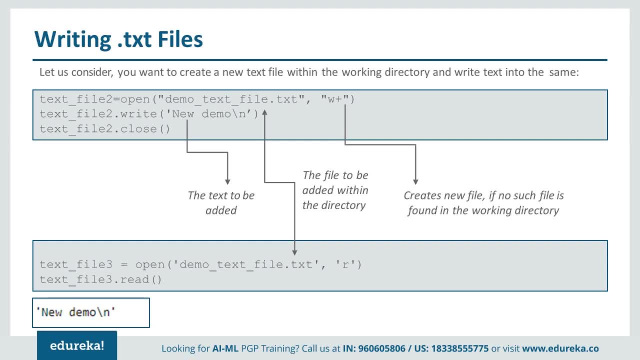 and write text into the same. So you'll say demo underscore text file, dot txt, and open it in the read and write mode and write their new demo and close the file pointer And then again you are reading the same file: demo text file, dot txt. 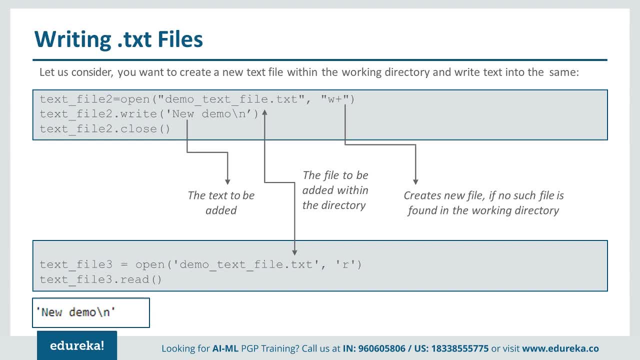 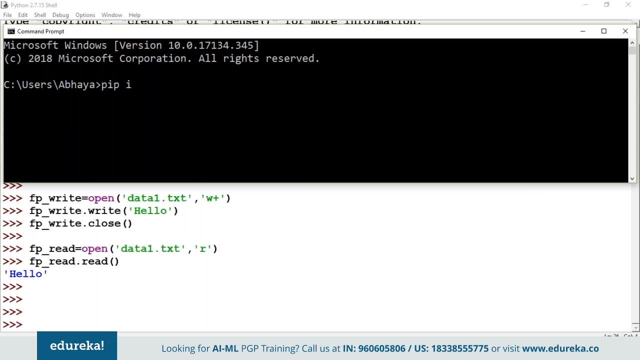 and reading the contents, You will see the same contents- new demo- written over there. So let's move forward. Let's talk about this is a library called docx. You'll see two docx libraries. One is pip install docx. You don't have to install this docx. 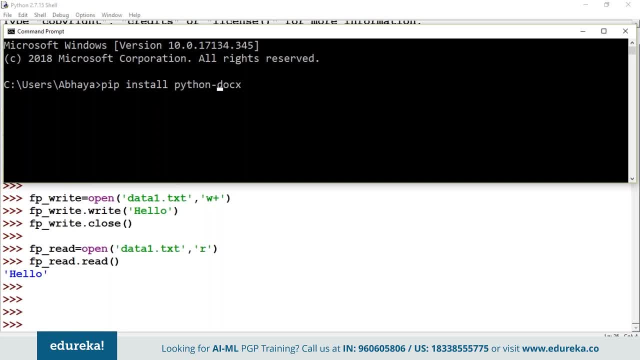 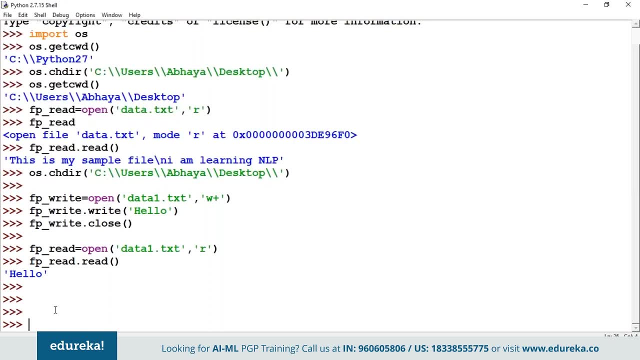 You have to install python hyphen docx. So this is a library which is generally used for reading some external document files. document files are like docx files in MS Office. when we use MS Word we have a certain file called with extension Docx. so you can read this kind of a file called docx files. 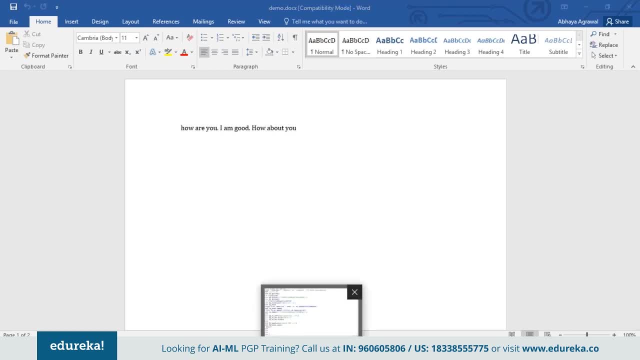 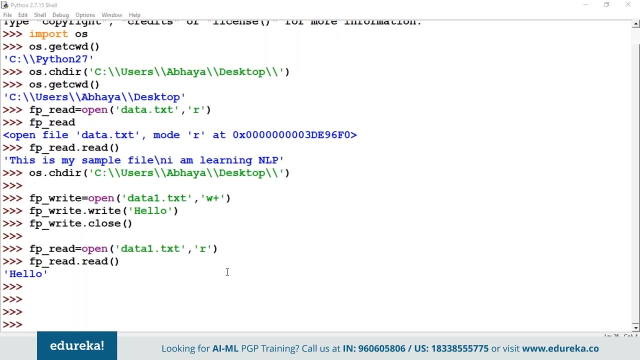 So docx is basically library which is used for reading the external MS Word documents and generally this is quite handy when we want to create some word documents reporting. So not many times what happens is you connect to a database from python. you get the results in a form of a pandas data frame. 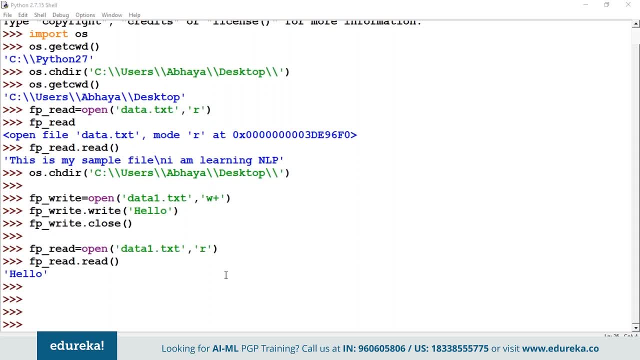 So one way is you dump it in the form of a CSV file by using write CSV. another can be create a customized report or customize kind of a word file which is as per your understanding, As per your requirements. you can create some kind of a MS Word file dynamically. 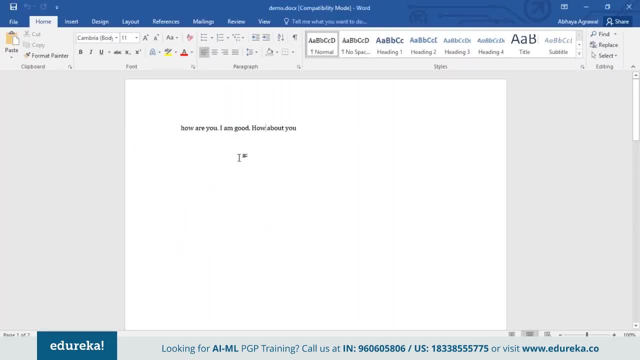 So when we create a MS Word file, what we do? we open MS Office, MS Word, and then we start typing over there Whatever the text we want to write. text again can have multiple headings, It can have multiple subheadings, It can have a paragraph. 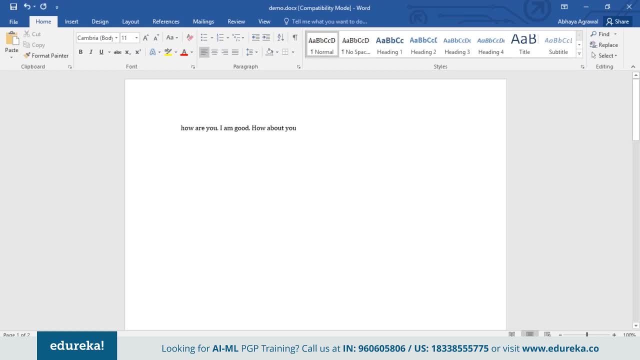 So when you press enter in MS Word, it starts a new paragraph. Otherwise it keeps on typing in the same paragraph. in MS Word, When you start typing- obviously like when the page is over the line- comes on the next line And you start typing on the next time. it is in continuation. 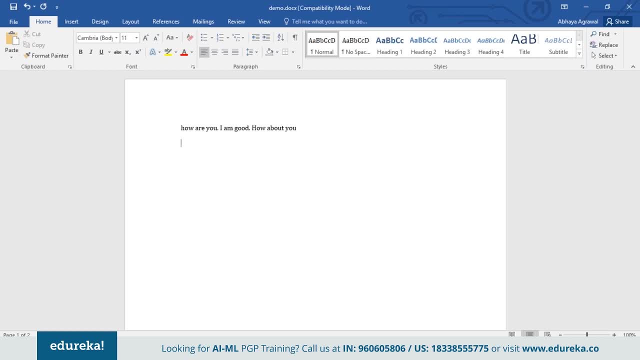 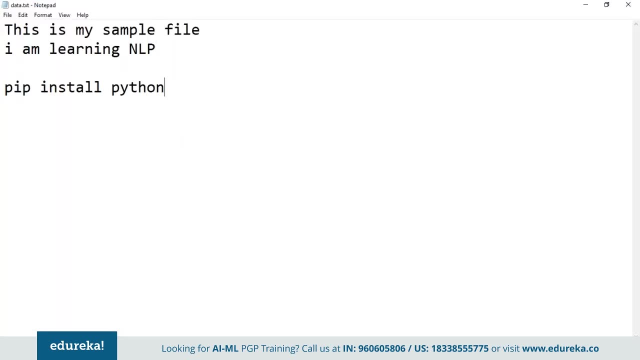 But when you press enter, hit enter key, it starts a new paragraph. So we can create our own document files using this in Doc X and you need to install it like using pip: install python-docx. don't directly install docx, because we'll get a different library in that case: python-docx. 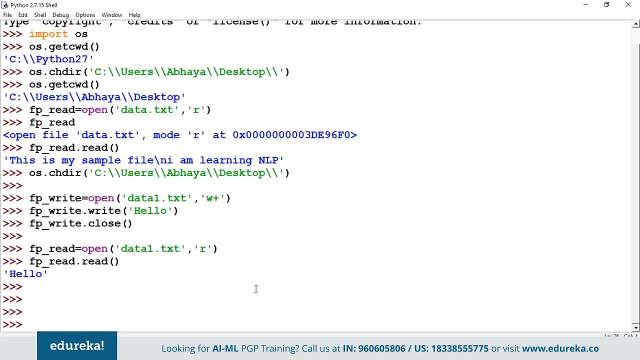 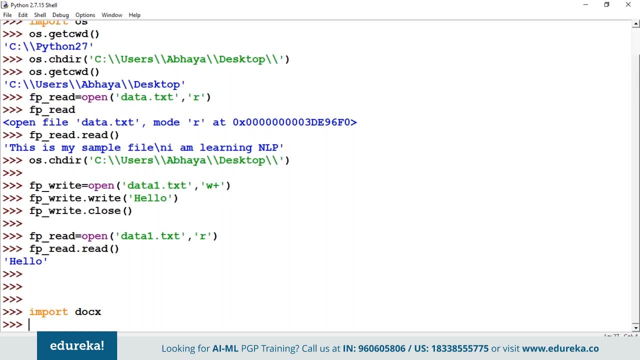 is the right library which you need to install, and once you install it you can import this, import docx. So this lab is pretty handy in creating some word documents. I'll show you one fancy program as well. So we'll say: doc equal to docx, dot. 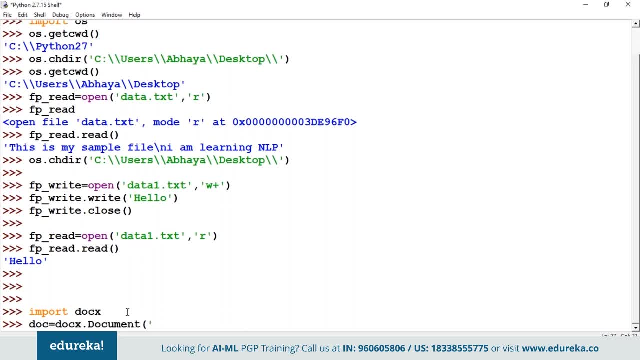 There's a function called document which is going to tell you open the particular document for you. So let's say I have a document called demo dot docx on my desktop, So I can simply say demo dot docx. So I'll say length of dog dot paragraph. 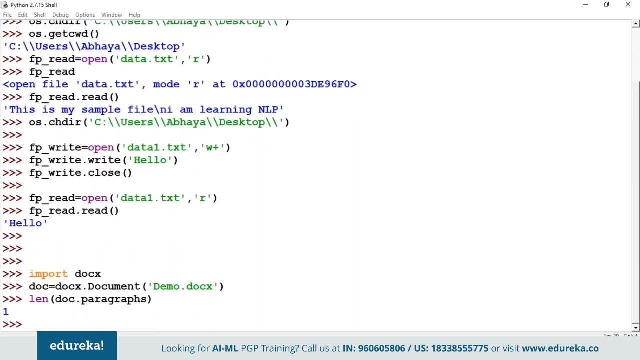 So we have a one paragraph. of course, because we have not hit in the enter key here. It's a single line. We have a one paragraph only in this, so it is going to tell you how many paragraphs are there in the particular document file. 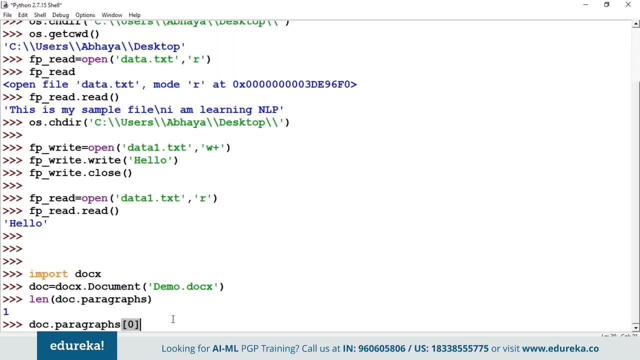 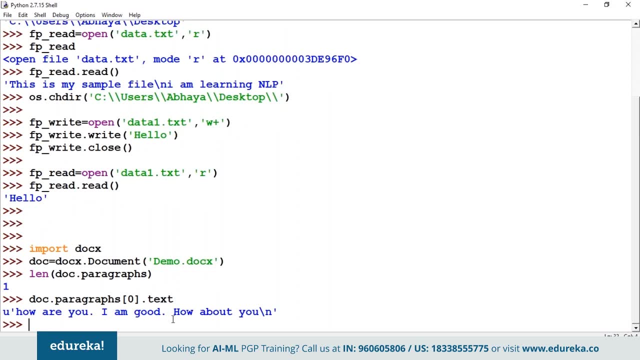 So we can simply say it: dot paragraphs: 0 paragraph, dot text. It is going to give me the complete details. So 0 paragraph, first paragraph, second paragraph. So when you hit enter there can be a number of paragraphs. So we can read a particular paragraph. on the word file by 0, 1, 2, 3. 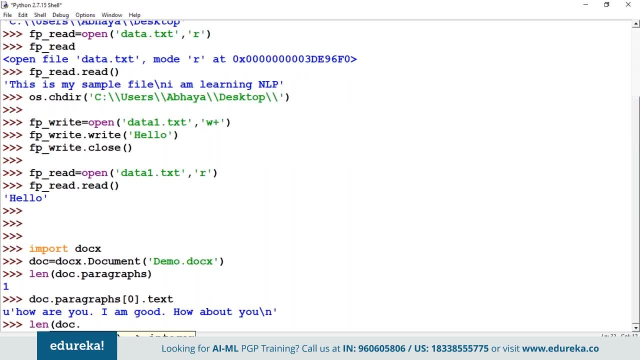 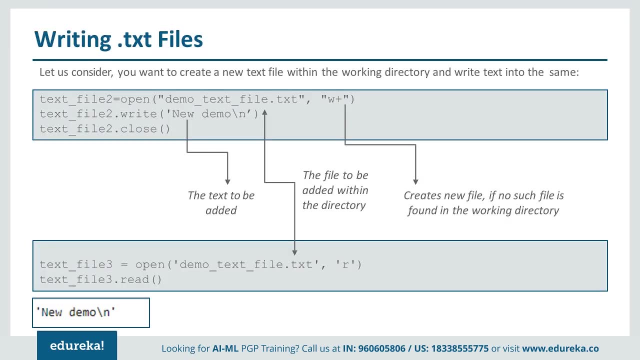 and so on. similarly we can use length function: doc. dot paragraphs 0, dot runs, their total 8.. So if you see here, total 8 runs is going to tell you how many words are there in the particular Talk file. So let me give you some brief idea. first, 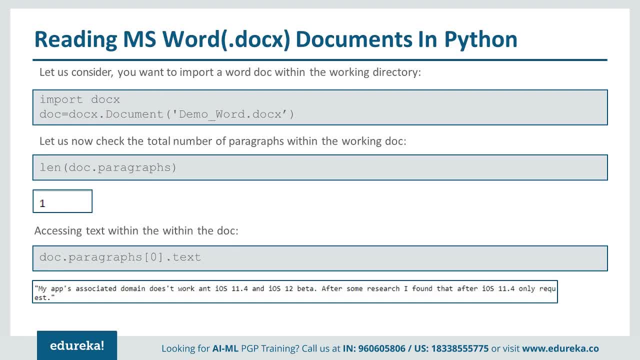 Let us consider So you want to import a word doc within your directory. you import doc X and you read the file demo world or doc X. So let us check the total number of paragraphs. So length of dog dot paragraphs will tell you how many total paragraphs are there accessing text. 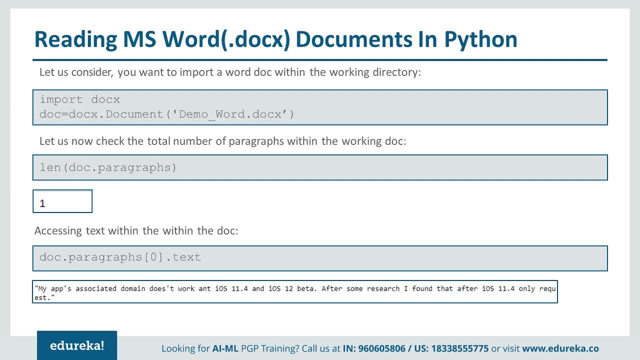 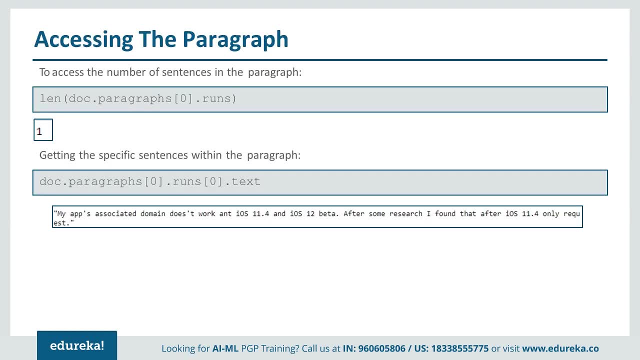 within the doc that you will see: paragraph 0, paragraph 1, paragraph 2 and text. It is going to filter out the text from the particular paragraphs to access the number of sentences in the paragraph You are going to say runs. runs is going to tell you number of sentences in the paragraph number. 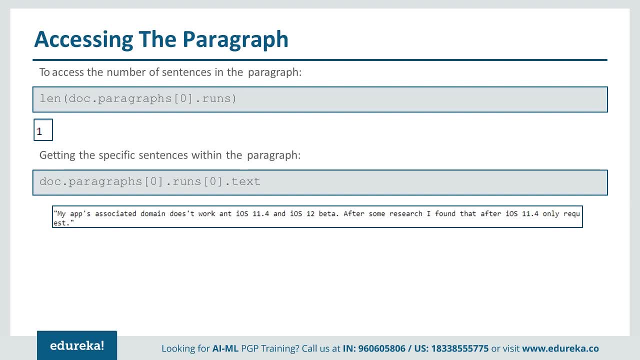 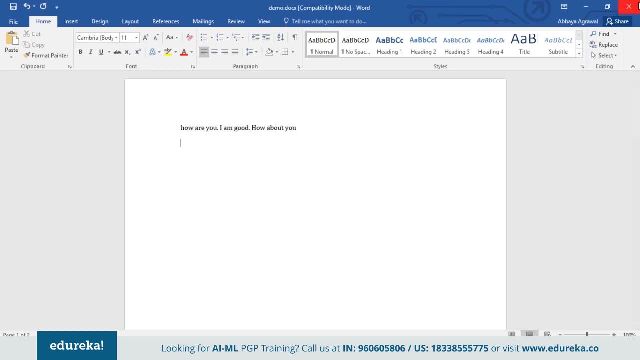 of sentences means logical sentence. So here we have one, two, three, four, five, six, seven, eight. So it is going to internally. So it looks like we have three sentences here, but here total of eight sentences get printed over here. 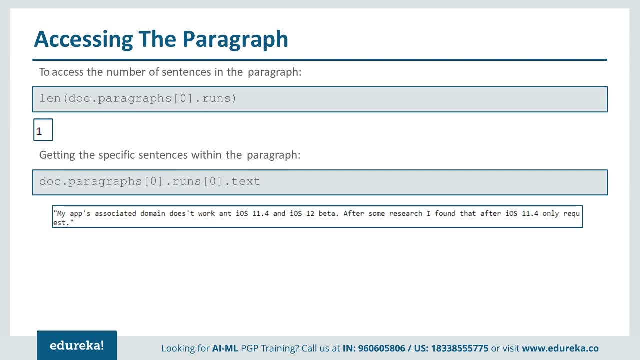 So getting a specific sentence from the paragraph, We can say paragraph 0 from the 0th paragraph, from the first sentence, 0th sentence. filter the text. similarly from the second sentence: filter the text. So within paragraphs we have certain sentences within sentences. 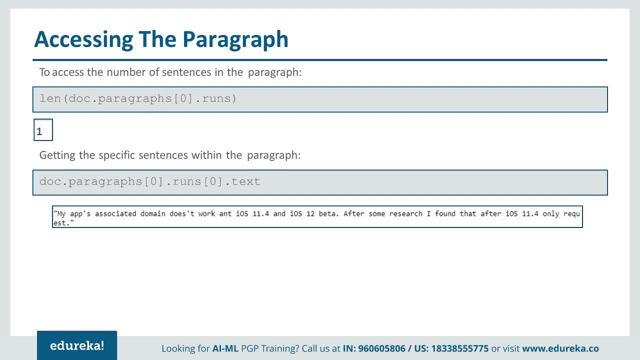 We have words. So if you want to take a complete paragraph and want to filter out the first sentence, you'll say run 0.. We want to filter out the second sentence, You'll say runs 1, and so on. So it will pick up the sentences as per the definition given. 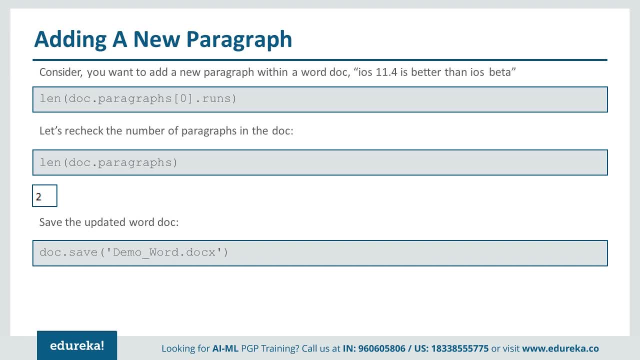 there in this paragraph library. suppose you want to add a new paragraph within word doc. So it will simply say it is not saying about adding. I'll show you the code for adding. it is simply taking the length of the particular sentences total. How many sentences are there in the first paragraph? 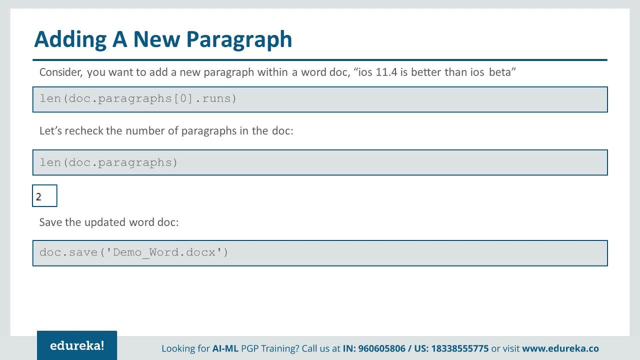 because it runs, tells you sentences, So run, 0 means 0th sentence, 1 means first sentence, 2 means second sentence and so on. and length is going to tell you how many total sentences Are there in the particular paragraph. length of doctor paragraphs will tell you total paragraphs. 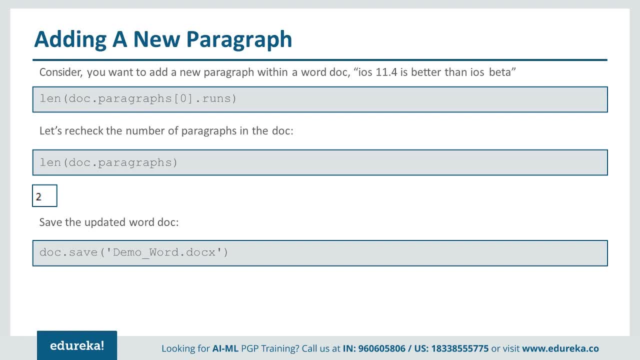 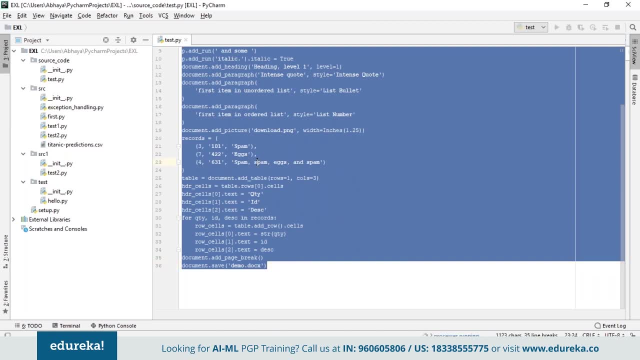 in the word document. We can save the word doc as well. doc Save will save the word document. So there are multiple functions in build in this. Let me open pie charm and show you the code first. This is a very good example. 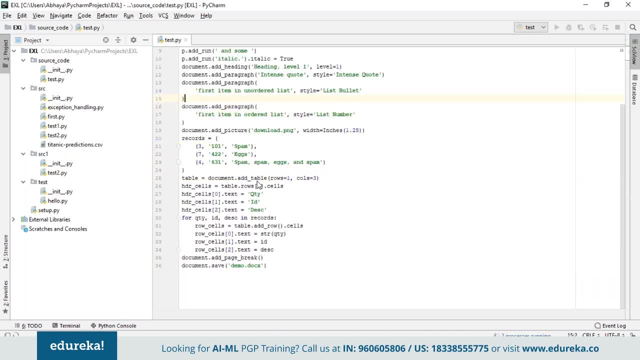 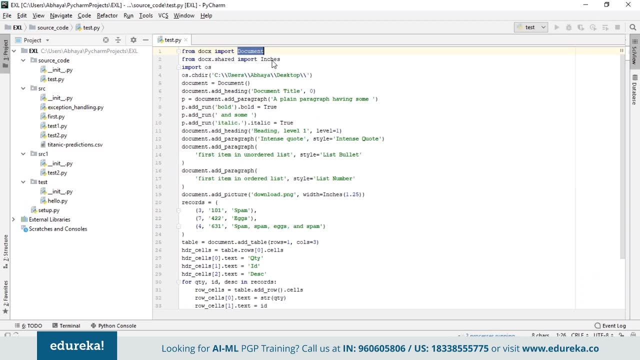 It takes care of everything in this. I'll explain you, land by land, what it is doing. So from Doc X, we import document, document. We import just to create document or read the document. Similarly, docorg, She had imported inches. I'll tell you what is the reason why we imported inches. 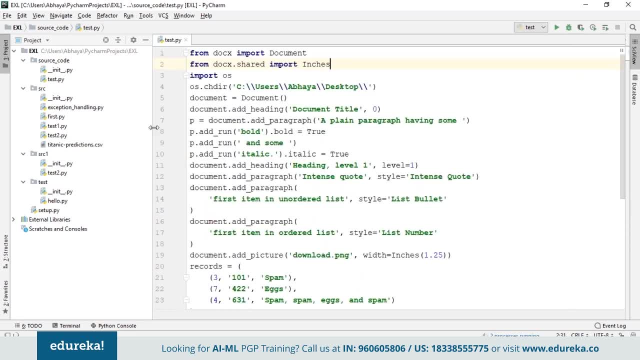 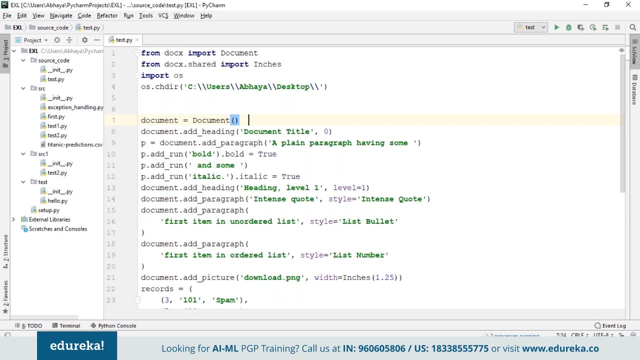 Let me increase the font size. So here what we are doing. We are importing OS library and changing the directory of desktop. Then we create a document object. So document equal to document is going to create what document object on which we are going to work? 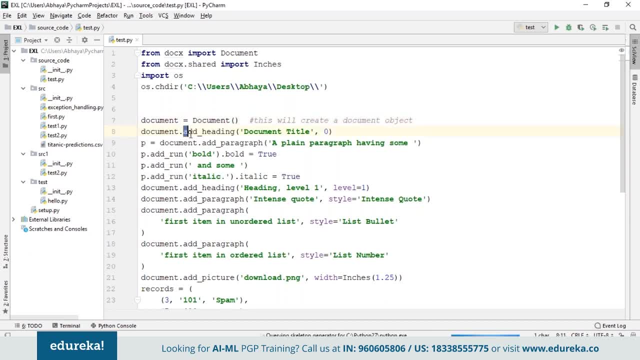 So this will create a document object and add heading. So whenever you prefix something, add, it means you are writing the things over there. So add heading is going to had heading to this document title and from the 0th row It is going to add the particular title in the document. 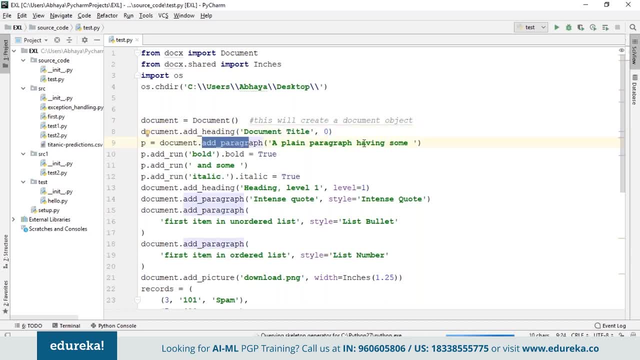 Similarly, add paragraph is going to write a paragraph, a plain paragraph, having some bold and some italic. So P dot, add run. add run is going to run the particular command, like, for example, when we are working on MS word. you might have observed, we click on certain buttons. 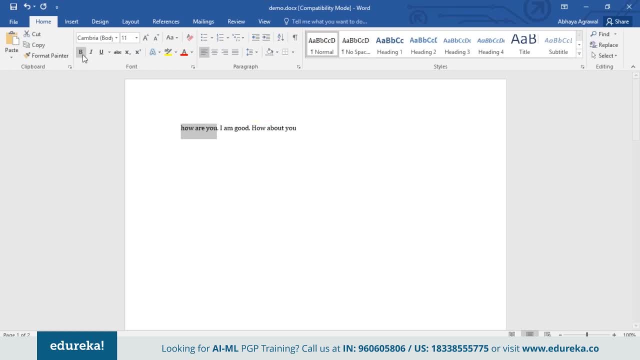 We say: what suppose I highlight something, and I highlight it after writing a press on bold. So what we are doing, we are executing some command. So whenever you want to execute some command, we call it as run over here in this terminology We call it as run. you say: add, run, bold. 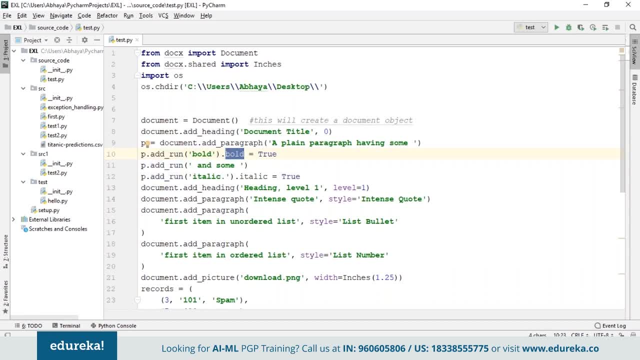 So it is going to add the text bold and bold it out. Dot bold is going to bold it out. Similarly, add run some text. This is simple text, I have not done anything. Similarly, it is going to write italic and italic it. 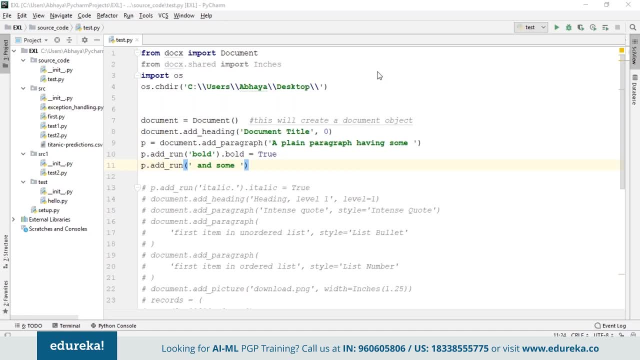 So let me run up to this level first, So we can create a document with a document object and then we can add: whenever you see add function, which is prefixing with add, It simply says we are adding something, So we want to add a heading to it called document title. 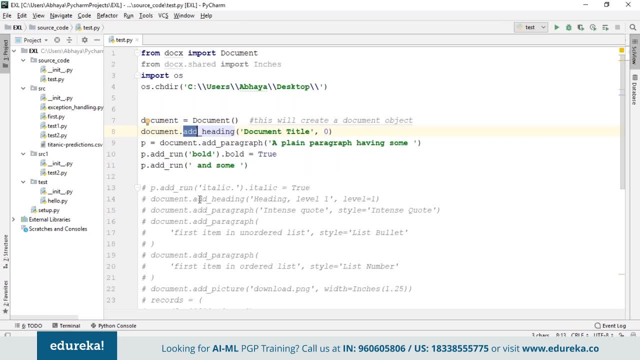 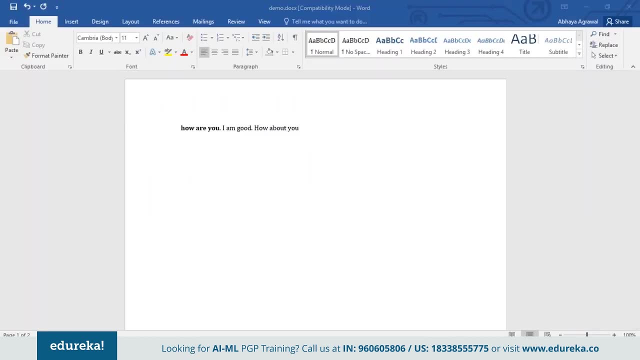 and then we add a paragraph, a plain paragraph, having some so like an MS word. We want to do something bold. We click on the bold button right. Suppose you are, highlight something and click on the bold button similarly here when we want to make something bold. 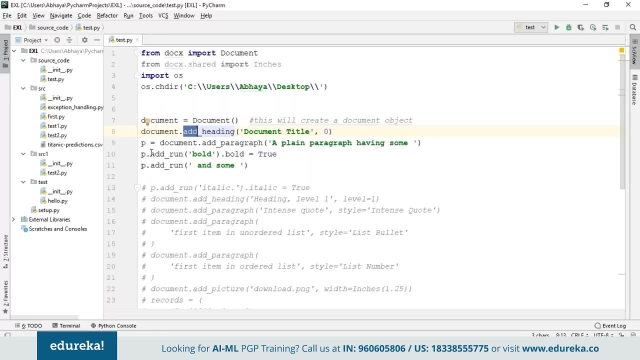 or we want to make something italic. We use the add run command, Add run function. So add run function is going to do some kind of action. We say I want to keep it on some bold. Similarly, I can add run and says I want to put something. 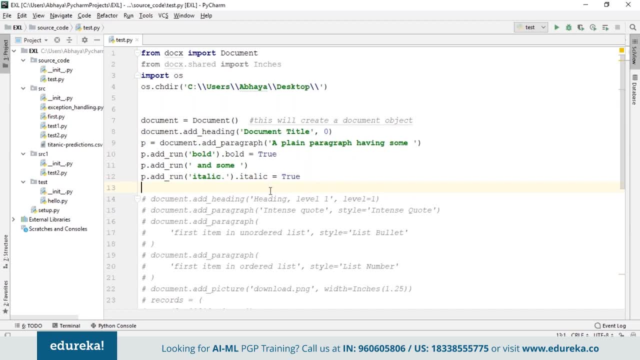 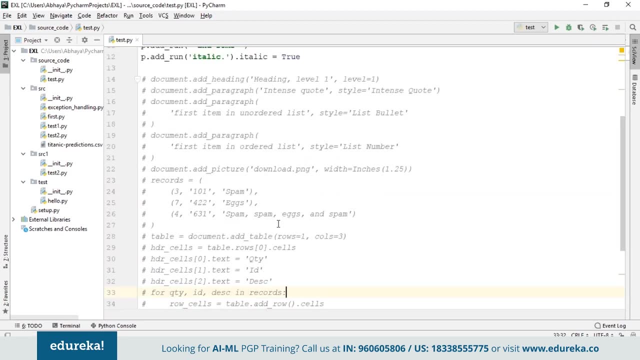 in italic. with this italic, What will you put in italic? So I'll save this document. I have commented rest of the things I have saved. the document called demo dot X- demo. Let me put demo one here. So it is going to save the document with demo one. 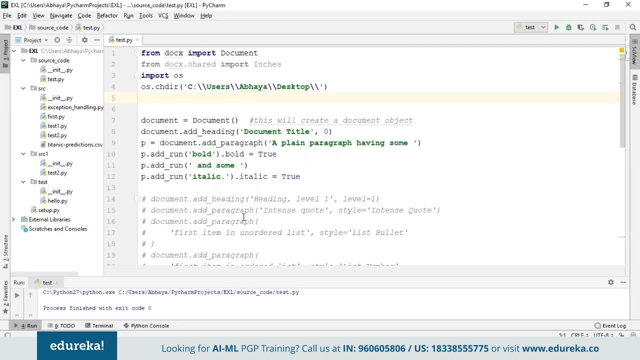 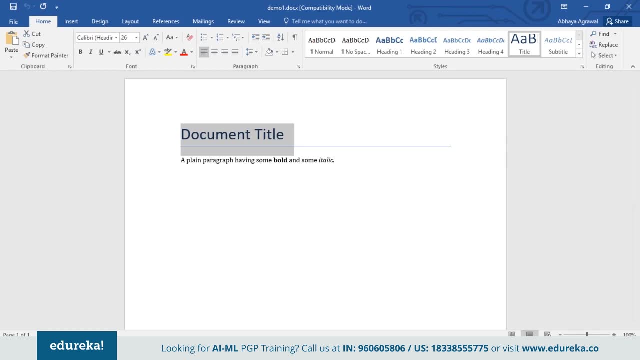 So let me run this. So it is going to create a demo one on the desktop And let's open this in MS word. You can see document title, what we have written, the code We want to give their heading. heading is coming as what document title. 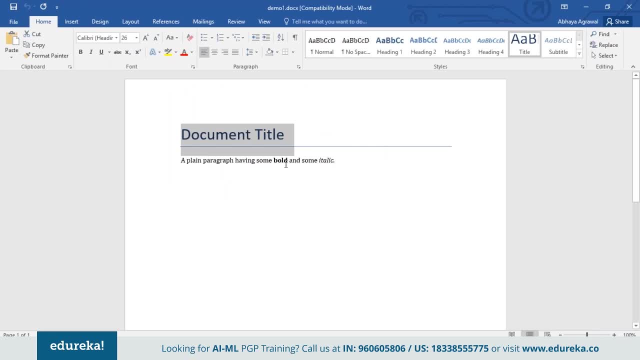 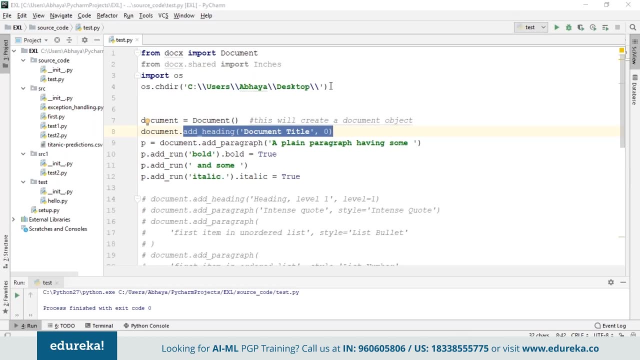 and it is coming a plain paragraph having some bold and some italic, and we gave this kind of a coding only. So what we have given, we have given: add run bold and add run some italic. So we have given like this. now we will see some more functionality in this suppose. 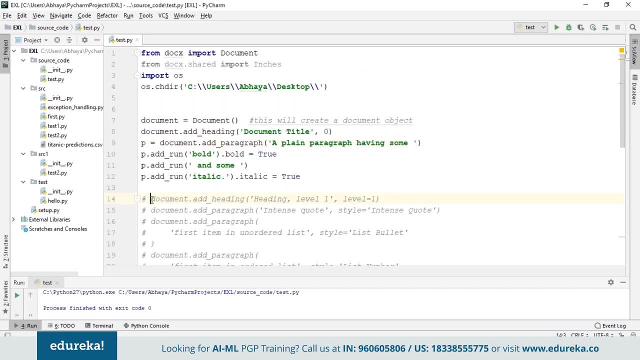 You want to add heading, You will simply say: add heading, You're going to create a heading as well, heading level 1.. So in headings we have a different level: level 1, level 2, level 3, level 4 and so on. 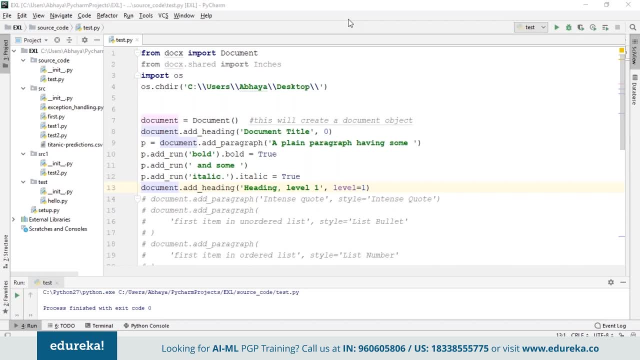 So in headings we can go from one heading to another. similarly, We want to add some paragraph and say add paragraph, style equal to intense code. So I'll show you what this style is. Similarly, you can say add paragraph and you can add some paragraph here as well. 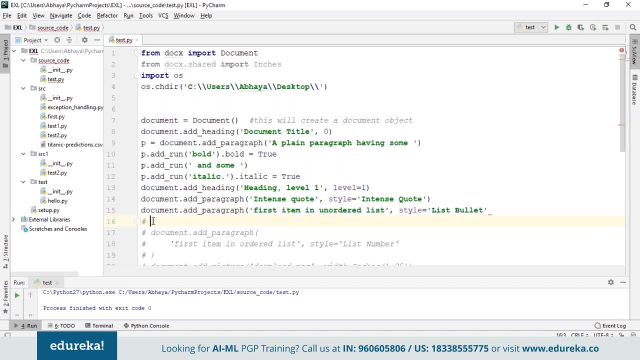 And when you are adding the paragraph you can give a bullet style is bullet style, and similarly you can give a paragraph in the form of a list number. So let me run this again and show it to you. We see here, So we got a heading. one intense code means it is going. 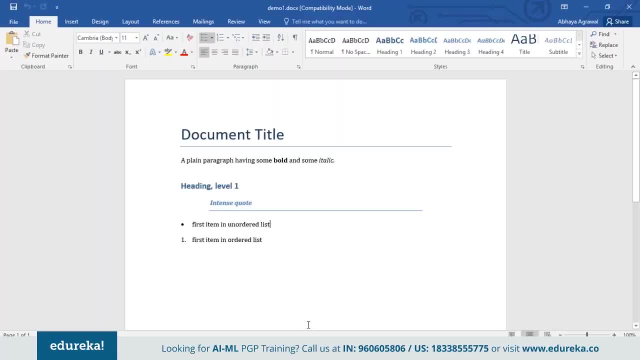 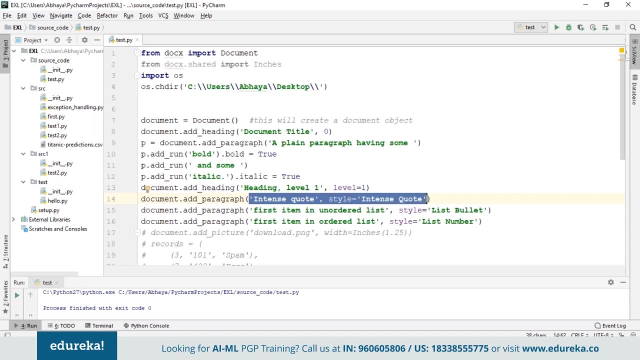 to put another heading. So that's another type of heading called intense Code and we have given here heading level 1, intense Code. style is intense Code. intense code is it is going to be underlined, It is going to be heading and then paragraph. first item in the ordered list. 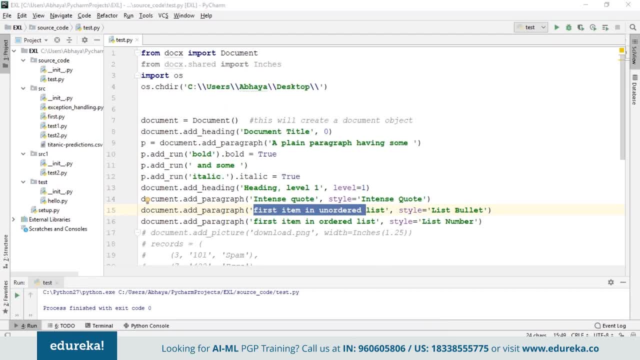 for list bullet. So we get what bullet. similarly, numbers: first item in the ordered list, We get the numbers. style is this number. So list bullet is going to print a bullet. list number is going to give a number. similarly, if you want to add some picture, 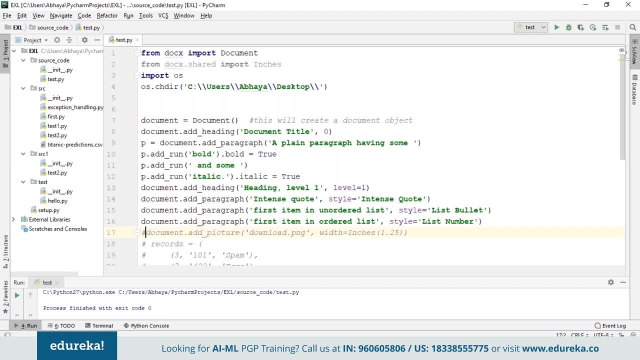 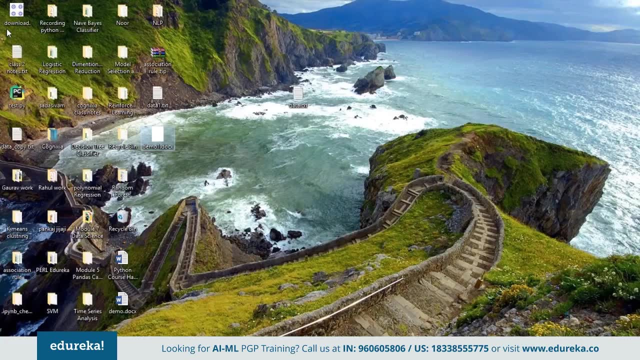 so you can say download document, dot. add picture, download PNG. So I have a picture on my desktop called download dot, PNG. So I already have some picture there with me. It can be any picture, You can have any image. So I want to incorporate this image into my document. 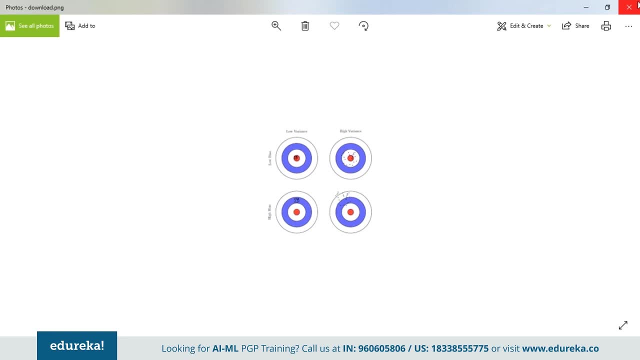 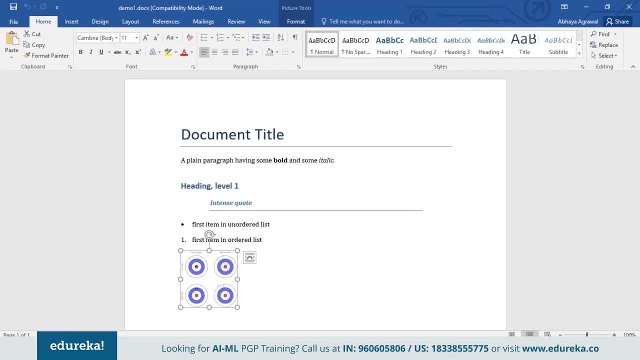 So I'll do what I simply have to say: add picture, download PNG and in with how much inches I want to put this image. Similarly, we can have more functionality. We can create a table as well. Suppose I say records are in a format of this. 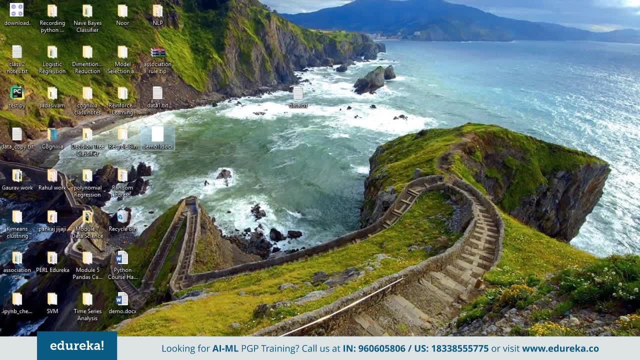 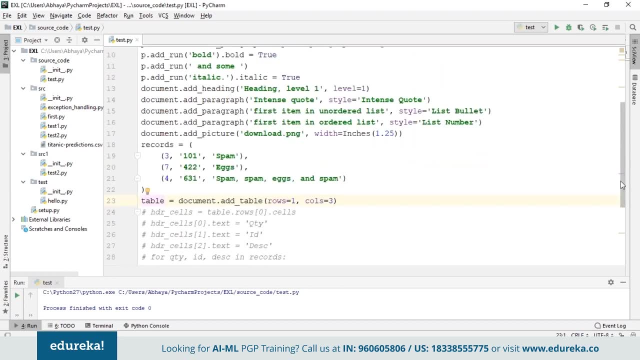 and I want to create a table. So I'll say: table equal to document, dot, add table. So all the functions are very self-explanatory: add paragraph, add table, add heading, add run. Similarly, we defied the number of cells. What is the cell 0? quantity of cell 1. cell 1 is column heading. 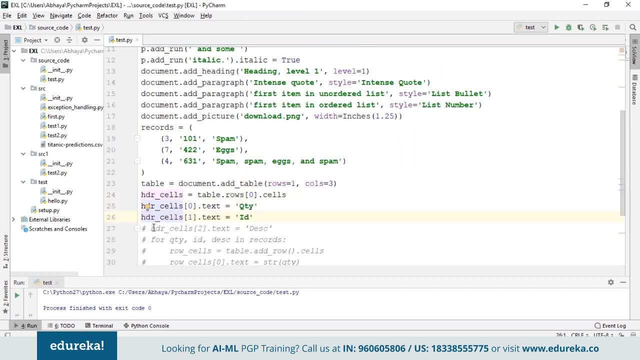 So cell 0, heading will be quantity, cell 1, text will be ID, cell 2 will be description and we run this in a for loop for all the records. records is: what's tuple of a tuple? we run it in a form of a for loop. 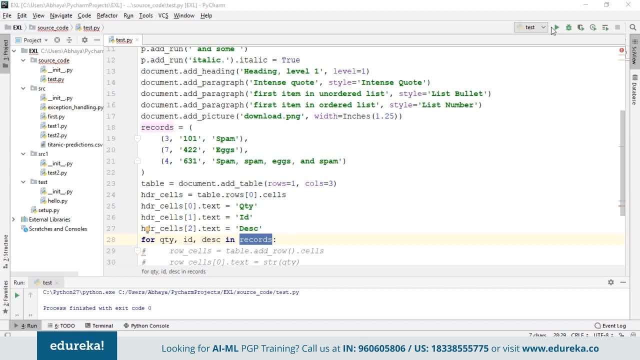 And once you run it in a for loop, we are going to put one by one all of these values grow cells equal to table dot. add row in dot cells. So every time it is running is adding new row, one by one and all the cells. 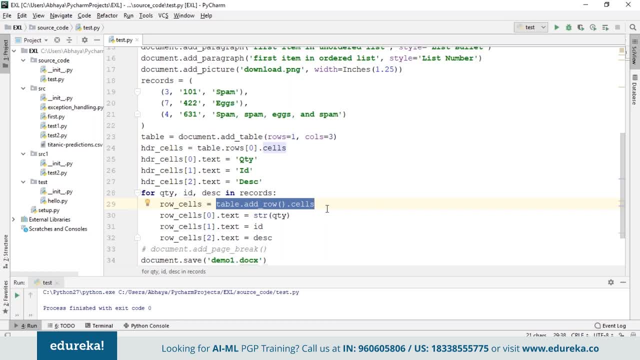 Cells means columns. that is going to add one by one all the cells and adding the text, their quantity of the string, quantity, ID and description. and we can have a page break as well in the document. page Back means it will go to the next page. 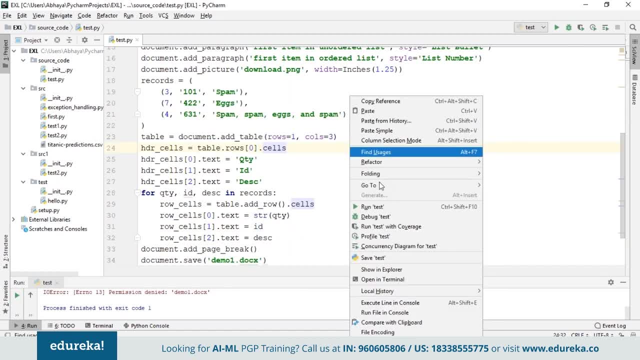 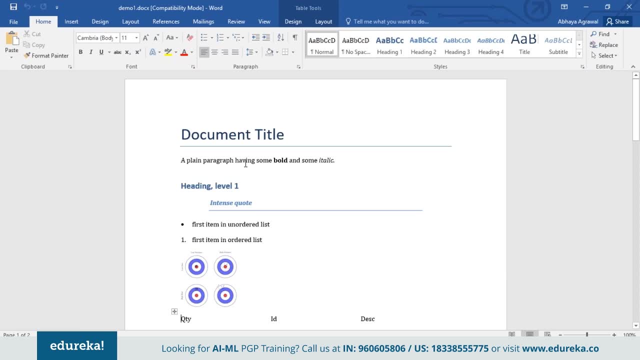 So once I run this, it's denied. We have opened the file. You can see, so I did a document title: We have added a bold and italic. We have added headings. intense code: We have added a bullet and a number. We have added a table. 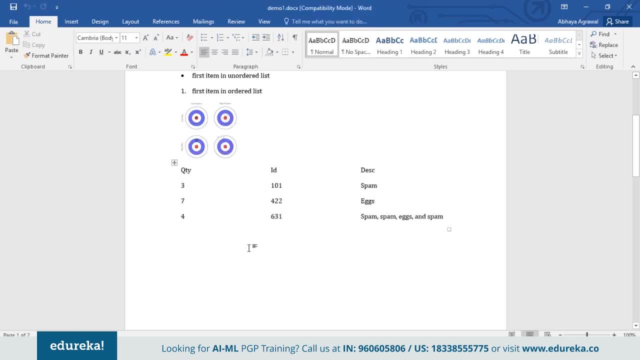 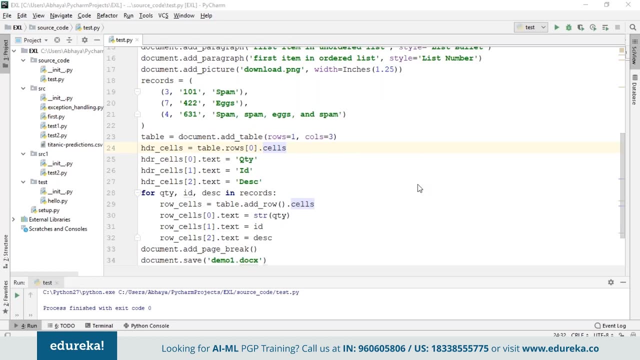 So this is going to be a table having quantity, ID and description. you can start anything over here, So this is generally like how we create reports basically. So generally we use docx library to create beautiful reports for us So we can do formatting. 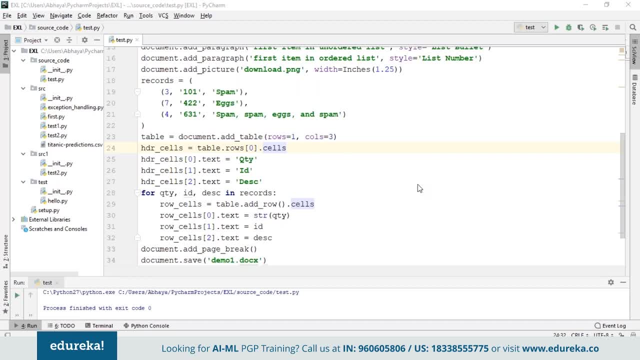 We can put the data in a form of a tuple of a tuple or tuple having a list, in a form of a table in Word document. So very helpful library for generating MS Word document to for you. now coming back to the presentation. So we have seen the paragraphs. runs means running the command. 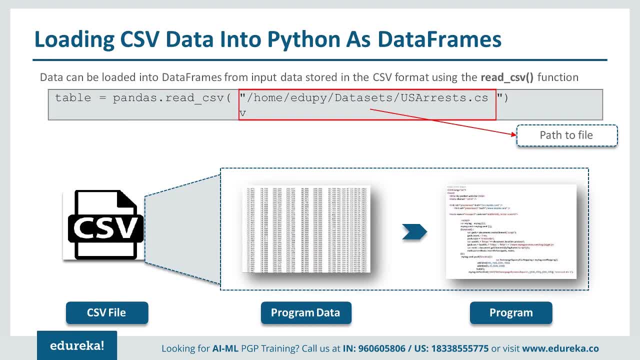 We can save the word document as well. Now We have already known pandas library. Panda is a very common library. We read the CSV file, so we can read the CSV. We can write the CSV, so we can read a CSV. We can read the particular table as well, particular column. 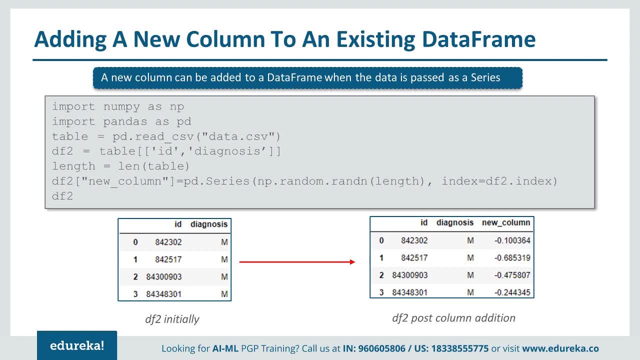 Then we get: give the length of a table, We can add a new column, taking the length and some random values, and we can create a data frame out of it. So we have seen all this: how to read a CSV file, how to take a column, how to add a new column. 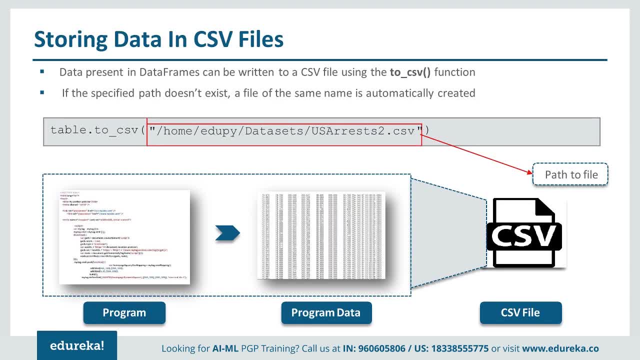 to us already existing pandas data frame. and to CSV function is going to write the contents into a CSV file. to CSV function is writing the contents to a CSV file. now let's talk about analytical every, which is quite handy. So, working on NLTK Cobra, most popular library in python for NLP- 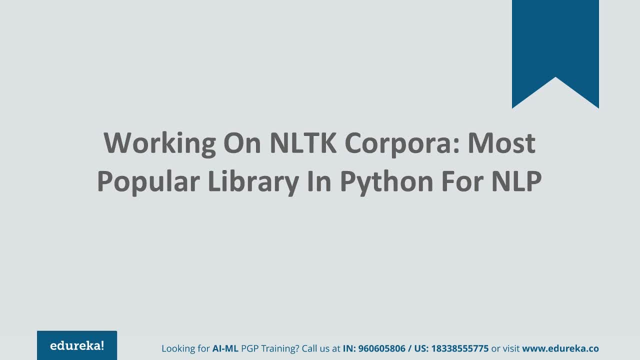 So in NLTK it's a bunch of libraries. So NLTK is not a single library. It is having a bunch of libraries for different purposes and one of the most popular library in NLTK is Cobra. So in NLTK there is a group of libraries. 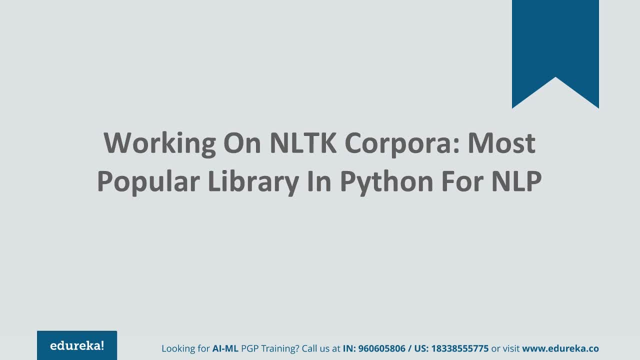 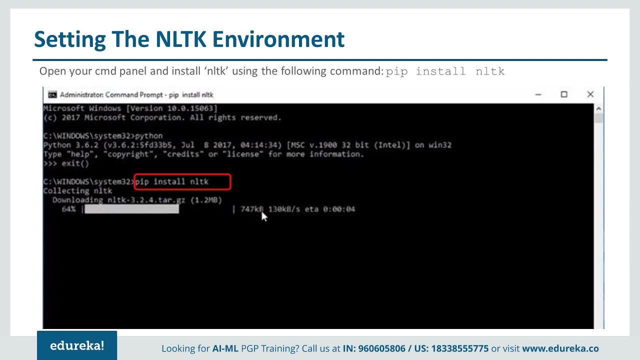 So what is the first step? So first step would be download NLTK. So first of all on your DOS prompt you can search, just write pip install NLTK and if you are using a Jupiter notebook you can simply say exclamation: pip install in the Jupiter notebook. 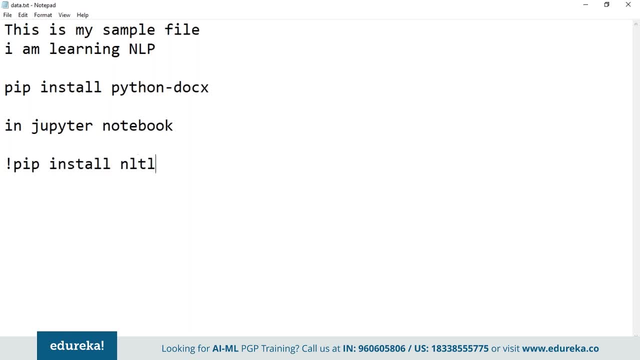 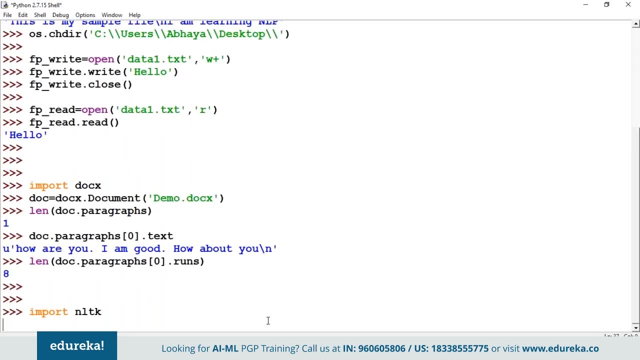 You have to write exclamation pip, install NLTK and install NLTK for you. So once you install NLTK you need to import NLTK in your program. So it's a big library. It is going to download a lot of things for you. 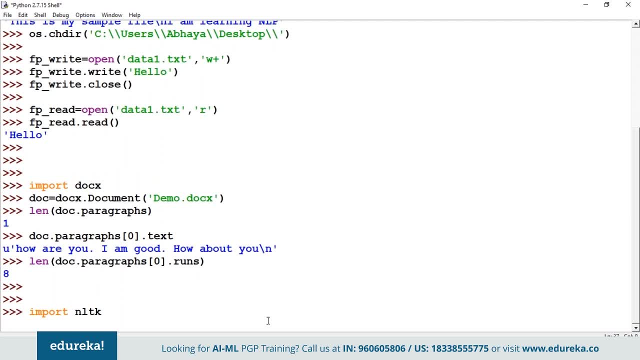 Once you install NLTK and it is a base library which comes to you, all the sub libraries in NLTK- or you can see all the libraries which are part of NLTK- do not comes automatically. You need to download them. So once you install NLTK, you need to download. 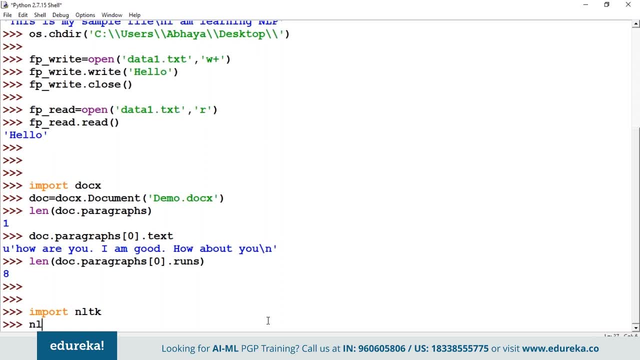 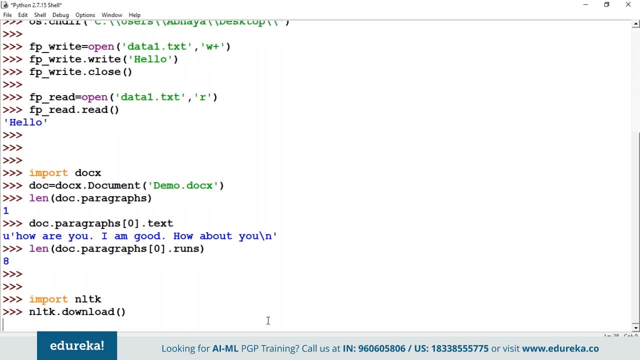 all the libraries present in NLTK. So you, how do you do that? We'll simply say NLTK dot download. It is going to download all the libraries for you, So it is going to open a new window for you in which all the library names would be listed. 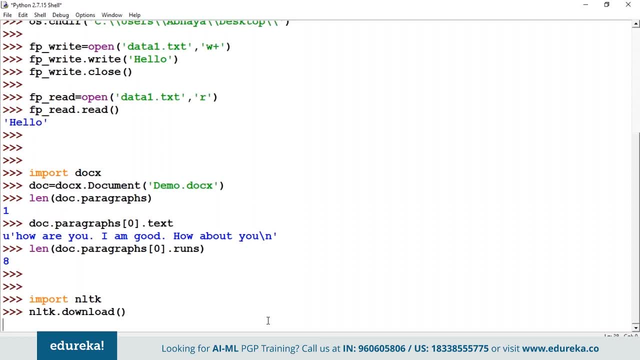 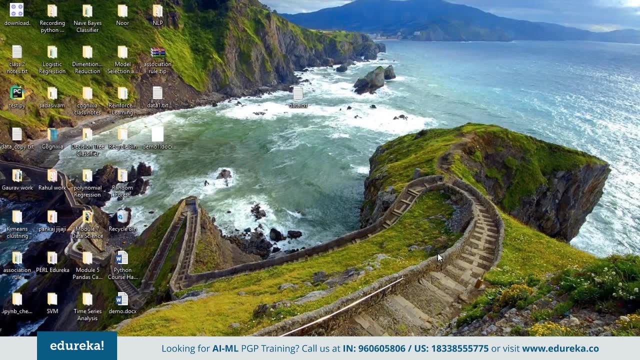 and you can simply click on install button there and download. So it is going to open a new window for us. See here, this new window has been opened and you can see collections- copra library. So within copra there are so many identifiers. similarly, models. 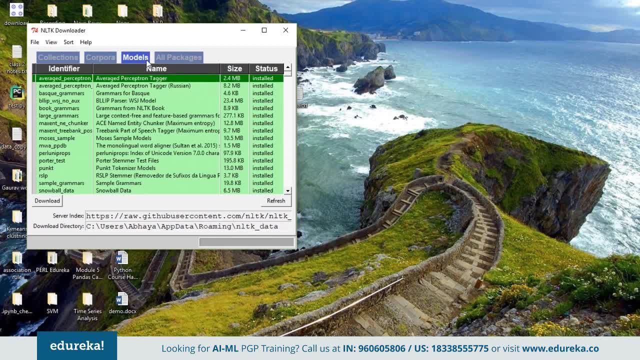 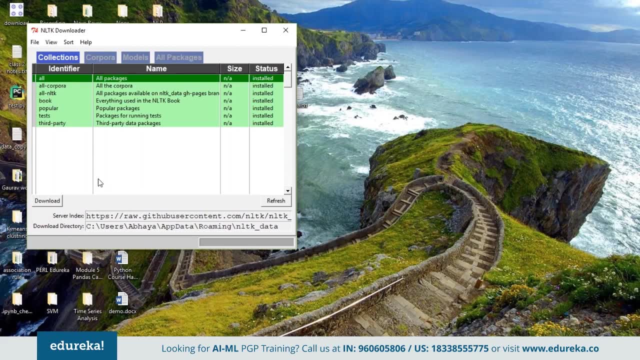 inbuilt models in NLTK, all packages within NLTK collection of packages, So you can download all of them. So simply, when you press download, it is going to download everything for you- Cobra models, packages- everything get downloaded for you. So that's the first step you need to do. 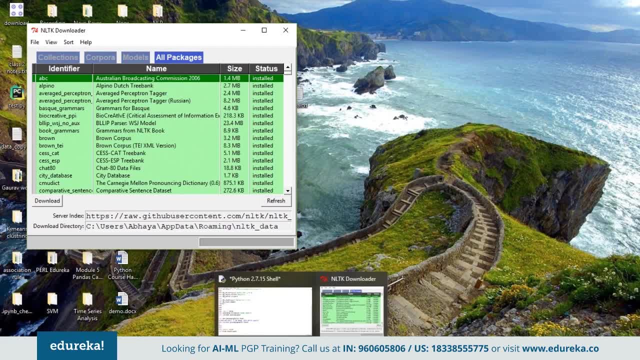 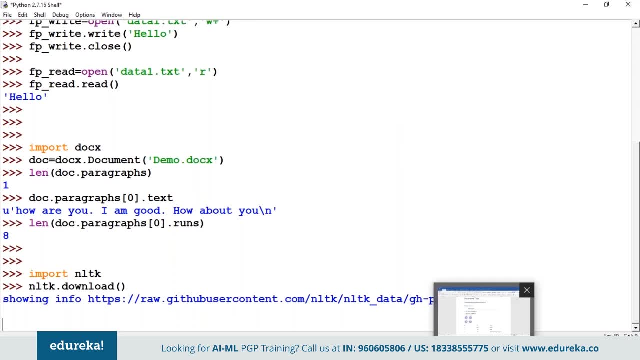 Once you install NLTK test, import NLTK, run NLTK dot download- It will download it. Now, what is there in this sub libraries? Let me show you. so this will take some time. It will take approximately half an hour for you to download everything in your machine. 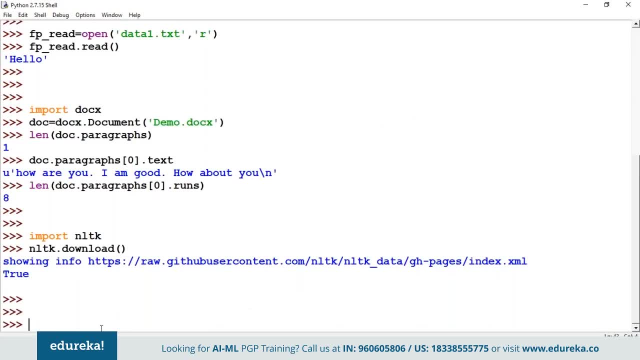 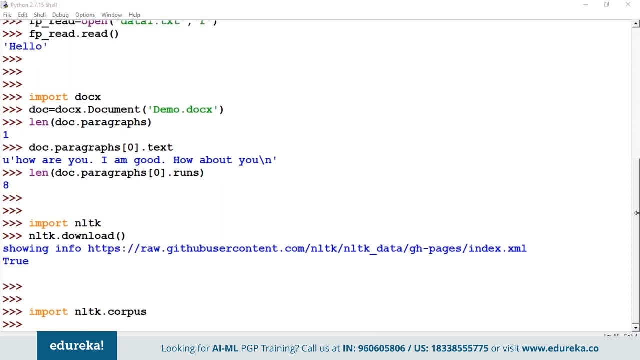 So once you download, all this library comes to you. So, if you can say, import NLTK dot corpus. this is again a sub library of NLTK. Now, this is the corpus is a very important library. It has got a lot of text into it. 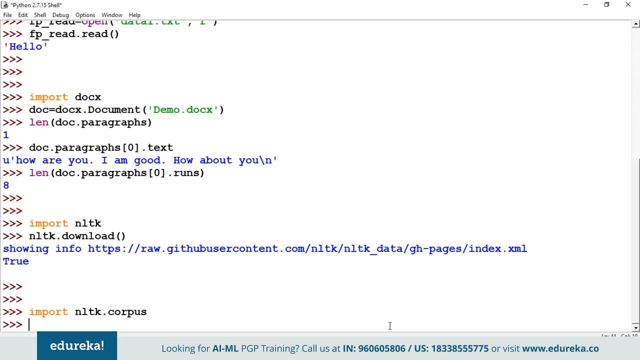 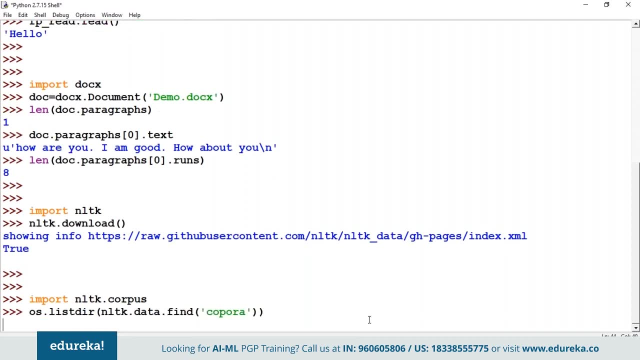 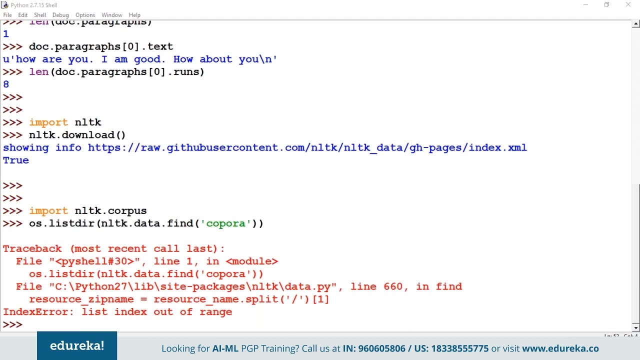 So once we install corpus, we can simply say: print or OS dot list directory NLTK, dot, data, dot. find this trend X out of range. So we need to. it's a very big list, It's coming out of range, So let me see there. 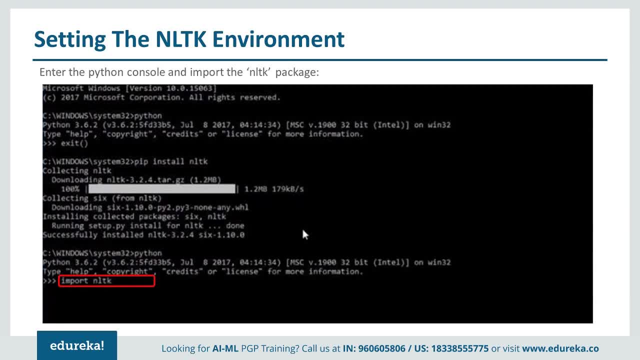 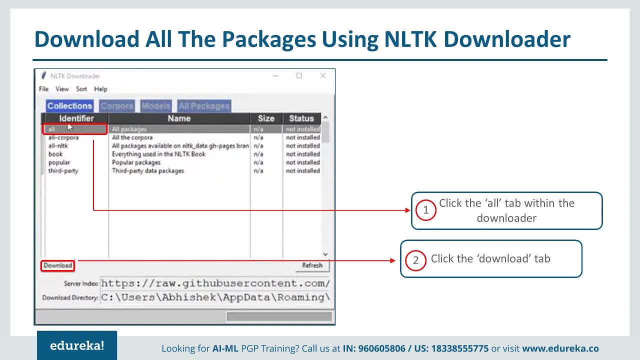 The first step is import NLTK. That's the first step. after downloading it, Second step is NLTK. It will download. it will download all the libraries which are there in the NLTK and you get a identify. click all tab within the downloader. 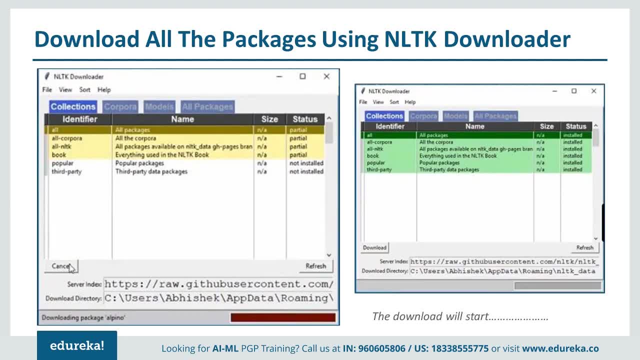 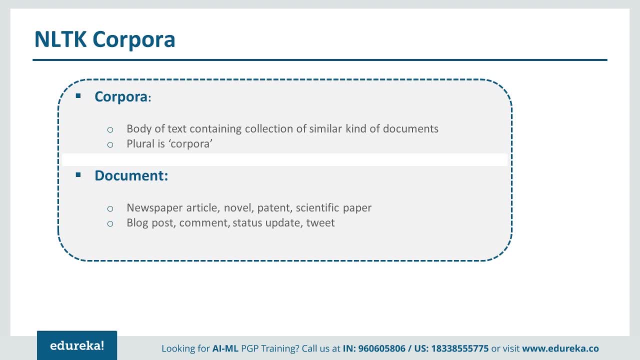 Click on all and click on download. It will download all the libraries for you. So this is going to, one by one, download all the libraries for you. now corpora is what corpora is: a body of text containing collection of similar kind of documents. 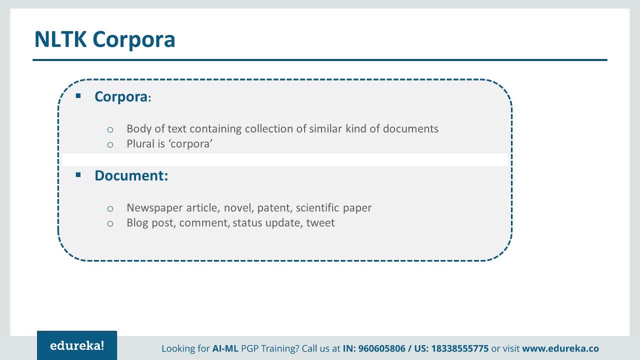 Plural is known as corpora. What is corporate library? corporate is a sub library of NLTK which is having collection of similar kind of documents. Let's say, see what is happening is how this NLTK works. I let me give you a brief. 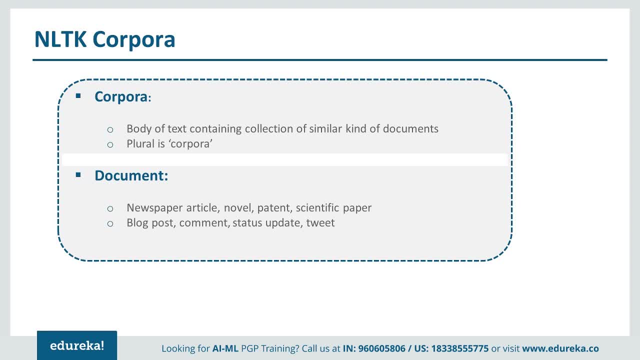 Idea. suppose you suppose, as a layman, you are learning English, right? What do you do when you start learning English? you come across with many words and you do what you use: dictionary, hard copy of a dictionary called Oxford dictionary. You search the word there, right? 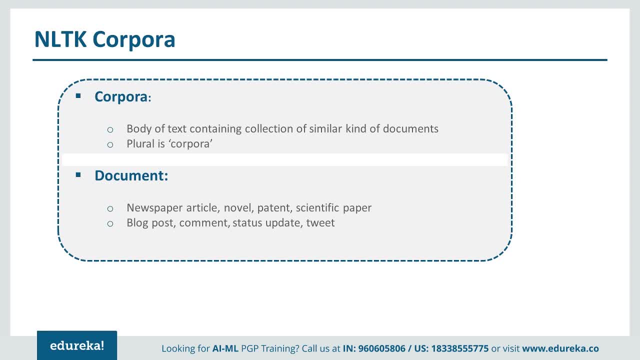 Suppose I say suspicious, you're going to search the word suspicious in the dictionary. see whether it's a objective, It's a noun, It's adverb, see its meaning, pronunciation. Everything is there, The dictionary. maybe in some dictionary examples also a sentence using that word. 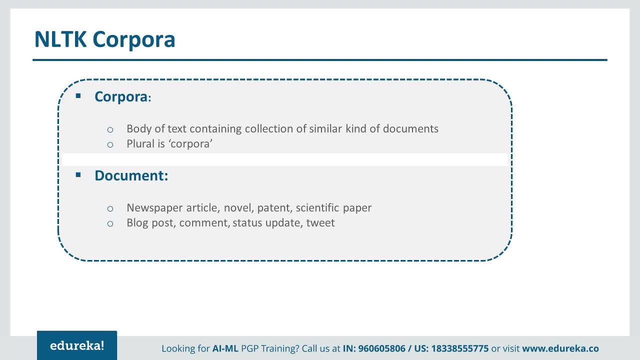 So copper is something like a same kind of a repository which is having in through throughout the world, Whatever the domains can exist: fields like science, like mathematics, like English or maybe within from the general life, maybe news, maybe army, maybe Air Force, maybe aircraft engineering, maybe biometrics. 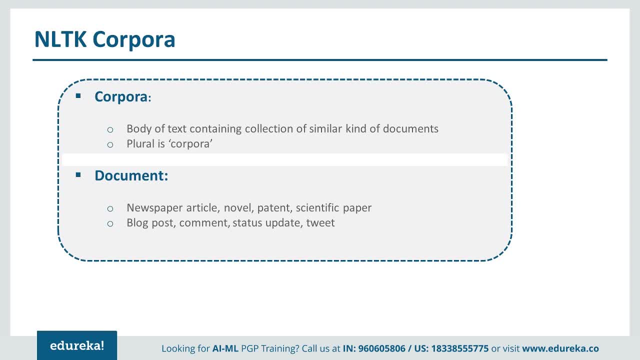 So it has divided the documents into these categories. and what is happening? Let's say, tomorrow you are going to give some data which is having some details of the airline Industries, So it is going to look at the Airlines document and look for the words. very similar to that. 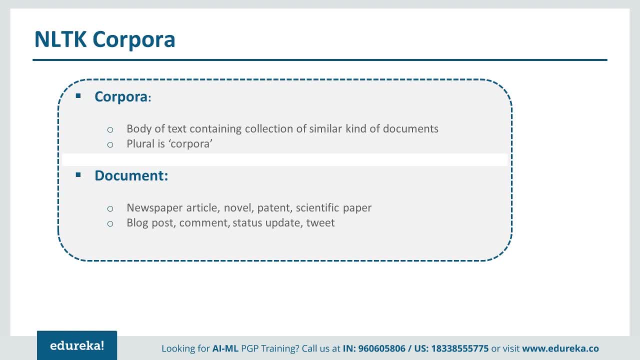 because every feel like the different words. if you go to an advocate, he use the different word terms of vocabulary. If you go to a doctor, he will be using different types of vocabulary, like benign tumor or malignant tumors or maybe some kind of a disease. 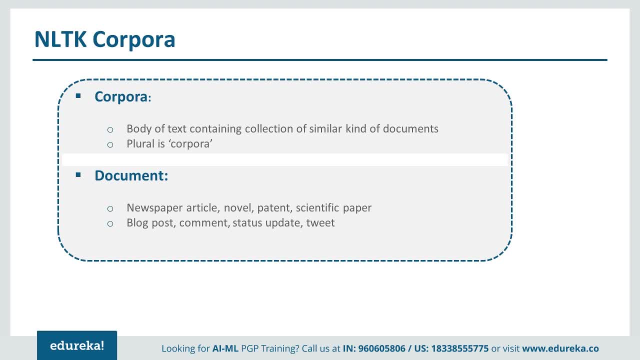 So every area has got its own words and this copper lab is doing what. it has got a files pertaining to this, pertaining to all the areas, and again, the documents can be a novel, patient, scientific paper, block comments, status update, tweets- any kind of a document is there in this library. 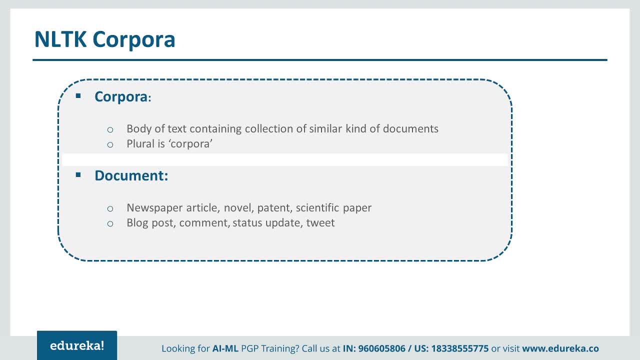 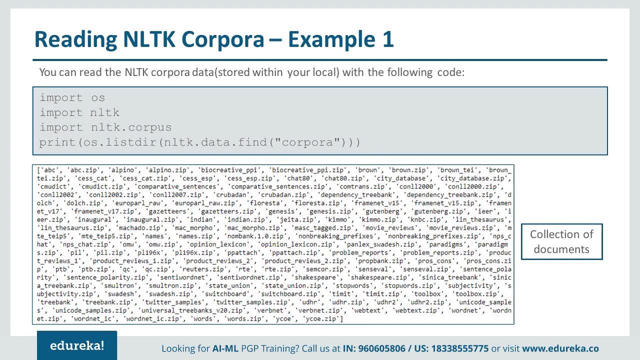 which is going to help you in filtering out What type of word you are looking for. So, reading the NLTK lab is who will say corpus, import NLTK dot corpus and say OS dot list here, DIR, NLTK dot, data dot, fine corpora. see this file. 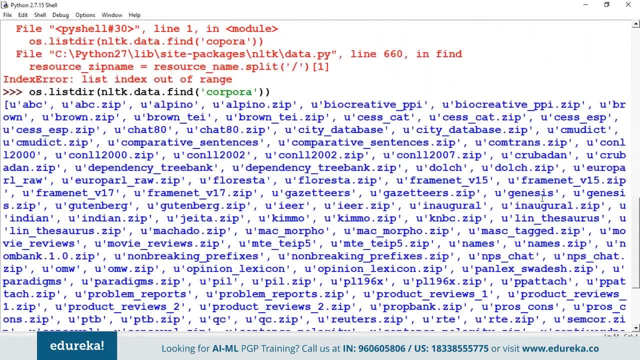 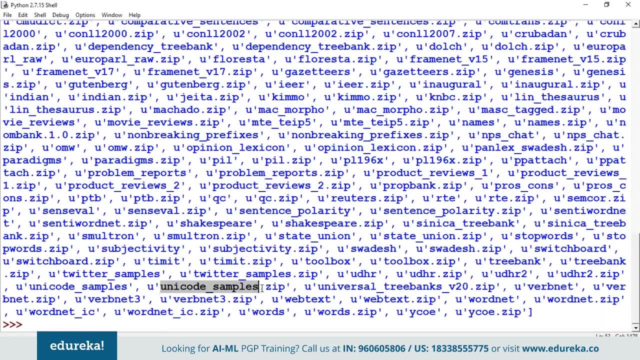 You have a something like zip files having all the suppose some sentence: popularity dot zip, maybe problem reports dot zip, maybe few other like Unicode samples dot zip. Twitter samples dot zip. So this zip files again have a hundreds of folders there within them and each folder is having 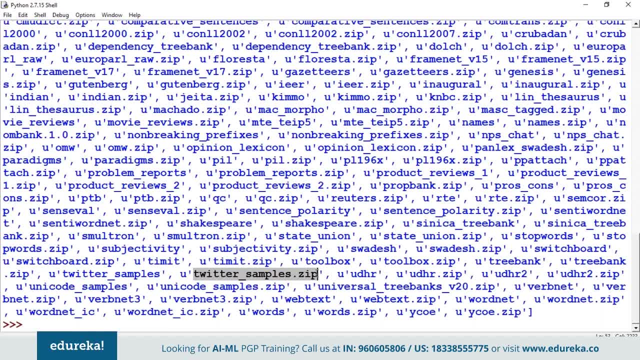 Different, different categories. suppose you want to filter out some Twitter data and do sentiment analysis and somebody said something in a document that is going to search within this library: What is the meaning of the particular world. So this type is like a metadata which is going to map. 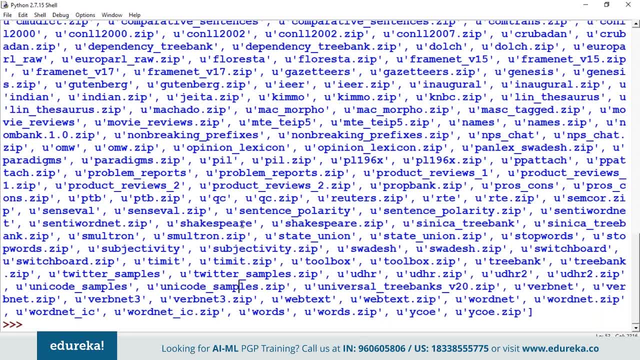 up with your document. Whatever you are having it is going to find the exact match and find out the relationship between them, like how it can be used for this, in making these like a metadata. for that you'll have a business like a dictionary- Oxford dictionary for us, and suppose you are learning English- what we see, we regularly see. 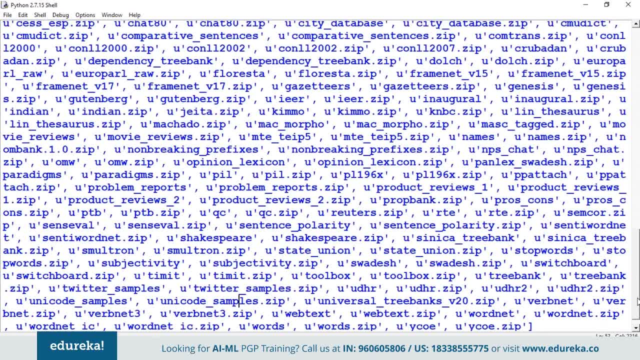 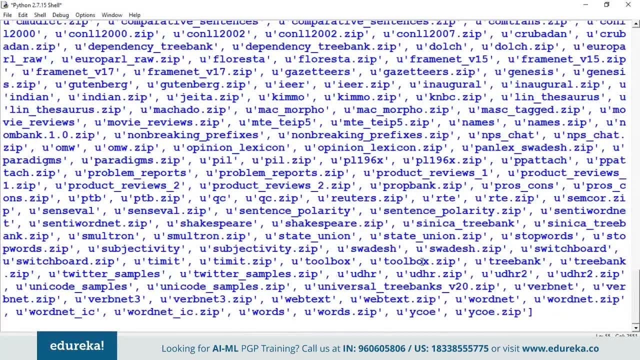 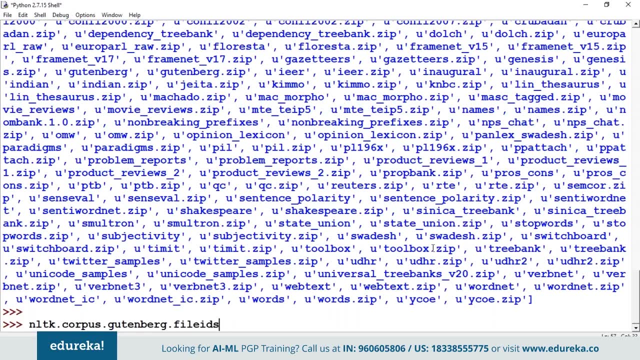 The dictionary find the meaning for synonyms, for antonyms. This is going to help it like this. This library is like a dictionary, So we've got suppose I say NLTK, dot corpora or corpus, The plural is corpora called. There is one library in this called Gutenberg dot file IDs. 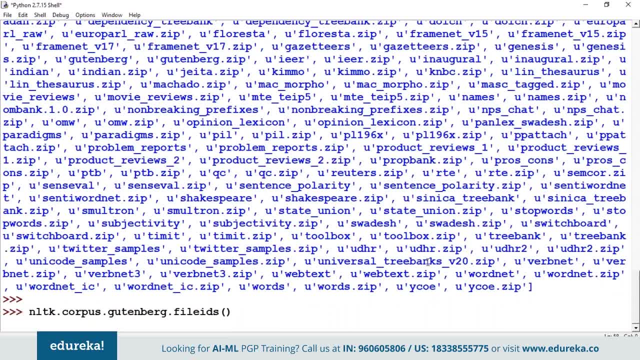 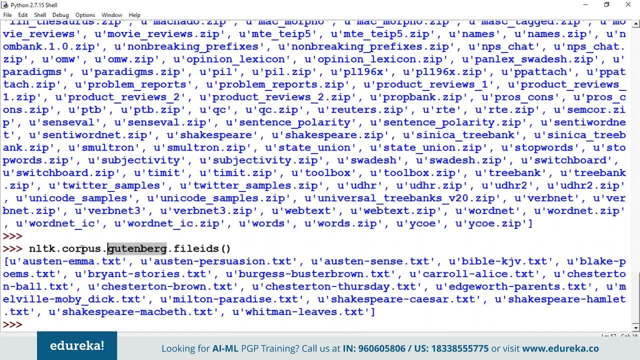 So what we want to see, if there's something, what is there in the particular sub library? Gutenberg, file IDs is going to tell you the name of the files present in the same. So this Gutenberg is one of the sub library in this corpus, on which or Gutenberg is a kind of a zip file. 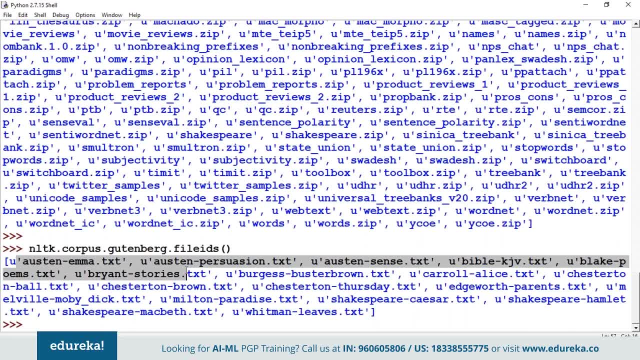 You can say in this, which is having all this text files present in this, so it can have hundreds of sub libraries and we have a text file. having some metadata into it means like definition of some car or maybe some word which you are interested in. It's something like a dictionary, Oxford dictionary. 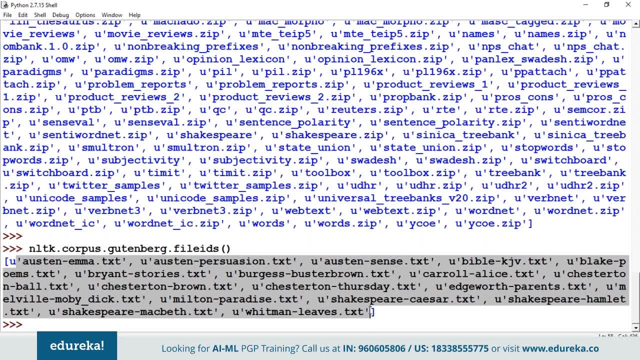 which is having all the details there in it. You can use it for a decision-making purposes, Suppose. I want to see the text within this and see that said: create a variable X equal to NLTK, dot, corpus, dot, Gutenberg file IDs. I want to filter out the words from Shakespeare. Shakespeare. 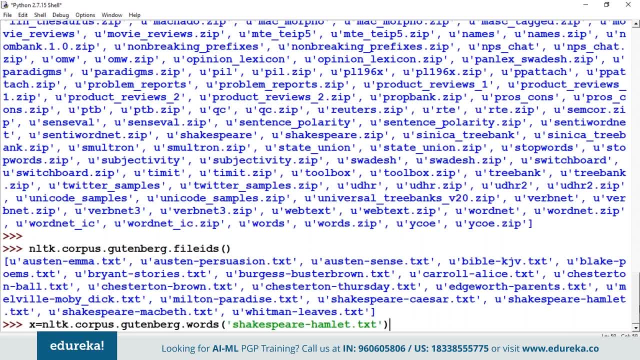 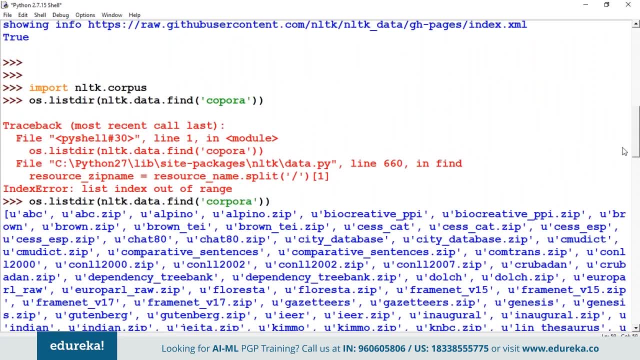 Hamlet. So we are going one level down. So first of all we did what we use: the corpus library all together in the bigger format. then we find within corpora. We have been filtering out all the files and folders present in corpora. 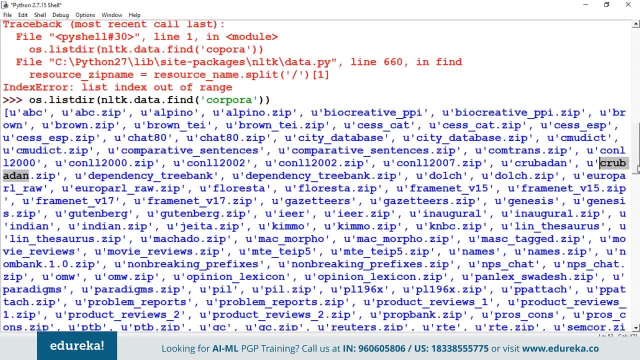 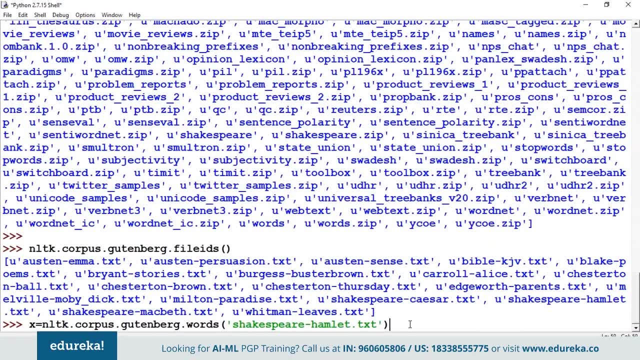 Then we filter out the file and folder and go to the level of the file present in the particular zip files. Then we are picking up a particular text file within this and going to store it in X. I can run a for loop forward in Hamlet. 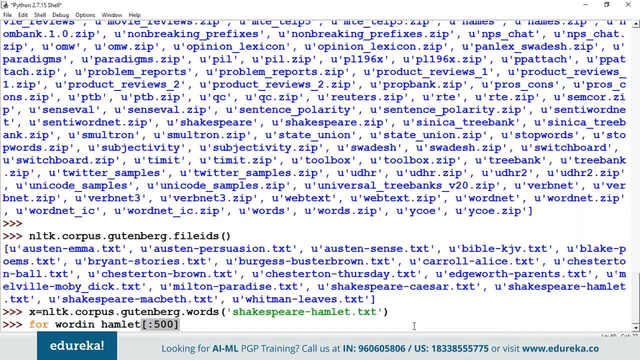 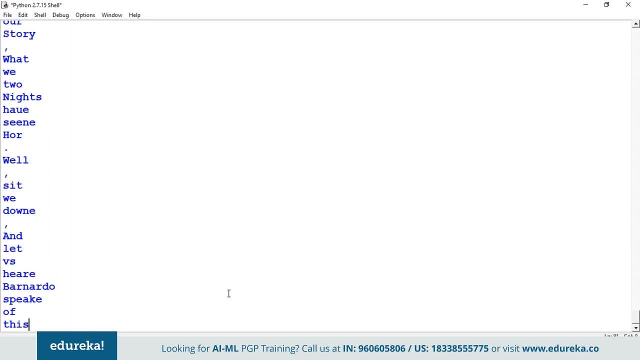 and I want to filter only. I wanted values forward in who. I've decided to text my mistake. Let me put it as Hamlet. You can see the text file is having so many words there in it, like a dictionary and information about the same. 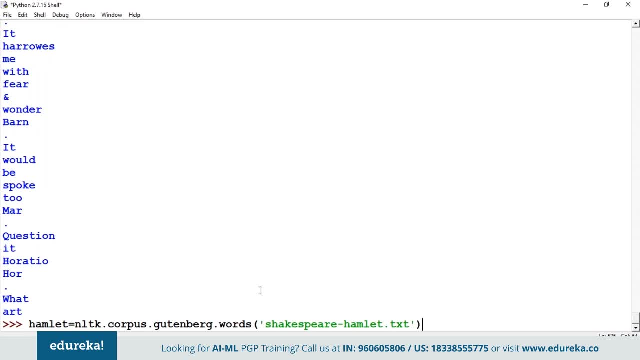 First of all, we go to the Gutenberg sub library. within that we pick up the words from the file Hamlet dot txt and after picking up we are printing all the words present over there in that particular text file. This is a metadata having all the data. 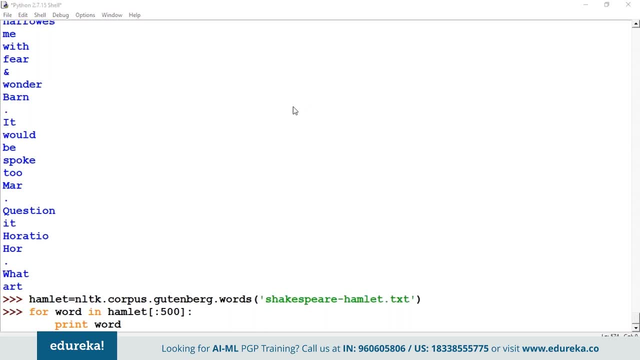 What are the words which are possible? Similarly, we have other sub libraries. Also There's one library called movie reviews. So we can say from NL, TK, dot, corpus, import movie reviews. If I want to see the movie reviews category say movie reviews. 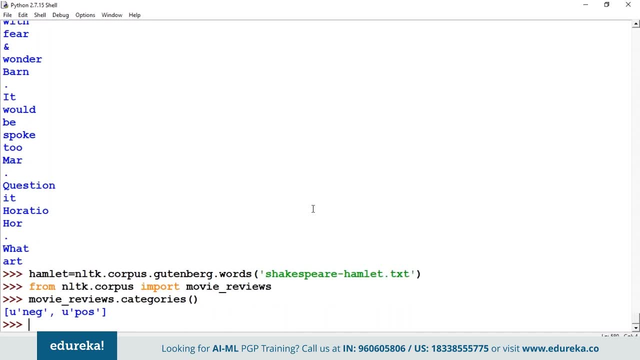 So we have a positive and negative keywords And if you want to see what is there in the positive keywords will simply say movie reviews, dot file IDs and again it has some text files. So, as I told you, we have a library within that library. 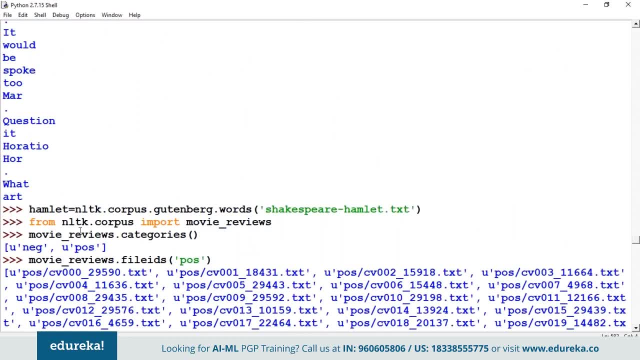 We have some libraries. It can have a zip files, It can have a text file. So what I did here? I have imported movie reviews. So movie reviews has got something called file IDs. file It is is basically like a dir. it is giving the contents. 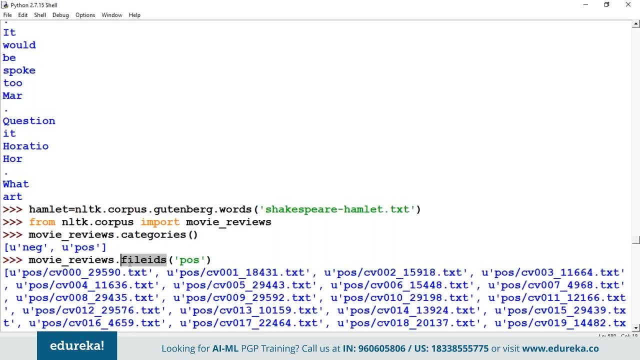 of the particular zip file or maybe sub library. So file ID is something like function on the particular object which is filtering out all the contents in it. So I want to see positive. I figure it out, POS, and it will give me the positive feeds. all the positive now. 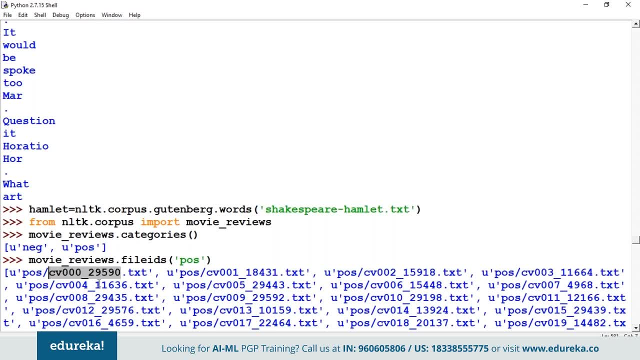 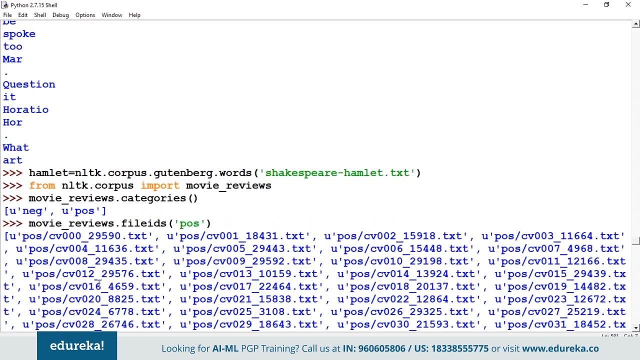 you can pick any of one of them and print the details of the same. What is there in the text file. I can pick any of them and print. what is there in this text file is something like I'm browsing a dictionary, randomly picking Any of the dictionaries. 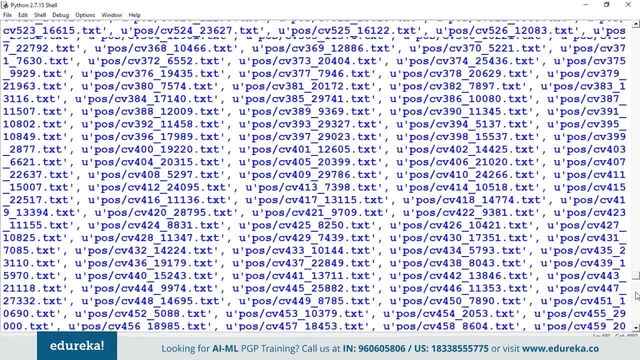 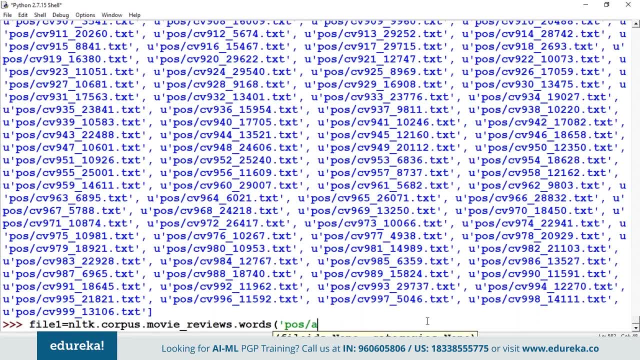 So if I write file 1 equal to NL TK, dot, corpus, dot movie reviews, dot words, and I want to access POS, a triple 0 underscore 2, 9, any number which is there is a part of this might, is giving arrow no such file. 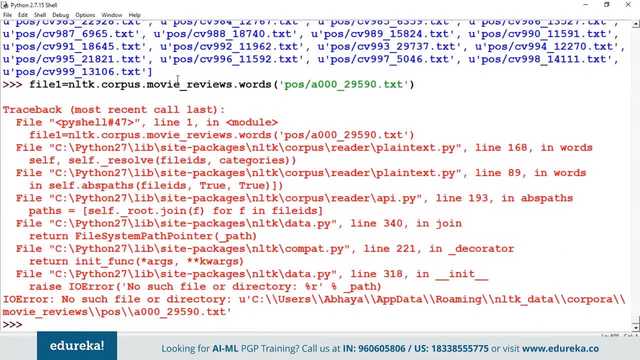 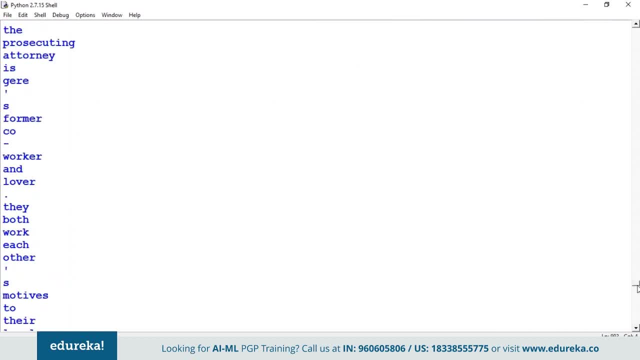 So we don't have a file this. let me take here this one. So these are the words present in them. So many words defies on them, So it's something like in real time. So daily we read newspaper. Imagine you have a year newspaper of, let's say, last 20 years. 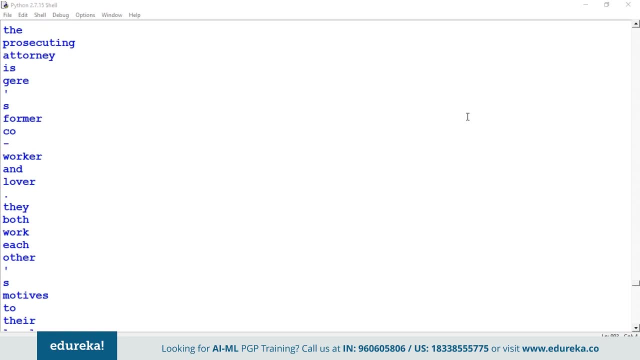 for the daily basis and you feed this all newspaper in the form of a dictionary with some meaning in there in the relevant files. If it is science related document, put it in the science. If is a chemistry related, put it in a chemistry. medical related, put it in medical. 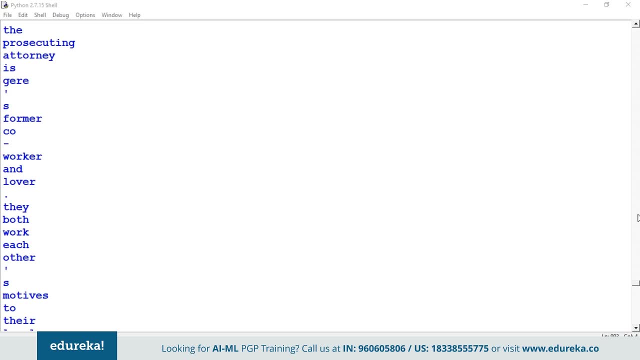 So this libraries, analytical libraries, have all the metadata, meanings or antennas, or synonyms or the mapping of these words internally. It has done any doubts up till here. guys, anything want to ask? Let's try accessing document from the copra. So these are the so many documents in Gutenberg. 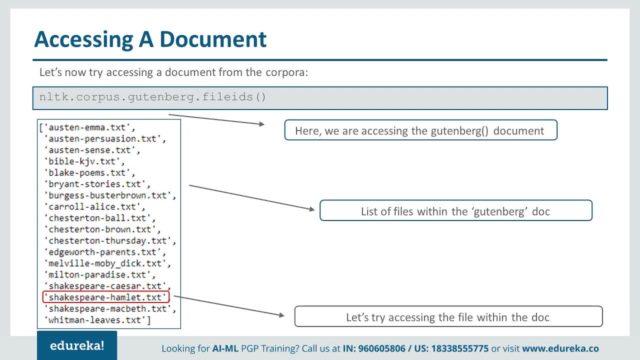 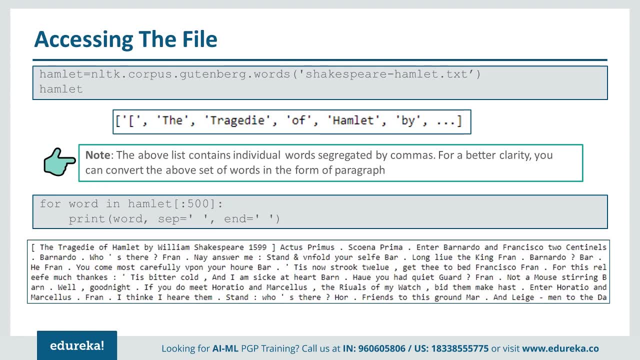 So so many documents pertaining to Gutenberg library. Similarly, Hamlet, Gutenberg dot words. Shakespeare, Hamlet dot txt. So you'll see some text from the file the tragedy of Hamlet by. so. the above list command contains individual words aggregated by commas for a better clarity. 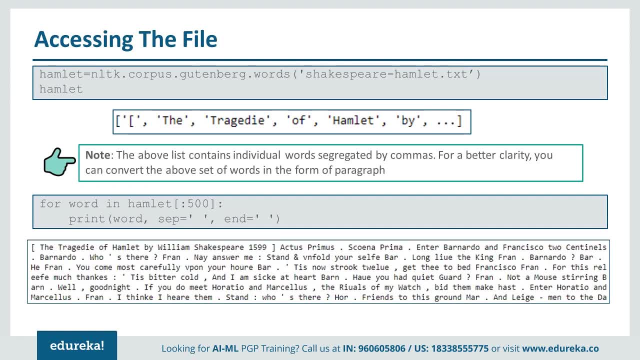 You can convert the set of words in the form of a paragraph, So you can put all the words in a form of form of paragraph, print word, each by line, by line, So you can see it's like some simple English newsletter kind of a thing, like a newspaper, like a novel. 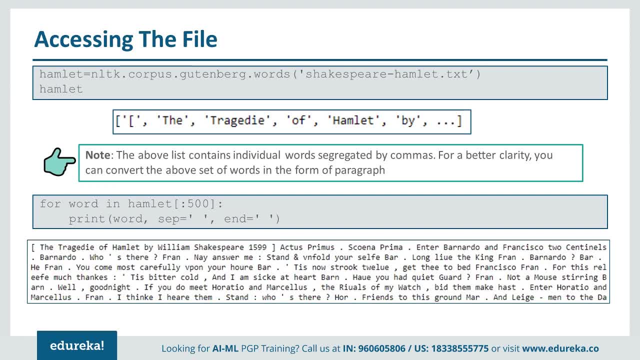 or a magazine. the tragedy of Hamlet by William Shakespeare, 1915, 99.. So you can see simple file which is having the text written in it, and this text are written such a way that we are going to search in future You'll get the context out of it. 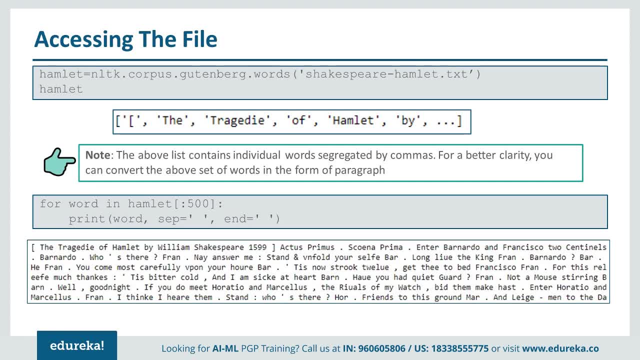 So why we are reading this kind of a text? because we want to know the context. like, for example, if I say what dog system should understand, the word dog is first of all a noun. Secondly, if it is a noun, in which context we are using. so we come to know a quick way. 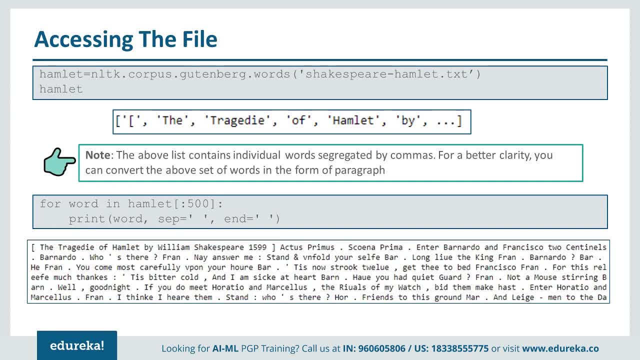 We will look at a tree inside. So inside the system, tree is going to getting created like noun is their word dog. dog is used in context of barking, dog is in context of pet, dog in context of security, dog in context of animal. Then again, we brought up tree like structure. 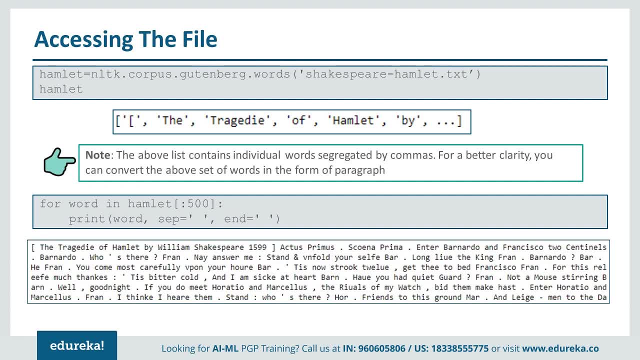 like a random Forest, big tree, Like what is? the word dog has an inference and in our sentence in which context we are using. so it is mapping that. that is, finding it internally mapping the word dog has what context we are using it. are we using in context of being a pet? are we using in context? 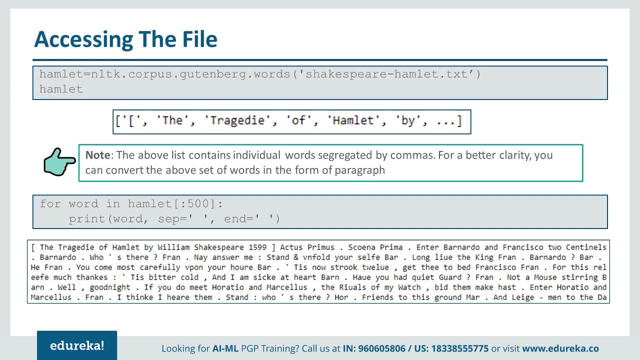 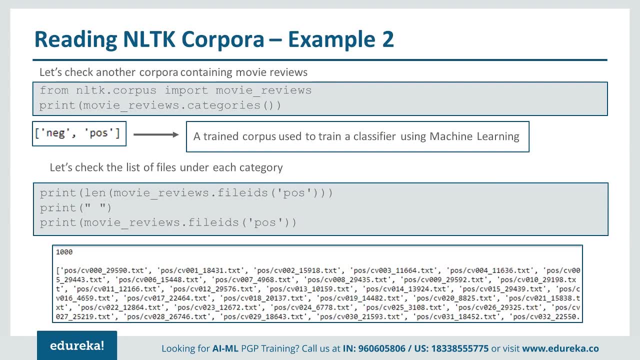 of barking are we using in context for playing? that's the purpose of this natural language: to figure it out in what context you are using this world. similarly for movie reviews. another: we have a category strain corpus. use a train to classify using machine learning. So we can have positive, we can have a negative reviews files. 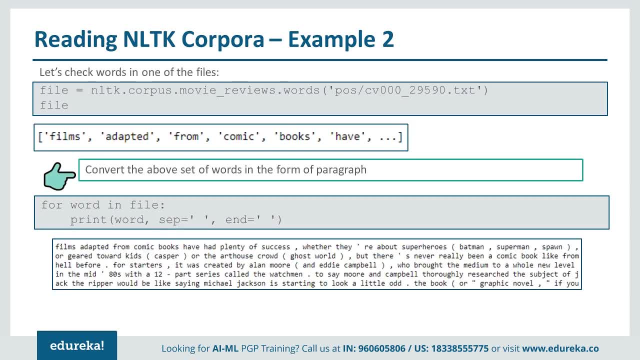 Similarly, you can see the file within words. You can see the file details of the files. you can print it in a form of a paragraph. fills are adapted from comic books and have plenty of success about superheroes. So you can see here There's some of the files are separated by single code. 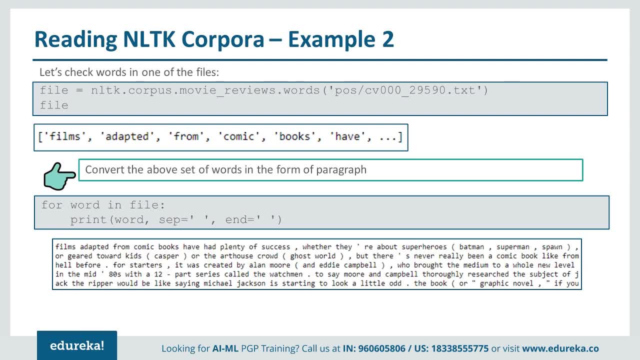 Some are separated by question marks, So it depends like how the file has been made. There's a separator always. some of the files are separated by question marks, some with a single code, some with a star, some with a double quotes, So it depends like how the programmer has made this.